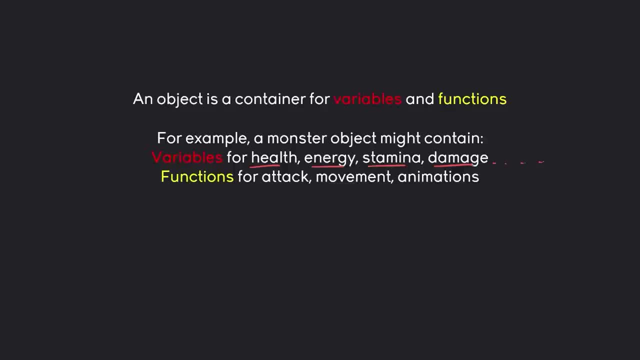 whatever else you want in here. it's really up to you. And then, besides that, the monster should also be able to attack. And then, of course, we want to have some health, some energy, stamina and damage, And you could add whatever else you want in here. it's really up to you, And again. 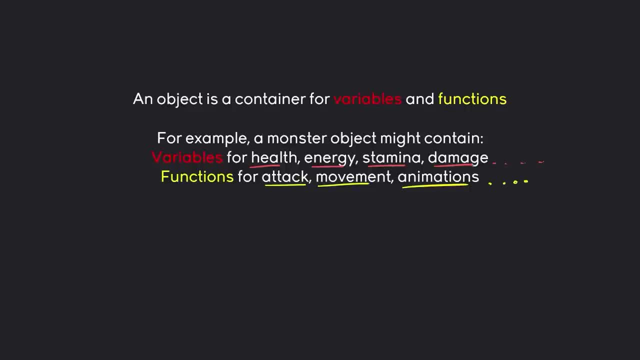 you could add whatever else you want in here, And what you have to understand here is that these variables and functions only exist inside of this monster object. It's very similar compared to the local scope of a function If we tried to get this health outside of the container. 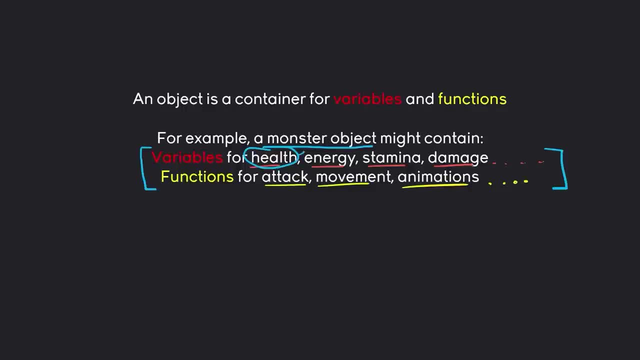 it wouldn't exist, because this health exists only inside of a monster object, Although in terms of naming, you could add whatever else you want in here. And what you have to understand here is that there's one minor complication, and that is special names. All that really means is that 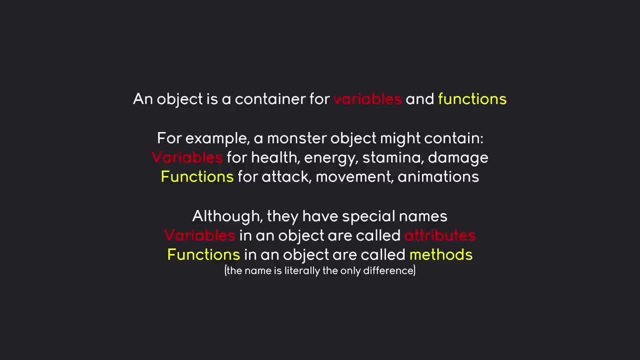 variables inside of an object are called attributes and functions in an object are called methods, And that is more or less the only difference. The only reason why this exists is so that we are a bit more specific with our language, For example, when you talk about health with 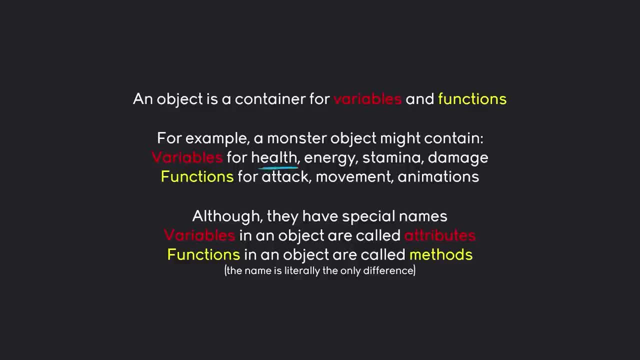 somebody else for your game. you really want to emphasize that you don't talk about a global variable, You talk about the specific attribute of one object. And one more thing: methods should actually be familiar to you, because you are using methods very, very often in Python anyway. 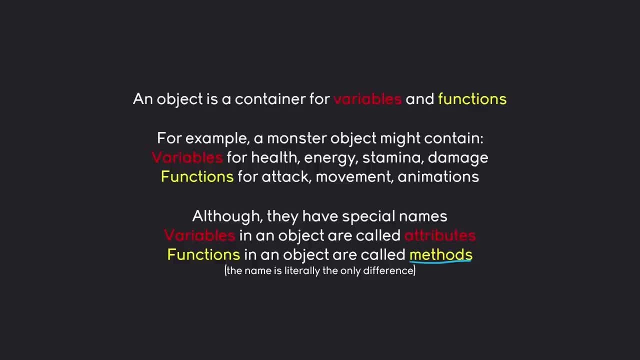 For example, when you call the upper method on any kind of string, you are turning every letter inside of that string to an uppercase letter, And that is also a method. And that is the same kind of method we are seeing here, Essentially a string in Python. 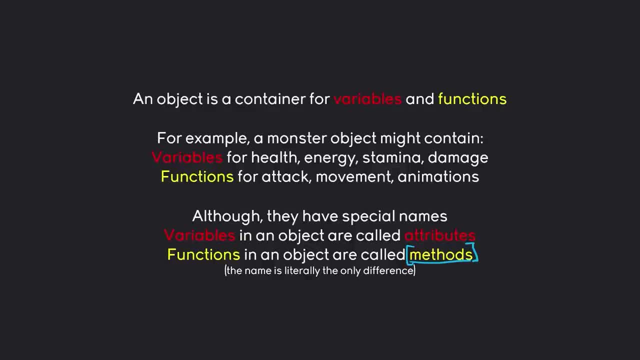 is just another object with functions inside of it or methods. to be more specific, This also applies to integers, floating point numbers, booleans. all of that stuff is basically just other kinds of objects that Python creates, But that's something we don't have to worry about for. 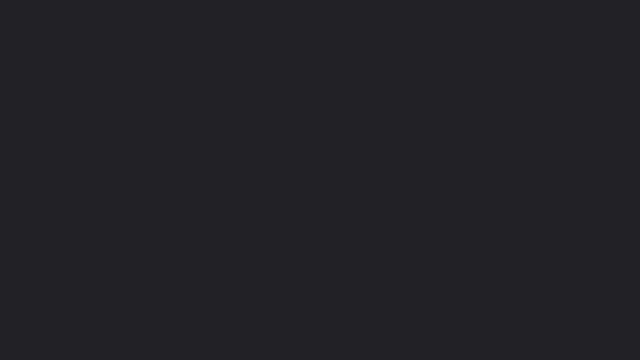 now. Now, another thing that is really important to understand is that it is possible to have multiple objects. For example, I could create three different monsters, And each of these monsters could have customized attributes, These red pieces of text here. So my first monster has 90 health. 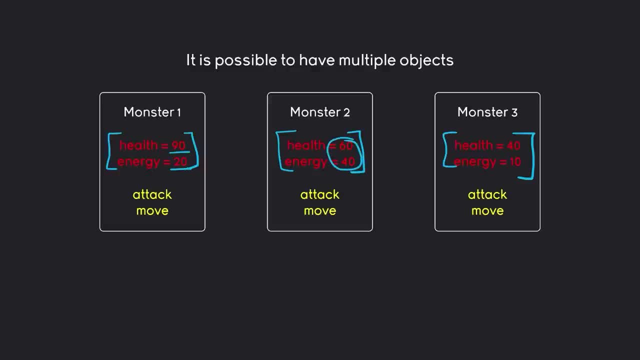 20 energy, the next monster has 60 and 40. And the final monster has 40 and 10.. So when you create an object, you can give it custom attributes. However, this does not apply to methods And, as you can see here, monster one, monster two and monster three. 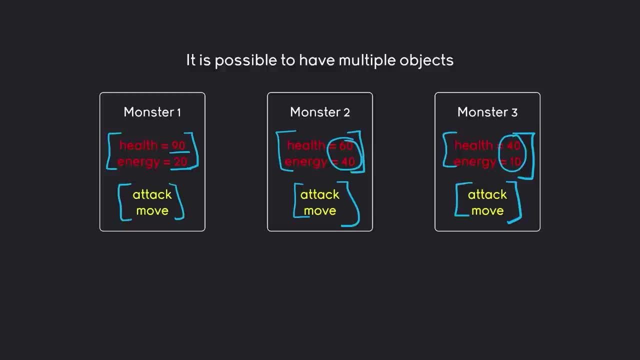 all have the same methods And these can be customized to an extent, but not nearly as much as the attributes. That's something you do want to keep in mind, But still, each object has its own attributes and methods, Meaning that this attack here and this attack are not the same. 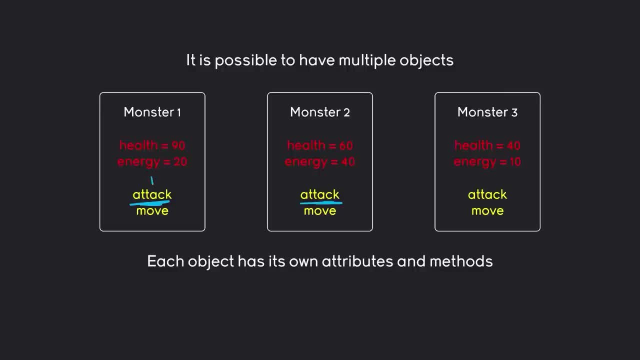 function or well, the same method. They always apply to their respective object, And what you can also do is that you can create an object that has the same attributes and methods, And this is something you can do is have objects interact with each other. For example, if monster. 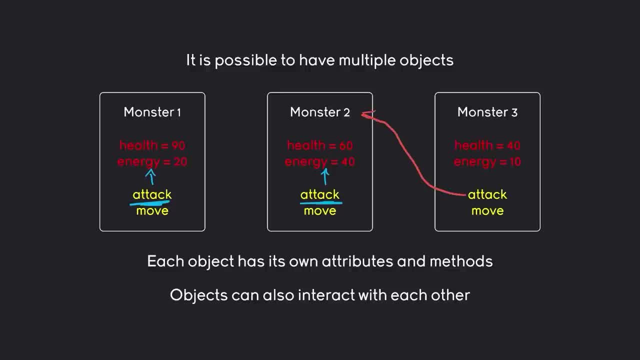 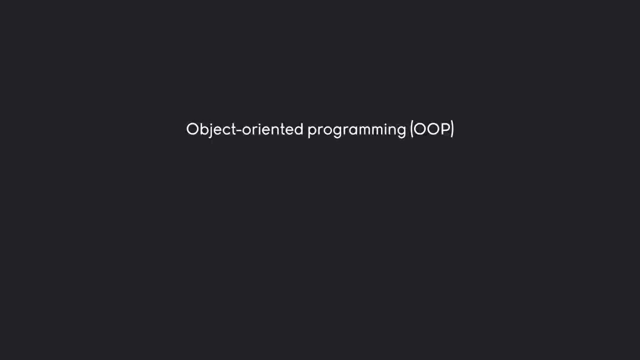 three attacks monster two. we could run some code to reduce the health of monster two from 60 to, let's say, 20.. And that actually brings us to a really important topic, And that is Object Oriented Programming, or OOP in short, And all that really means is that you're organizing your code via 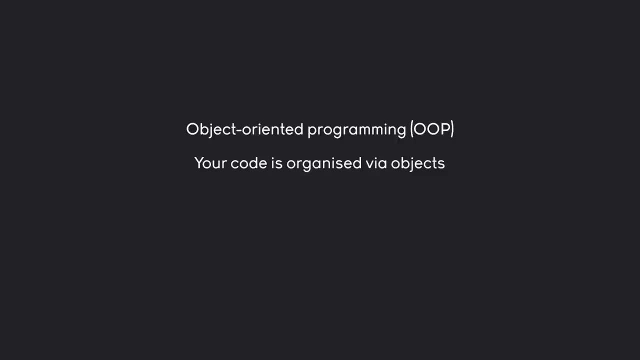 different objects, And that means that you're organizing your code via different objects And then you make these objects interact with each other, And this approach is basically how almost all large projects are made in any programming language, or, at the very least, any modern programming language. Meaning: if you don't understand classes, you will be very much. 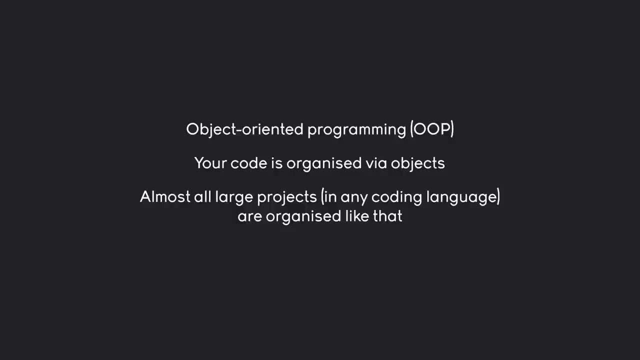 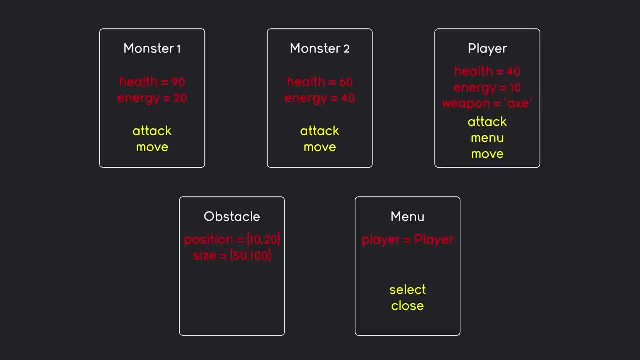 lost. And well, you will have no idea what you see when you look at larger examples of code. Here we have a couple more objects. We still have monster one and monster two, But now we also have an obstacle and we have a menu, And all of these have slightly different attributes and slightly 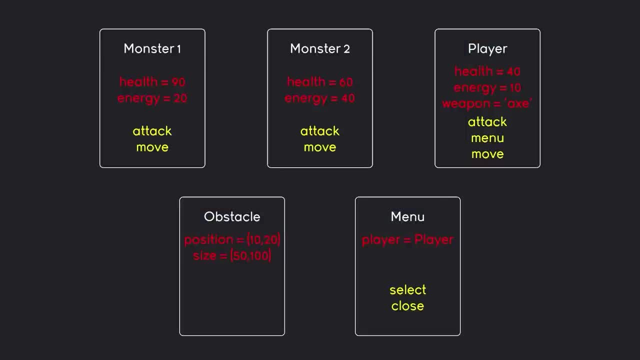 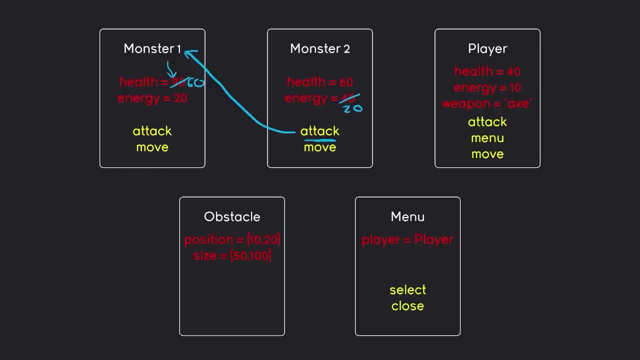 monster two is attacking. it might reduce its own energy from 40 to 60. So attacking isn't free for the monster. What we can also do is have an object without any methods, like the obstacle here- And all the obstacle is- is well, an object with a position and a size, And this we could use. 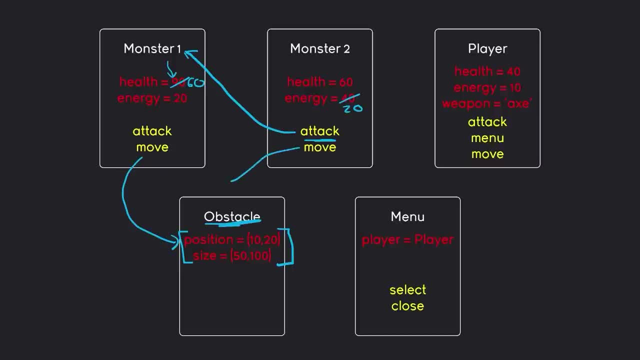 for example, with the move method of any of the other classes. So the player and the monsters all have a move method And this could interact with the obstacle. And let me clean this up, Something even more interesting If you look at the player, 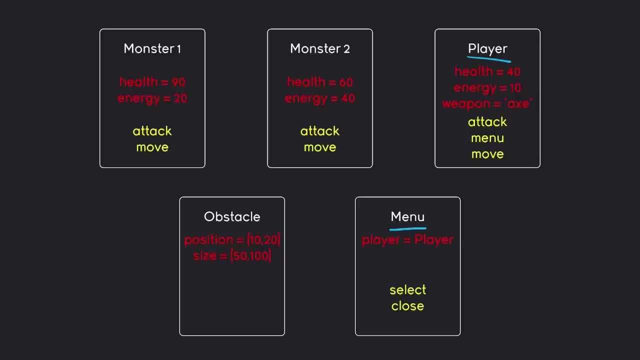 this one here and the menu. those two do look very much connected because the player has one method called menu And what this one would do is to create, or at the very least open a menu And then, when we create the menu, we are passing in the player itself. So this player, 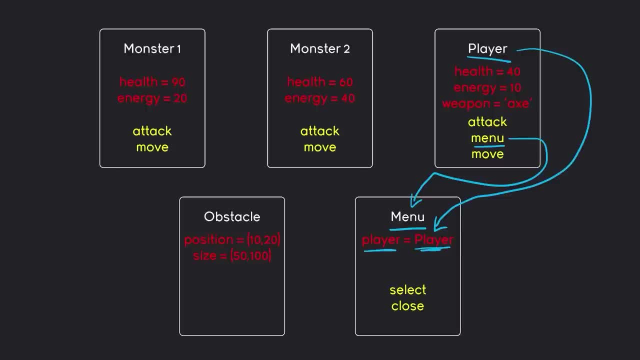 here is going to be passed in as one attribute of the menu object, And this is totally fine to do. You can totally add a function or an object inside of another object as an attribute, And then this select would, for example, change the weapon of the player And we could close the. 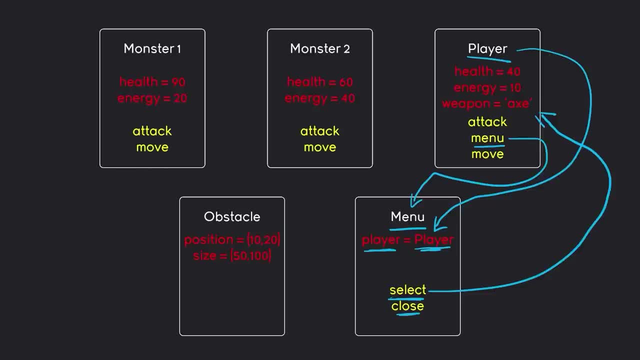 menu as well, And I hope this makes sense. The main thing you have to understand is that objects can interact with each other, And that's what we're going to do here, And then we're going to close the menu, And this is how you want to organize code. It makes it very easy to work. 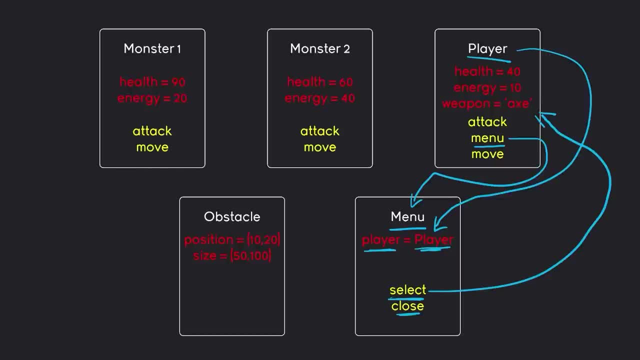 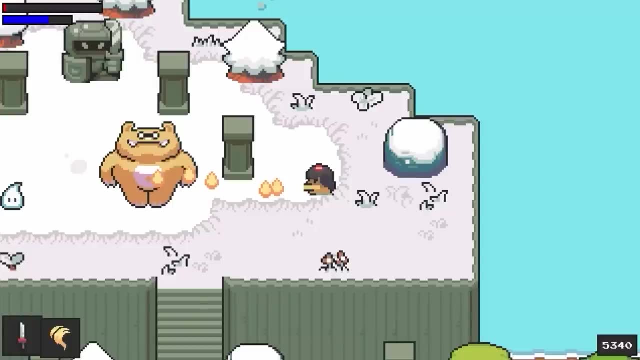 with, And especially for, larger bits of code. this approach is essentially mandatory, Or at the very least, it's the easiest way to organize it, And let's actually do. a practical example. Here is a Zelda-like game that I made a while ago, And basically everything you see on the screen. 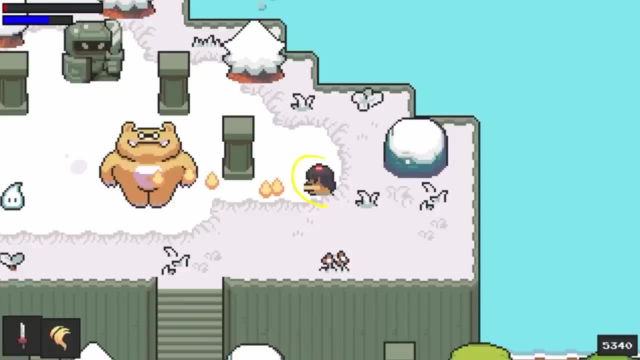 is an object. For example, right in the middle we have the player, and that's one object. Then we also have this raccoon here and the spirit, And each of those are one object, And beyond that, each of these flames here is its own object, And these are. 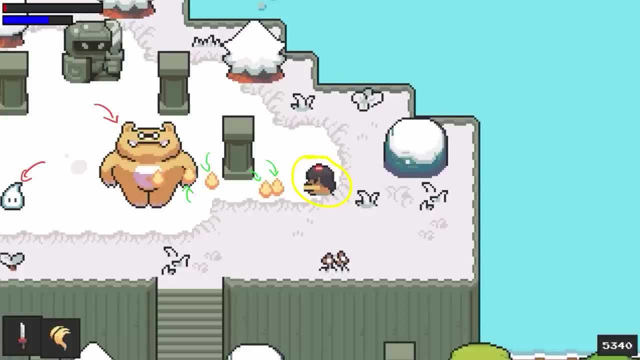 only created when the player is attacking with some magic. And finally, in the top left, the bottom left and the bottom right, you can see some UI elements And they are all part of the same object And this object is very much related to the player. So those two 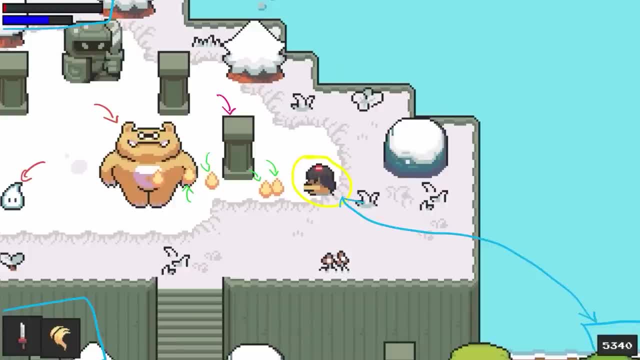 work together very closely. And besides that, each of these pillars and trees and rocks and statues- they are all objects that I created just for this game, So I hope that illustrates how useful objects are. They make it really easy to group together code chunks that should belong together. 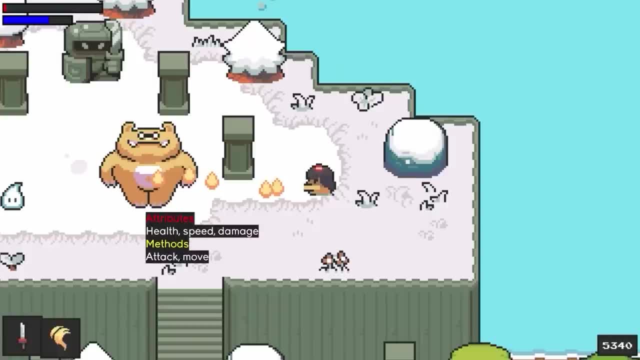 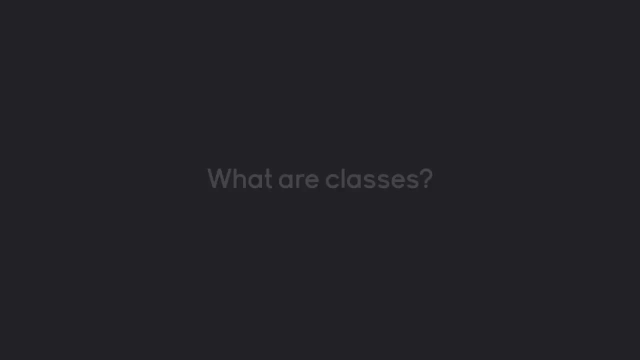 For a bit more detail. the raccoon, for example, has three attributes: health, speed and damage, and the methods, attack and move. And all the other objects would have similar attributes and methods, And with that we have objects. Now the next question is: what are classes? And this is: 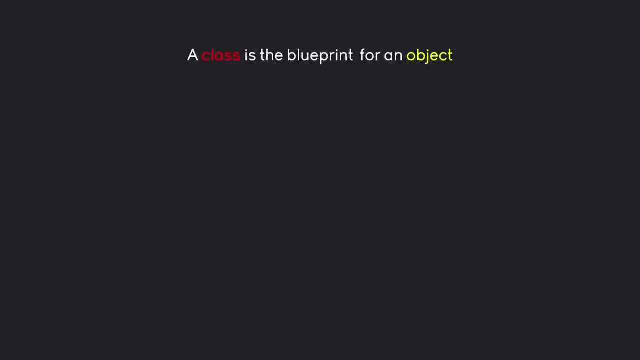 fairly easy to explain as well. The class is basically a blueprint for an object, meaning, whenever we create an object, we first have to create a class, And a class can also accept arguments to customize the object we are creating. For example, this would be a class, we have a class and this class has two attributes: health. 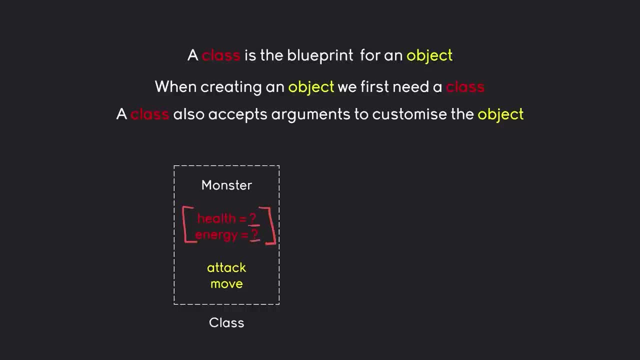 and energy, And right now the value for both of these is not being set. This we do when we actually use this class to create an object. But this class also has two methods- attack and move- And those do not change. And basically what we're doing is use this class to create the object And in the process, 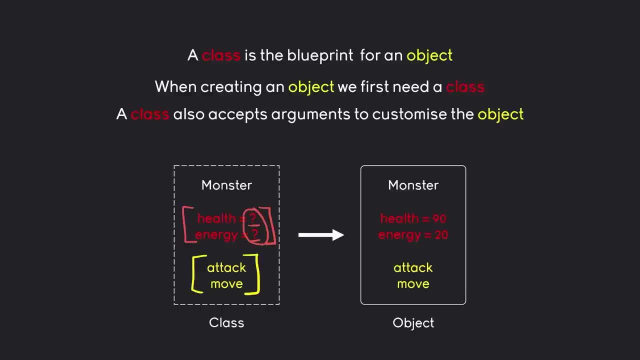 we are giving it the specific values for health and energy. So in this case the monster is going to have 90 health and 20 energy, And this process we could do as many times as we want. For example, earlier you have seen monster one, we had monster two. 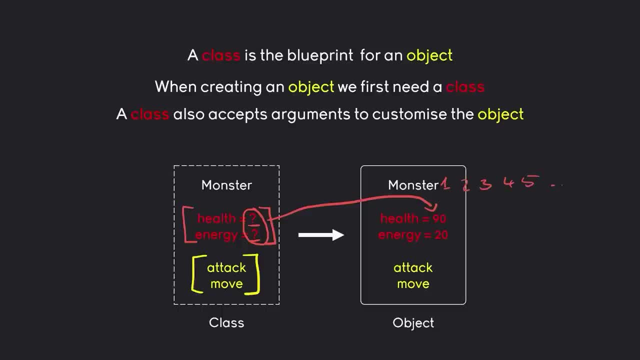 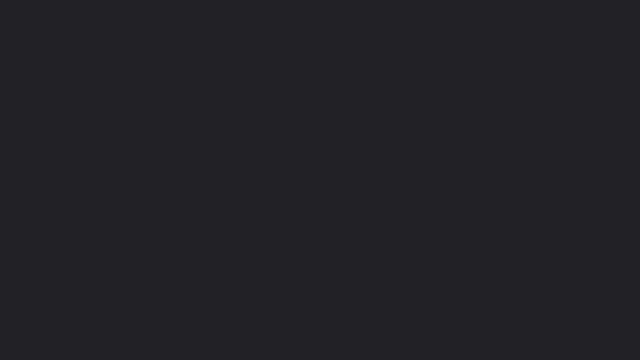 monster three, and we could continue with monster four or five up to an unlimited number, And that is essentially the main idea. All you really have to understand is that we always need a class to create an object. Now, what we can also do with classes is that one class can inherit. 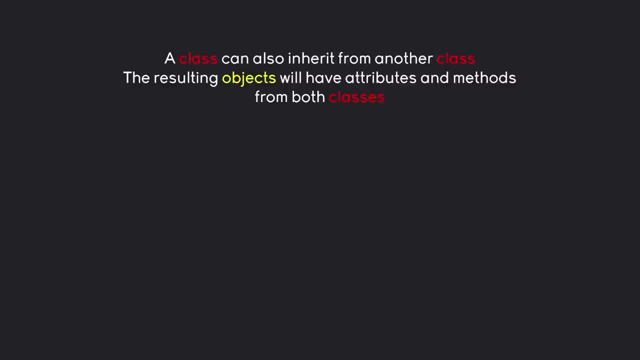 from another class And the resulting objects will have attributes and methods from both classes. For example, let's say we want to create a shark class And this one right now only has speed for the attribute and bytes For the method, And this class will be fairly limited because we well don't have any attribute. 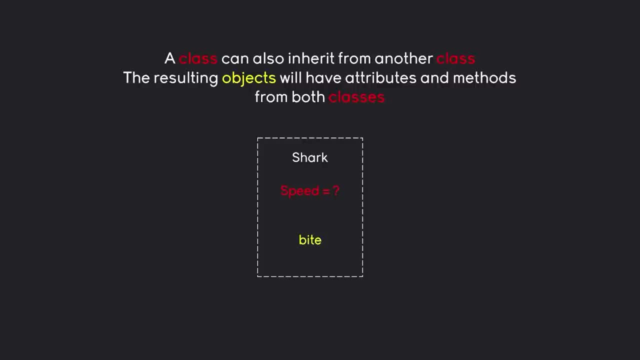 for health or for energy, And we also don't have any kind of method for move or attack. But we don't need to, because what we can do is have this shark class inherit from the monster class, And this means this shark is going to get the health and the energy from the monster parent. 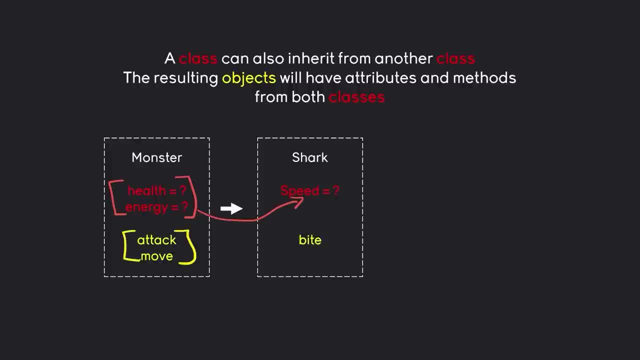 class And that is also going to get the attack and the move from this class as well, Meaning, when we actually use the shark class to create a shark object, we are going to get health, energy and speed for the attributes and attack, move and bite for the methods, And I think I should use better colors here. 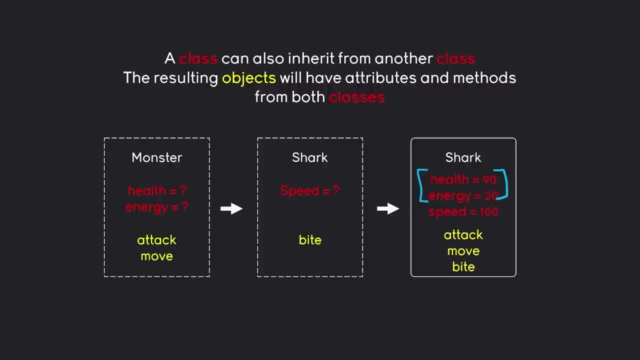 In the shark class. health and energy are coming from the monster class, Same with attack and move. Those two are coming from the monster class, And then speed and bite are from the shark class, And this would allow us to reuse code quite extensively, For example. 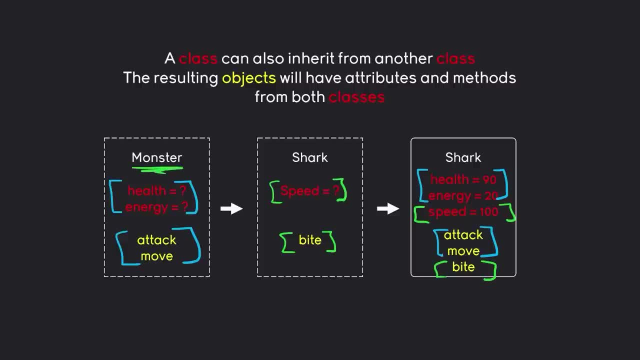 we could have a lot of different monsters. We could have a shark, some flying enemies, some armored enemies, lots more- And they all have different effects. So we can see that the shark class is going to inherit from this one monster class And with this approach, we would save a ton of writing in terms of code. And on top of that, 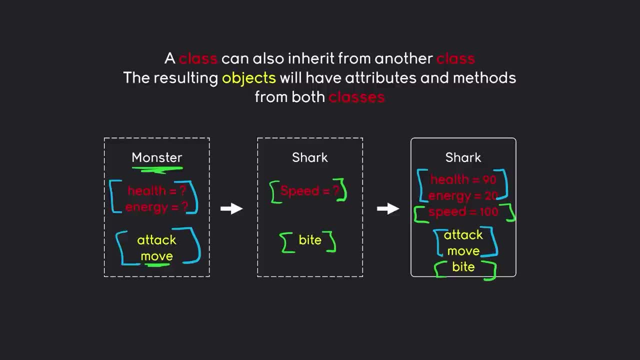 if we change the move method, for example, it would affect every single other class as well, which is very useful if you want to make some changes and make it affect every single other class, And especially with larger projects, this is just about the only way to manage them. 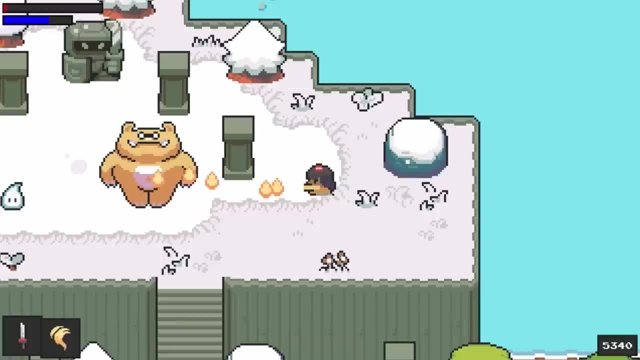 So let's do an example again. Here is the screenshot from earlier. And we have a monster class, We have another monster class, And those two have the same attributes and methods, although with different values, And besides that, we also have the player. 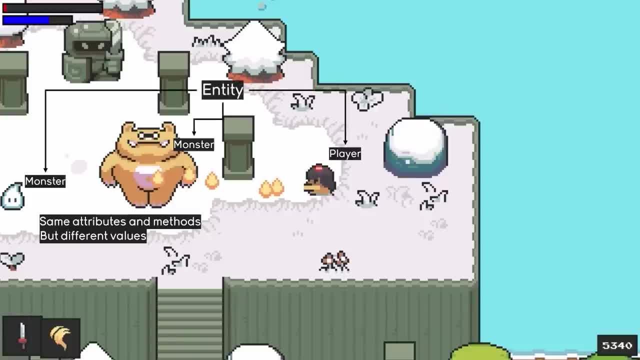 And what is really important to understand here is that all of these inherit from the entity parent class, And this, for example, contains the method for movement, Because all of the monsters and the objects move in the same way, So they could share this method quite easily. 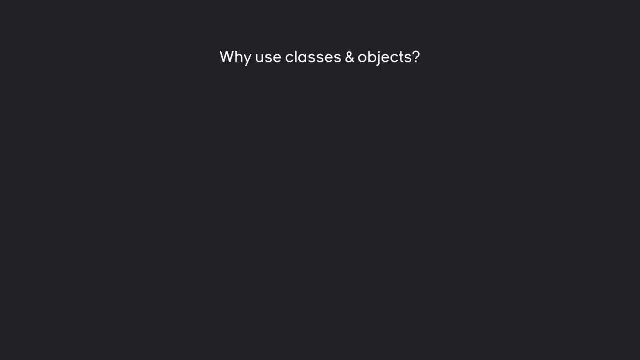 And just to emphasize it, I do want to go over the advantages of classes and objects, And the first point here is that classes and objects help you organize complex code, And the second point is related: Classes and objects also help you to create reusable code. 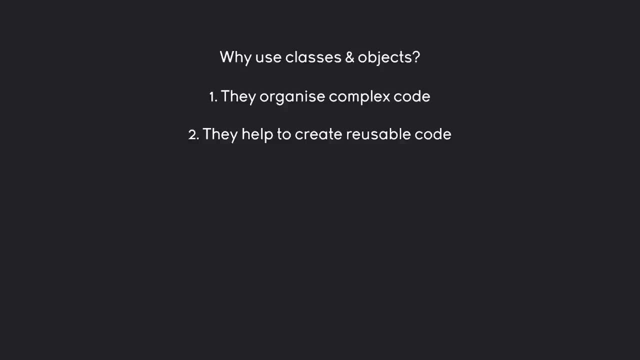 And just from these two points I hope it becomes obvious that if you want to create some really large project, let's say a really good looking game, you need objects and classes. Without them, it's still possible, but significantly more difficult. Besides that, classes are also used. 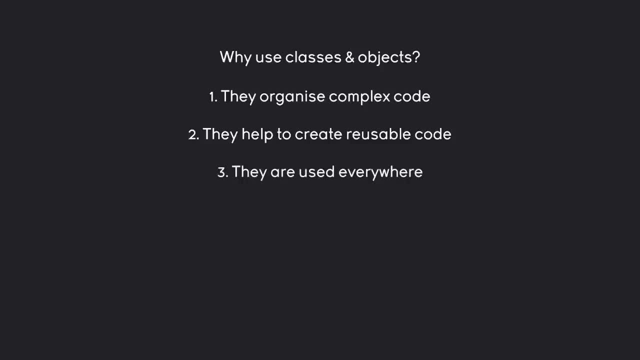 everywhere, Meaning if you don't understand them, you will be very much lost. As a matter of fact, in Python there are quite a few modules that require you to use classes, For example Pygame, Tkinter and Matplotlib, respectively the module you use for games, for GUIs and for data analysis. 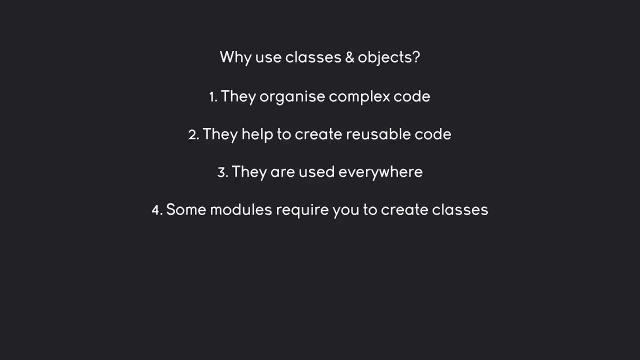 they all work with classes primarily. So if you don't know how to use it, you pretty much cannot use these modules, Or at least you could only use a very small part of them. And there's one more point that I haven't mentioned yet, And that is that classes make. 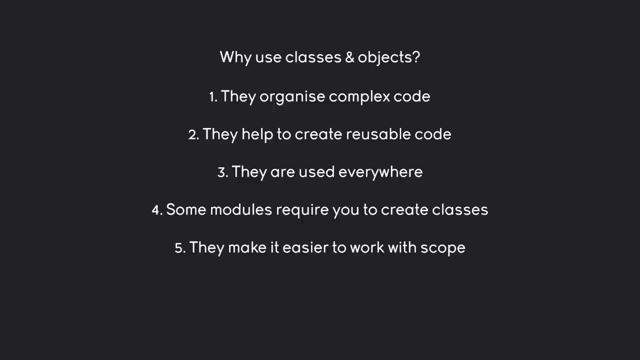 it much easier to work with scope. I will talk about this in more detail later, But if you have struggled so far with getting information in and outside of functions, you will really like classes. They make it very easy to work with different levels of scope. So these are the. 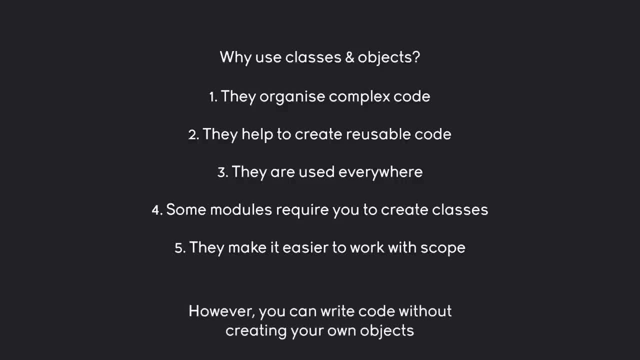 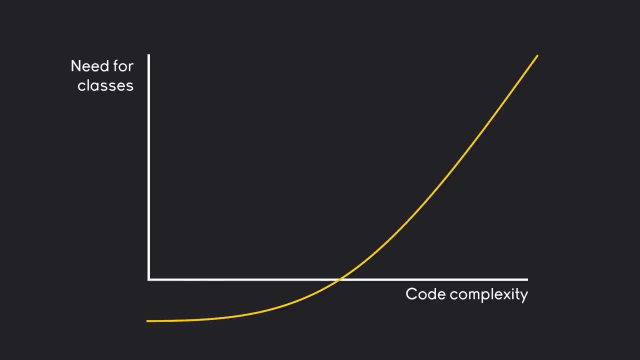 arguments why you would want to use classes and objects. However, you can write code without using objects at all, And this is very common, especially for beginners, And let me illustrate the problem here. The yellow line is the need for classes, And especially when you start writing code. 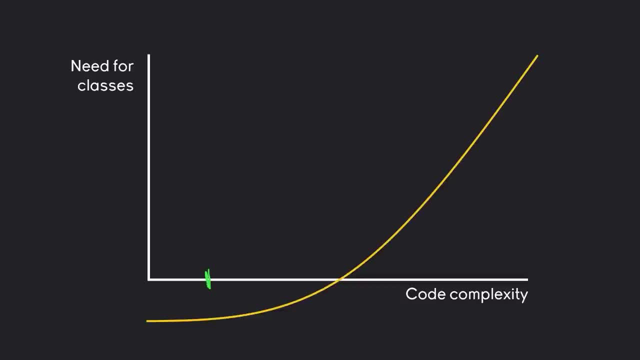 You are somewhere here And your average program is something like 50 lines of code. In this case, there really isn't any need for classes because, well, your code is very simple and there isn't any need to organize complexity. However, the longer and more complex your code is, 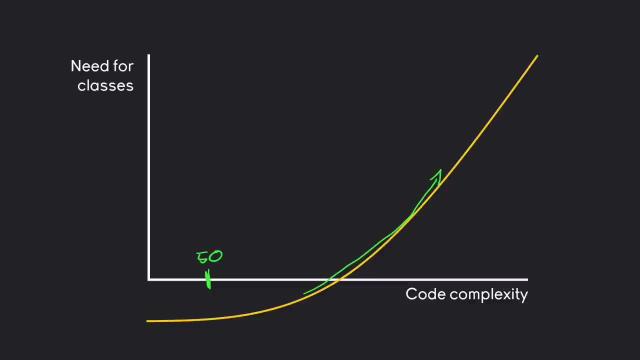 becoming, the more you will need classes, And this ramps up really, really fast. But as long as you are in this area, here, it is very tempting to never use a class and ignore them entirely, And this, especially as a beginner, you really want to avoid. So even though when you are here, I would really recommend you. 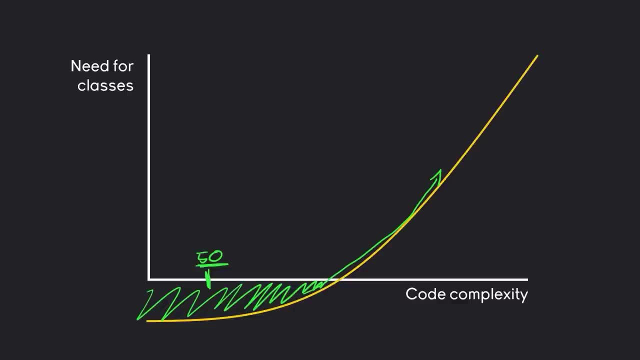 to use classes, even though it's not strictly necessary in your example, just to practice for more complex code, Because when you are an actual software developer, you are never going to write just 50 lines of code. Most of the programs you are going to work are somewhere here with a few. 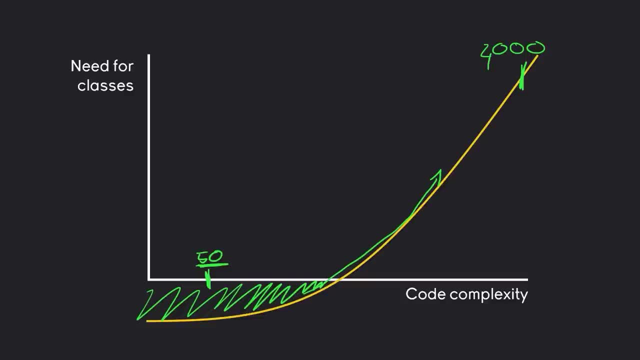 thousand lines of code, let's say 2000.. And if you are up here and you don't use classes, you are going to be in a lot of trouble. Alright with that. we have the theory of objects and classes And for the next part we are actually going to create and use objects. 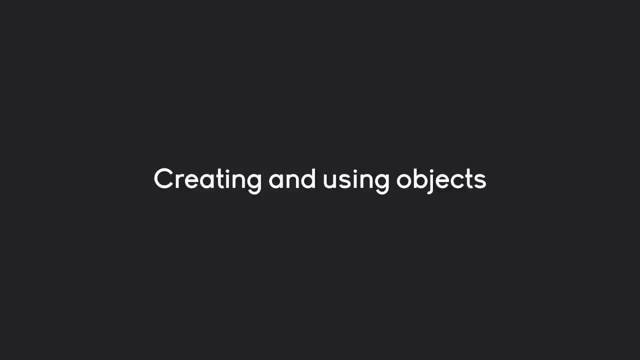 So let's have a look at some code Here. I have a completely empty sheet of code And the first thing I want to do is to create a class, And this you do with class and then the name of the class. In my case I want to go with monster, And here already we have to cover something. 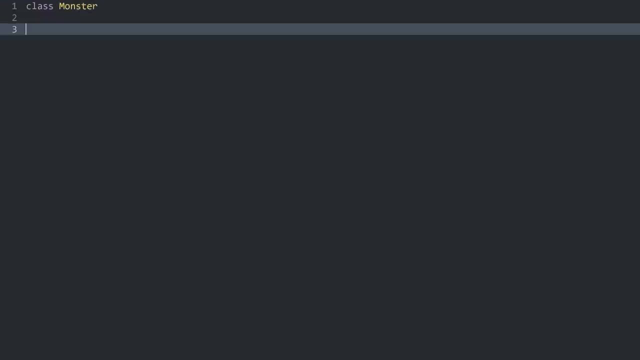 important And that is the naming scheme. So far, in Python, what you probably have written is something like monster, And generally you always used the snake case styling for any kind of text. So why is this different here? And well, in Python, by convention, last names are always written in the camel case. 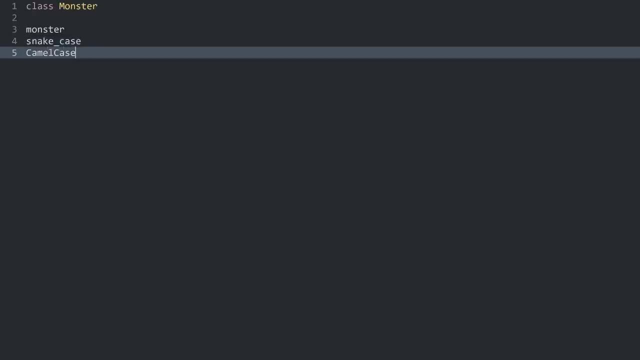 So camel case looks like this, where you don't have any spaces between words or, well, any underscores, But any word starts with an uppercase letter, And this is different from normal Python, where variables are written in snake case, where everything is lowercase and a space is an underscore. 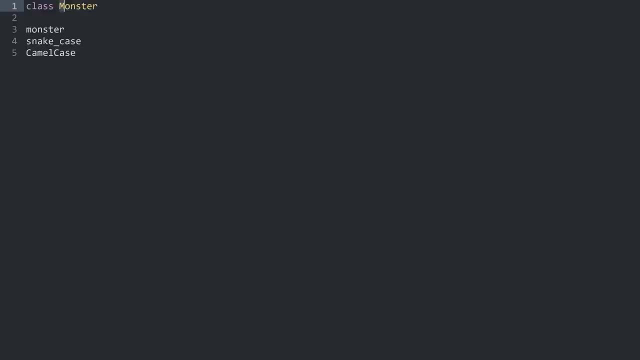 And this isn't so strictly necessary. you can call a class monster with a lowercase m, just fine. This is purely convention. But all the other Python requirements for naming still apply. For example, a class couldn't start with a number And we also couldn't have a space in between. 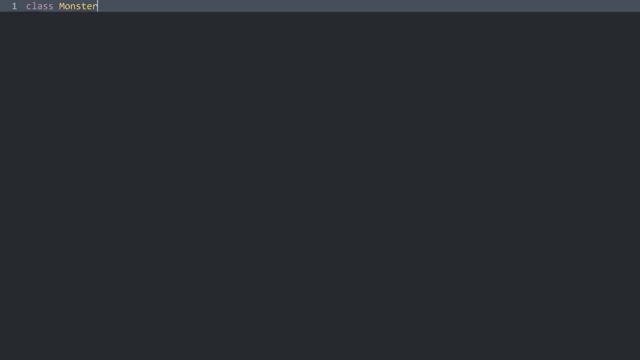 So we don't have to learn any new naming scheme Now. next up, what you have to do is a colon, And now in here we can work on the attributes and methods of our class class, And for now I just want to create some basic attributes. Let's say, I want to give this: 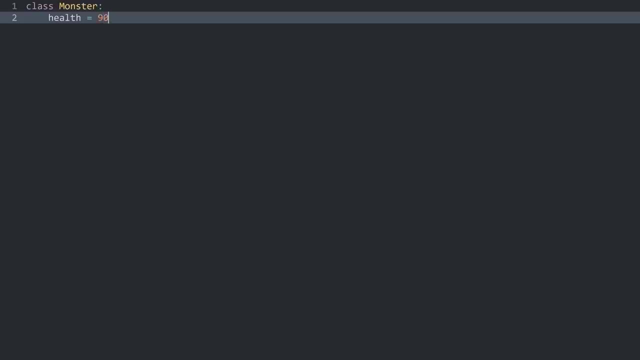 monster some health, And for now I want to have specific numbers, Let's say 90.. I want to have energy, And this one should be 40.. So now we have a class, And what we have to do now is turn this. 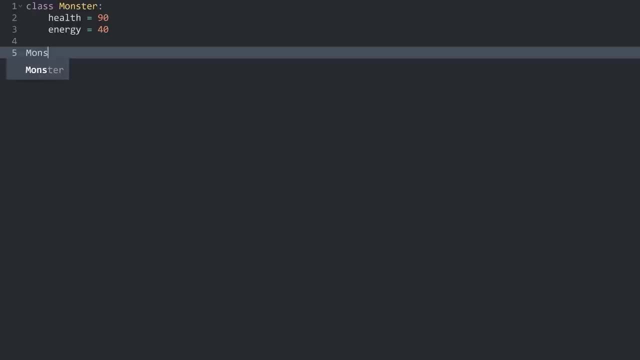 class into an object, And this we do by typing the name of the class and then calling it by using brackets- Again very similar compared to functions- And this is going to return the object. So we have to capture that in a variable And this very often is written like this: 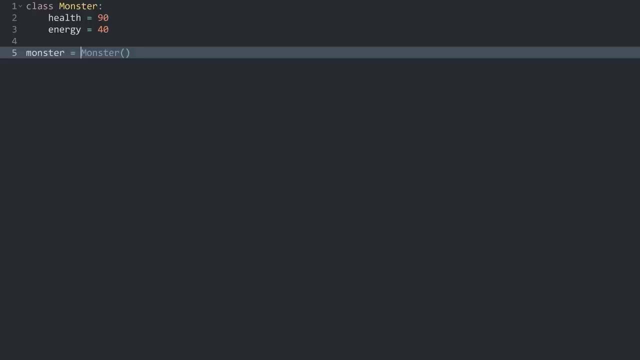 And here I hope you can see why we have the different naming schemes To Python. this name here and this name here are two completely different things, Because one starts with a lowercase, the other with an uppercase, Although to us, as the programmer, we can tell that those two are related. 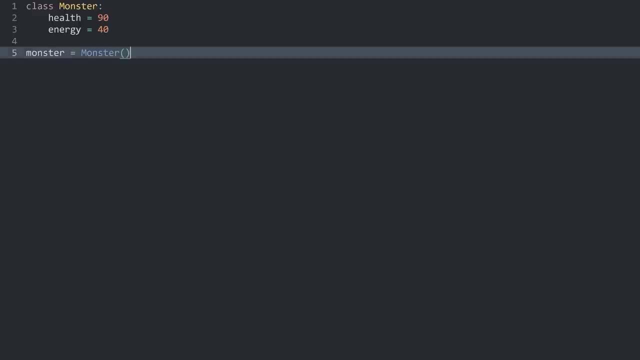 because they basically have the same name And for that reason we are usually writing class names in camel case, and variable names in snake case. It makes it very easy to connect these two and clearly indicate that they are connected, Although you don't have to do any. 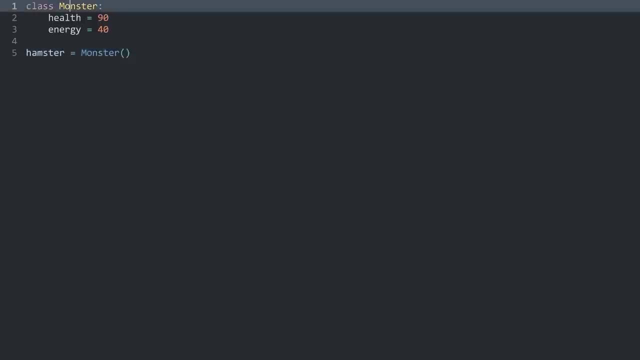 of this. You could totally call this- I don't know- hamster, And this could be lowercase. It's totally fine. All of this is just convention, Although you should follow conventions. they are there for a reason. But I can run the code now And I am not getting an error. That's a good sign. 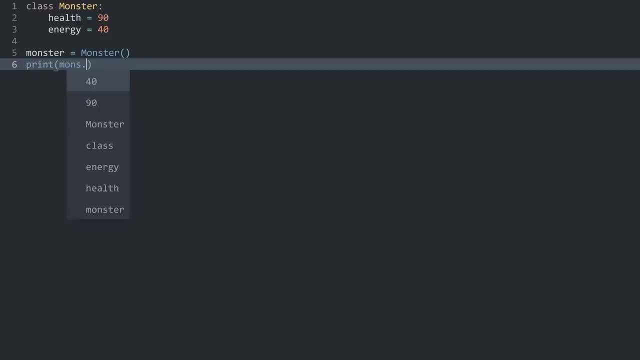 And now what I can do. I can use print and monster dot. let's say health. And now, if I run this, we are getting 90. And this 90 here is coming from this health, And the same would also work. 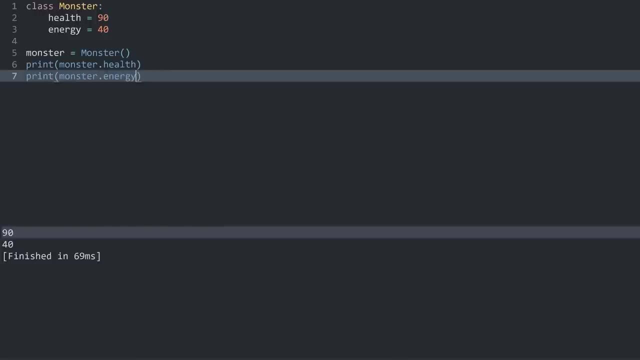 For energy in just the same way. So we get 90 and 40.. Now just to emphasize that both this health and this energy only exist inside of this class, Let me print health by itself. That is horrible spelling health, And if I run this, Python is going to give me an error And we have name health. 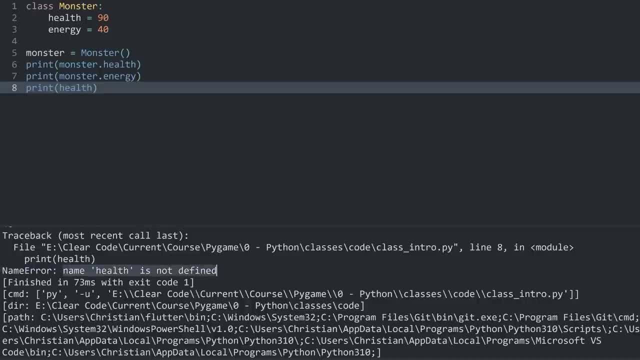 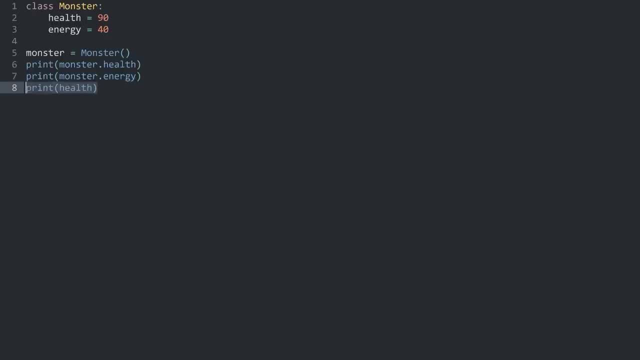 is not defined, Meaning Python cannot find this health. So we get health in the global scope, Which makes sense, because there is no health in the global scope. We only have health in the scope of this monster class. And let me add some comments here. 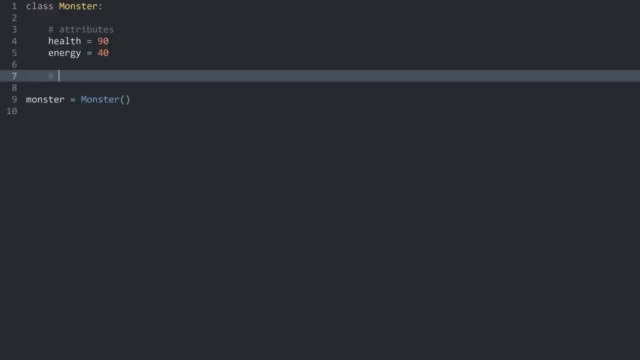 to make this a bit more readable. We have attributes And besides that I also want to create methods And those work kind of like functions. we again need the define, keyword or def, And now we need a name for our function And for that we have the exact same naming scheme for normal functions. 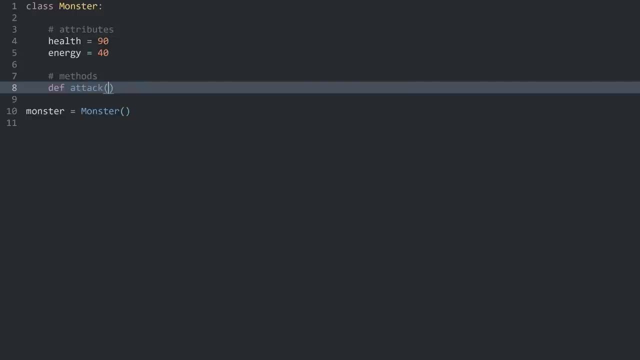 For example, attack would be a perfectly fine name, And after that you need a colon. And then let's say: for this attack method, I want to keep it simple and just print: the monster has attacked And now I can call monsterattack. 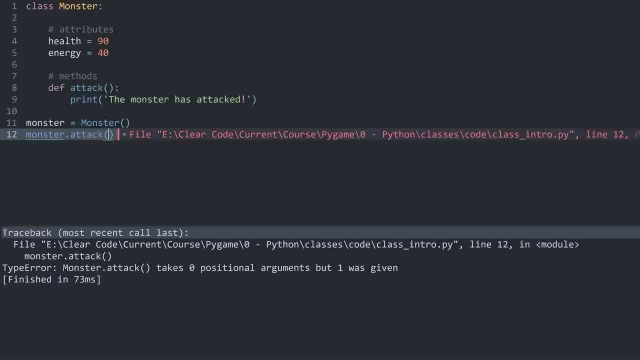 And don't forget the brackets. And now, if I run this, we are getting an error, And this error says that monsterattack takes zero position arguments. but one was given, And this is probably very confusing, Because when we called this method here, 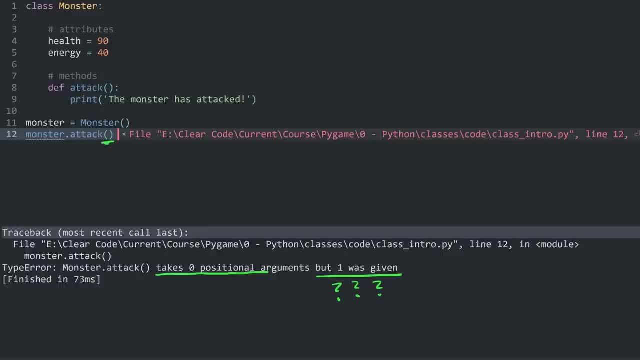 we didn't pass anything inside of it And the method itself doesn't have any parameters. So why is Python being so weird here? Now, the reason why this is happening is that whenever we call a method, so a function inside of a class. 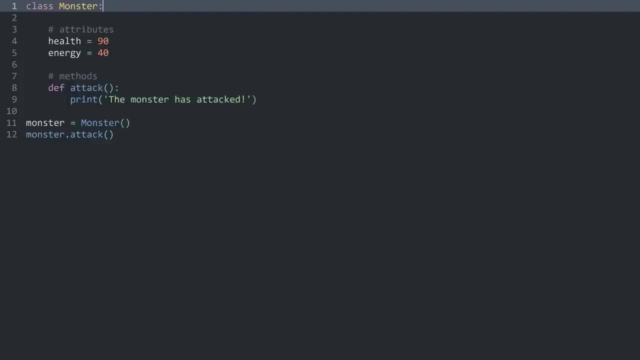 what is going to happen is that Python automatically passes a reference to the class as the first argument into this function or this method. to be more specific, And this first argument we always have to capture with some kind of parameter Meaning. a method always needs at the very least one parameter. 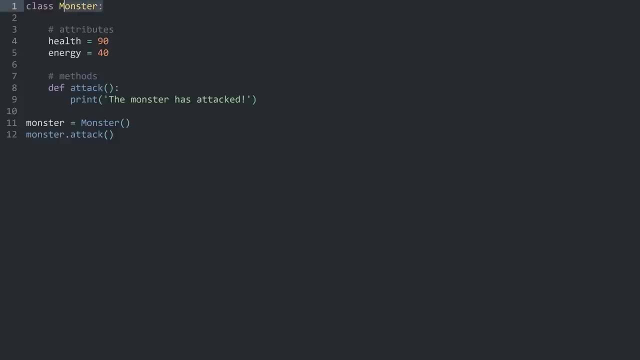 And that parameter is a reference to the class itself. For example, I could just write monster in here And if I run this now we get the monster has attacked And let me just print what we actually get. So I want to print the monster we get as an argument in here. 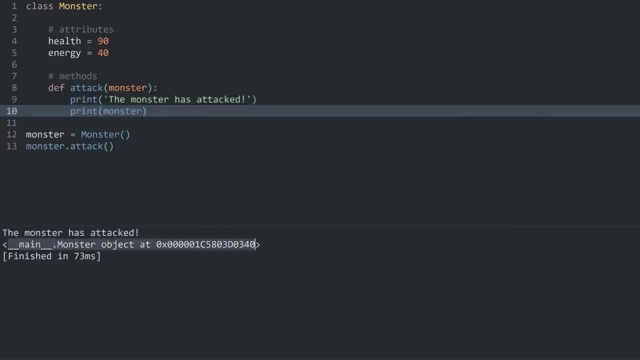 And what we get is main monster object at somewhere in our memory, And well, in my case, I don't really care about this monster. So let me remove the print statement, But I do have to keep this first parameter. However, once we have the first parameter, 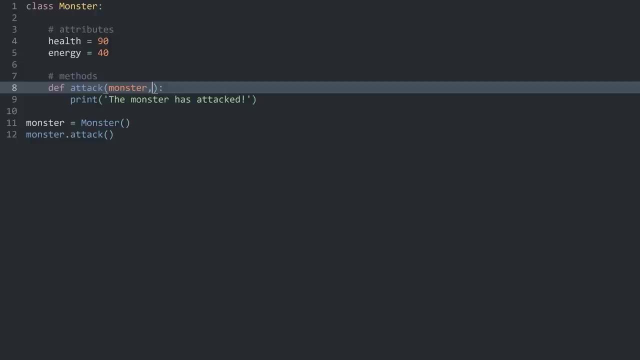 I can add as many custom parameters as I want. For example, I could add the amount of damage here And I could, let's say, print the amount with an F string And I want to say the amount of damage was dealt. 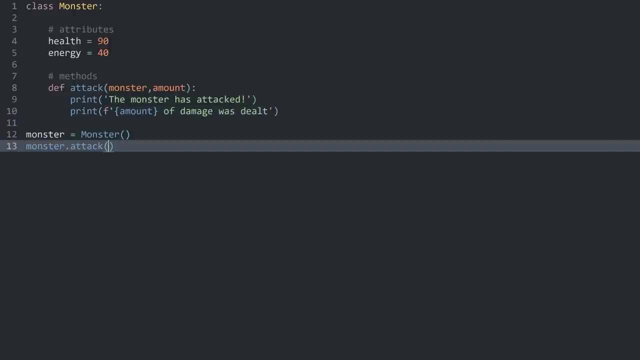 And now when I call this method down here, I can pass in any number I want And I get. the monster has attacked. 40 of damage was dealt. That does not make sense in terms of grammar. Let's try this again. 40 damage was dealt. 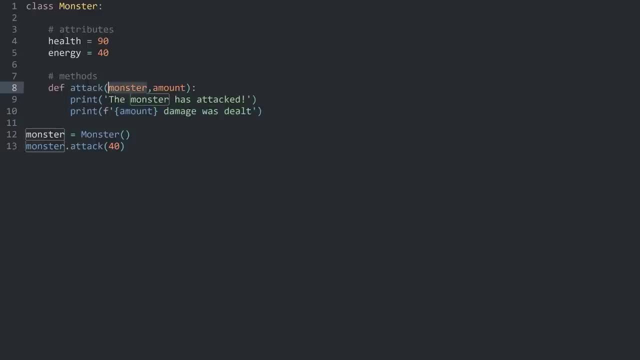 That feels much better. So the one thing you want to remember is that, for any kind of method, you always need a reference to the actual class As the first parameter, But after that you don't have to worry about it anymore And you just use it like any other function. 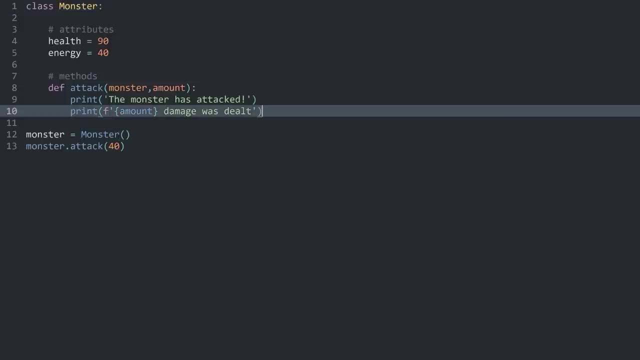 However, you could also use this reference to the class. What you could be doing, for example, is print- And let me just print- monster dot energy. If I now print this, I get 40 again, Meaning this: monster energy here. 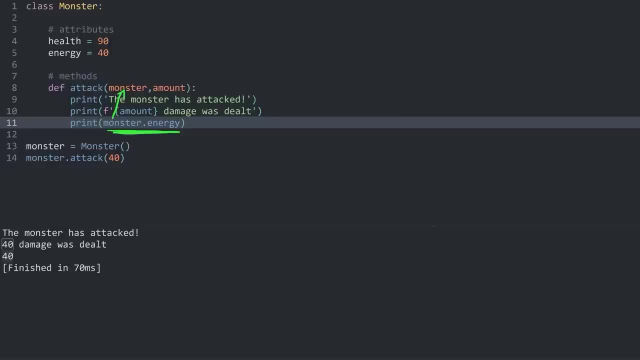 is looking at the first argument it gets, And this is a reference to the class itself. So from there we can get this energy and also this health, if you really wanted to, And what you could also do is increase this amount. So monster dot energy minus equal 20.. 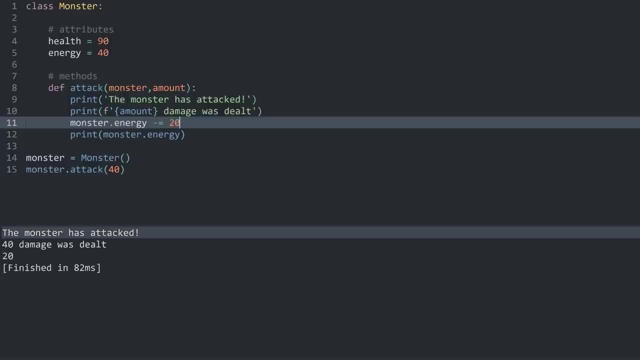 And if I print it now, we get 20.. And I hope you can tell how useful this can be, Because if you imagine that this monster here is the global scope And these attributes are global variables, If this attack was just a normal function, 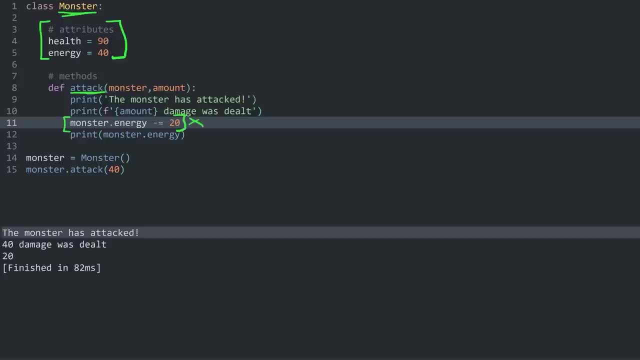 then this would not work Because you would be creating a local variable that wouldn't work with the global ones. But because of this first argument that the method always gets, we can influence variables or well attributes outside of this function, Which is incredibly useful. 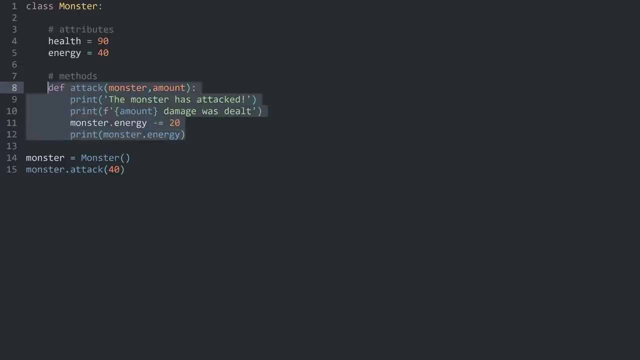 So I hope this kind of method here makes sense. As a matter of fact, let's practice this one. I want you guys to create another method for this monster, And this one should be called move And it should accept one argument besides the reference to the class itself. 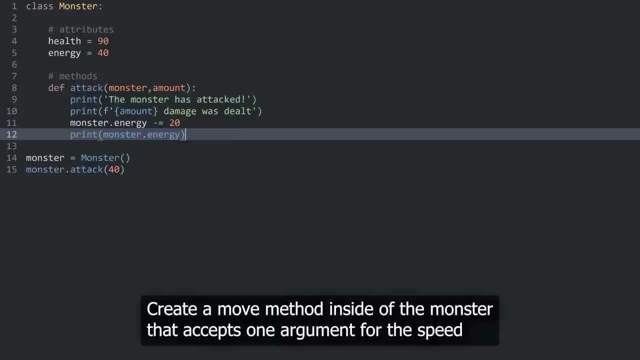 And that is the speed of the movement. And then, inside of the method, you should just print that the monster has moved at a certain speed. It doesn't really matter what you put in here, as long as it is working. So try to figure this one out yourself. 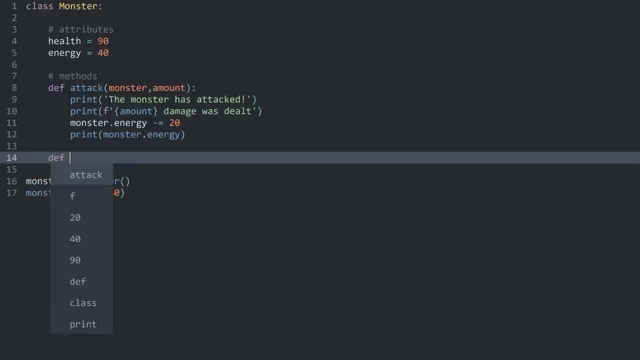 Alright, let's try it together. now. I want to create a method called move, And in here I want to have speed as a parameter. However, what we have learned from the attack method is that we always need a reference to the class itself. 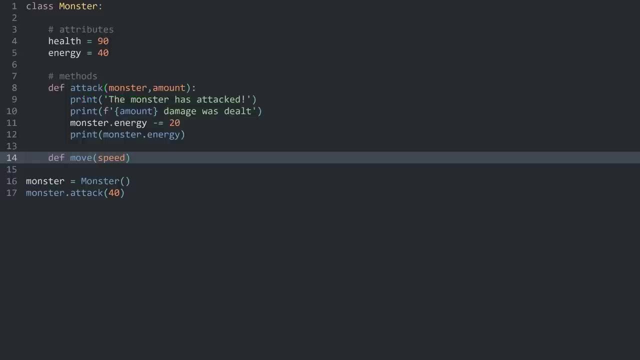 as the first parameter, Meaning, the first parameter here should be something for the monster, And it really doesn't matter what you call it. So I could even write something in here, It would still work. And now in here I can print: the monster has moved. 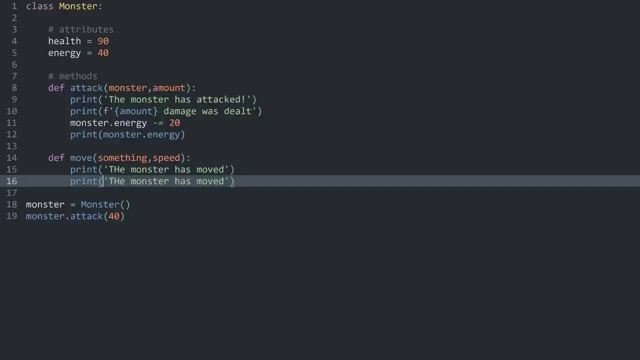 And let me add another line with an F string That says it has a speed of and then the speed. And let me fix the typo And now I can call monstermove and add, let's say, 10 in here. And let me comment out monsterattack. 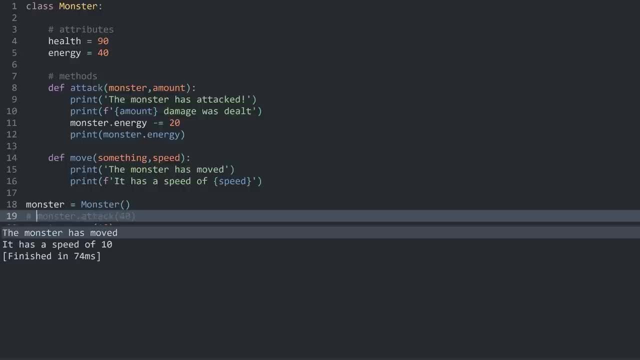 And let's see what we get. The monster has moved, It has a speed of 10. So all of this seems to be working just fine. So, all of this seems to be working very nicely. Now, obviously calling this first parameter something. 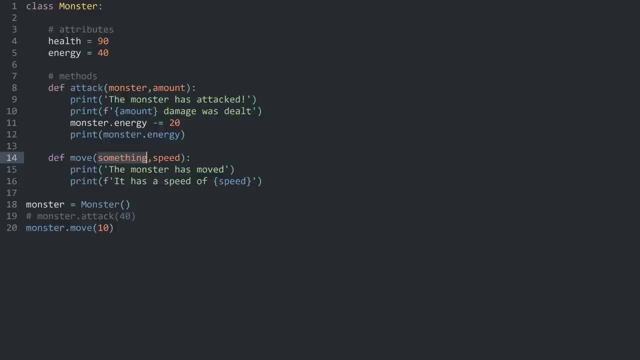 is a bit confusing And, as a consequence, in Python there is a convention that this first parameter is always called self, And this applies to all of the methods, Meaning this is what you are going to see most of the time and what I am going to use as well. 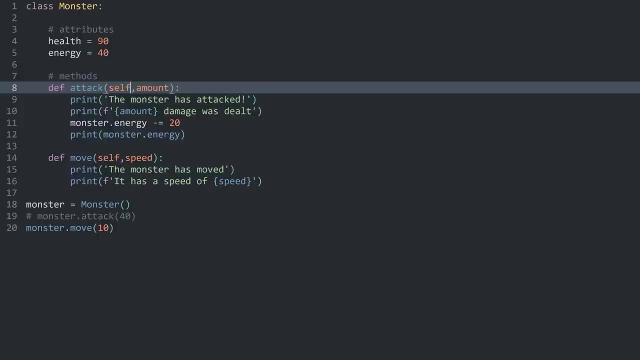 You don't have to do it, but I think it makes the most sense, Although I do want to emphasize that this parameter here and this parameter here have no relation whatsoever. They are entirely separate, Although, that being said, they both reference this monster class here. 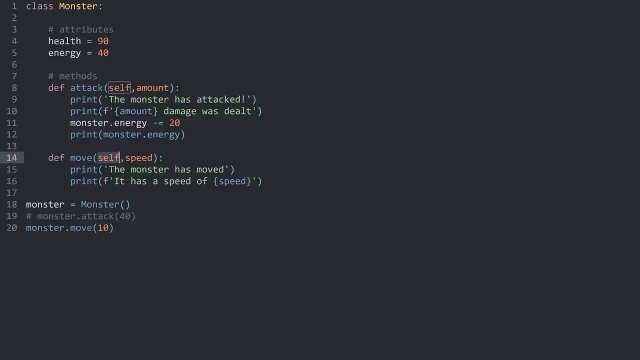 But it is totally fine to call self here and self here. The names are not in conflict with each other And alright with that. we have the very basics of using classes and objects, Although right now we do have a problem. 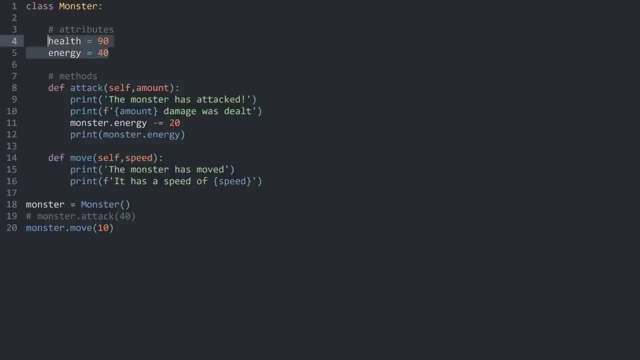 That our monster always has the same health and the same energy. So even if we created multiple monsters- So what I could be doing is monster1,, monster2, monster3- and let me get rid of this one here- All of these monsters would have the same amount of health. 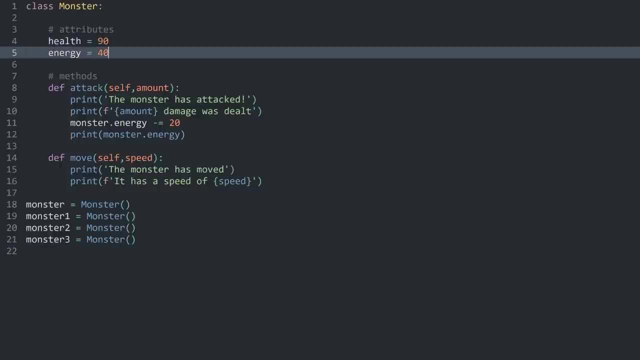 and the same amount of energy, And they all have the same attack and move method, Which is fine to an extent, but I do want them to have different amounts of health and different amounts of energy, And to implement that we need another concept. 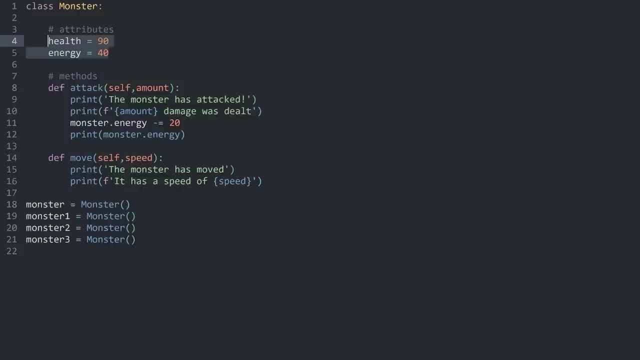 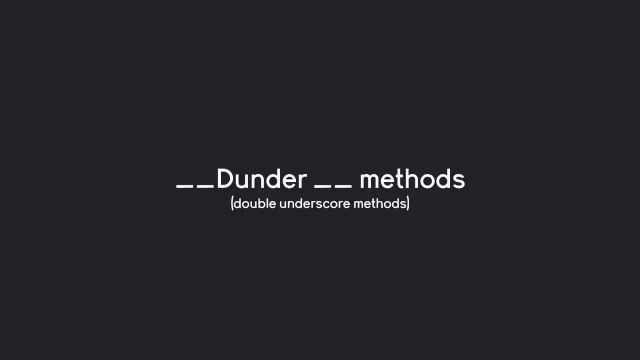 And that is called Dunder methods. So let's talk about that one. Let's talk about Dunder methods. And the Dunder here just stands for double underscore Meaning: we are talking about a double underscore at the beginning and at the end of the method. 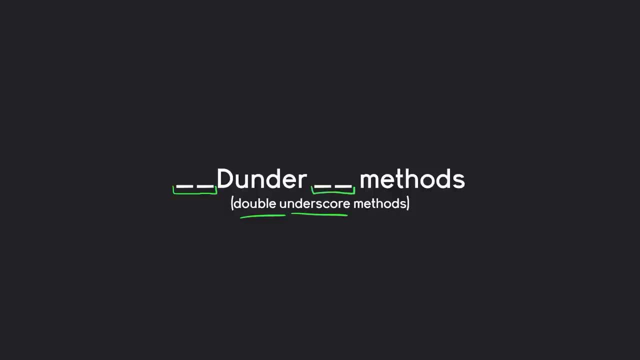 But it's important here we are still talking just about methods. So essentially we are calling a specific kind of function And let's talk about why it's special. A Dunder method is just another method, The thing that makes it special. 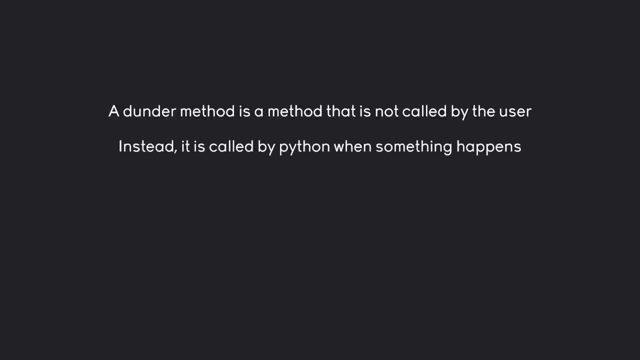 is that it is not called by the user. Instead, it is called by Python when something else is happening. For example, there is the Dunder init method, And this one is called when the object is being created. Another example is the len method. 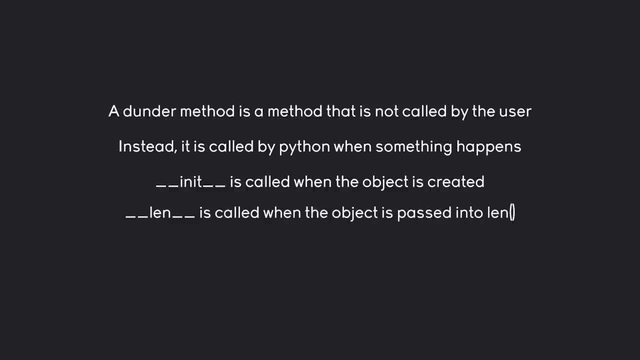 And this one is called when the object is passed into the len function. And besides that, we also have Dunder apps, And this one is called when we are passing the object into the apps function. And that is really the entire idea. It honestly isn't that complicated. 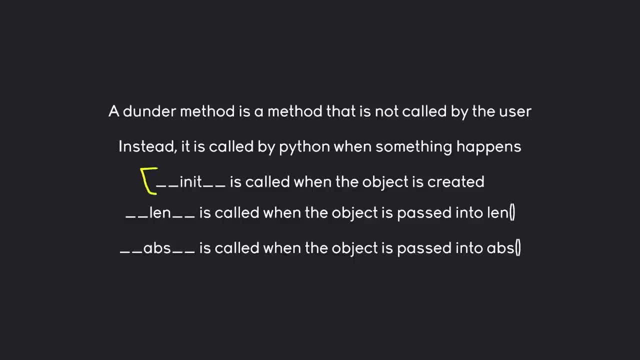 The most important Dunder method you have to understand is Dunder init, This one you are going to be calling all the time, But let's actually do all of this in code. that should make the most sense. Alright, here we have the class I created earlier. 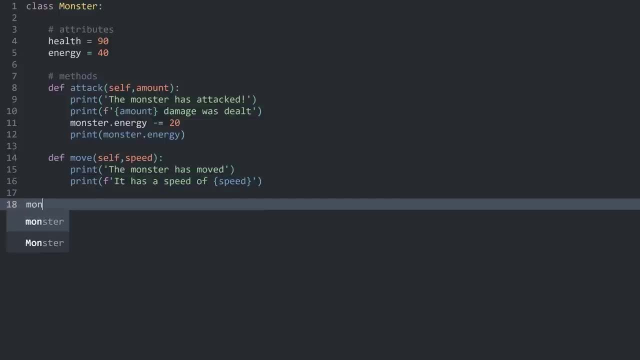 And what we have seen earlier as well. I can create monster1., And that is just going to be the monster, And I can also have monster2.. And if I now print monster1.health and monster2.health, we get the same number. 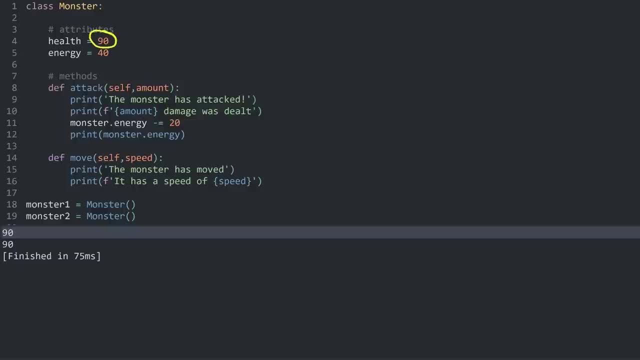 Because we always set health to 90. There is no way to customize it And basically, what I want to do is, as soon as the class is being created, then I want to create these different attributes, And instead, what I want to do is when this class is being created. 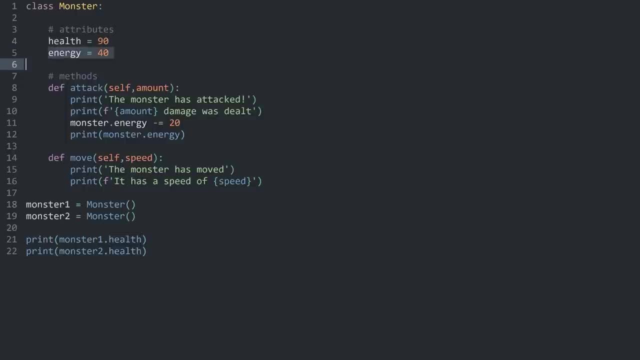 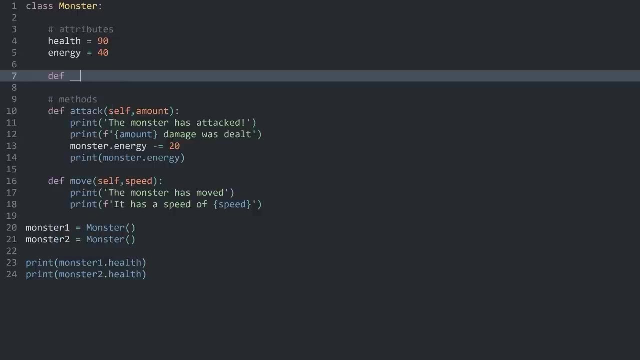 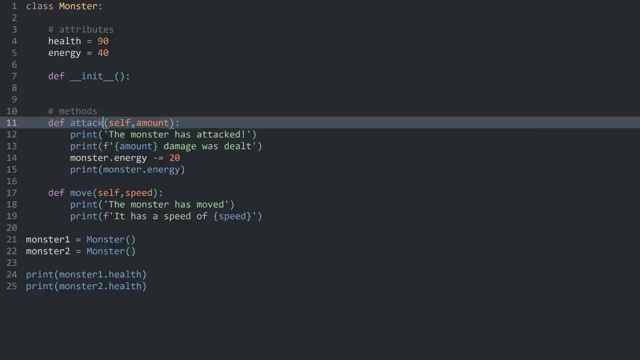 I want to create this health and this energy with custom values, And for that to work, we need to define a Dunder method, And the one we need is called Dunder init, And this is just going to be another method, Like attack and move. 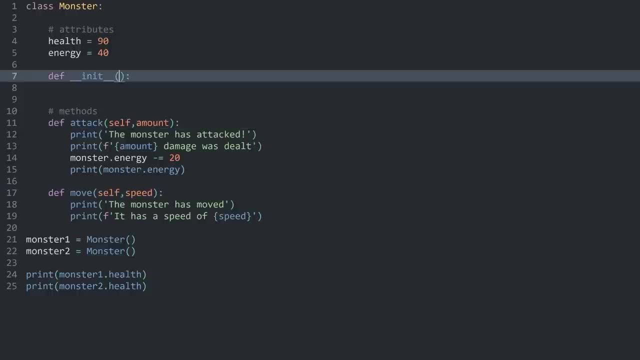 we are just calling a method, Meaning the first parameter here has to be a reference to the class itself, And for now let me just print: the monster was created. And do pay attention, I am never calling the init method myself, But if I run this 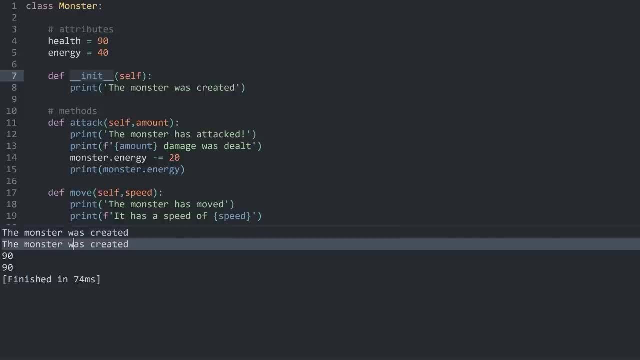 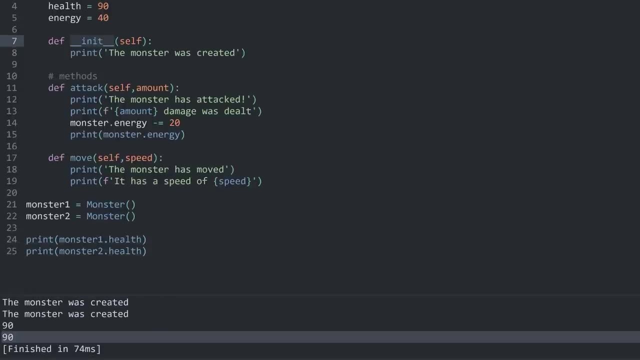 we get: the monster was created, the monster was created, and then 90 and 90. And what that means, if I minimize this a bit, every time we are creating a monster. so first here and then here, then we are calling this Dunder method. 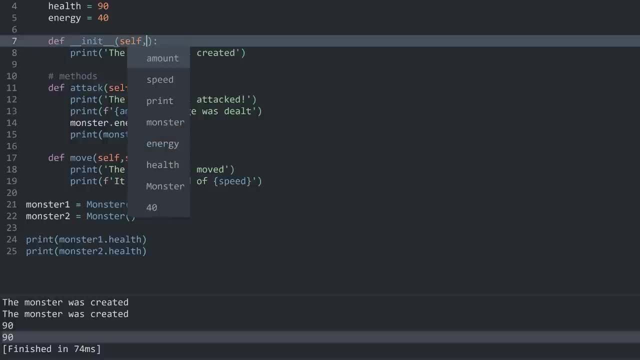 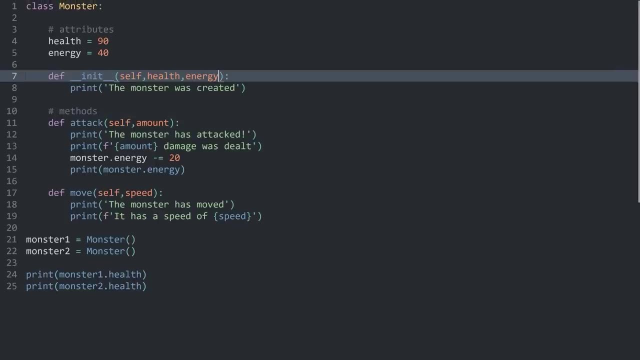 And this Dunder method. we can also give some parameters. For example, we could specify in here the amount of health and the amount of energy we want. And well, I hope you can see where this is going, Basically what we can do now. 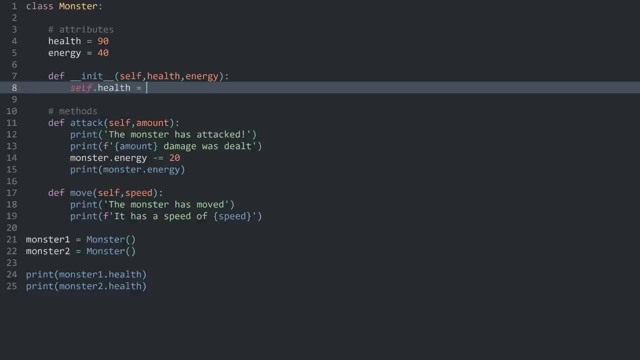 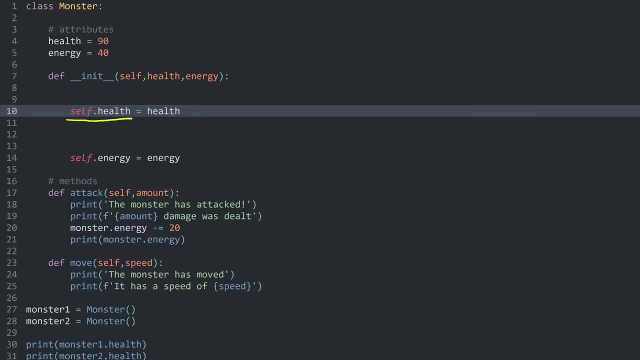 is, we can set selfhealth to whatever health parameter we pass in, And we can do the same thing for energy, And the names here might be a bit confusing, So let me add a bit of white space and explain This. selfhealth here is referring to this selfhealth. 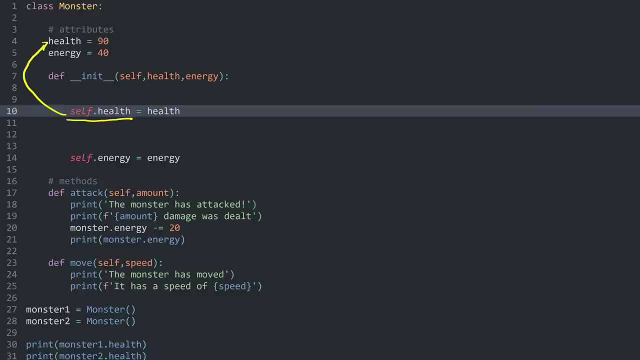 of the monster class, Whereas this health here refers to this parameter And the important point here is self, because this one specifies where health belongs to. I hope this makes sense. This is something you see fairly often. Let me remove the white space again. 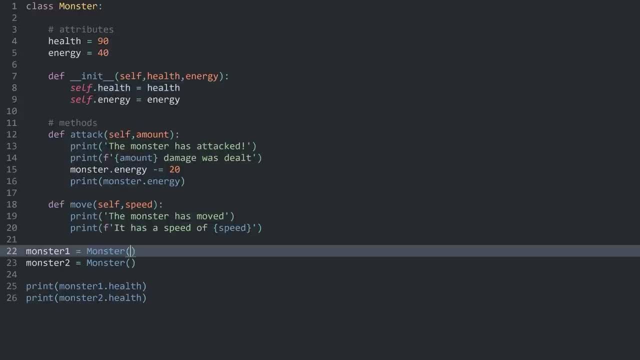 And now, when I am calling the monster, I can either pass in arguments or named arguments. Let's say, for the first monster, I want health 10 and energy 20. And for the second monster, I could specify health being 50. 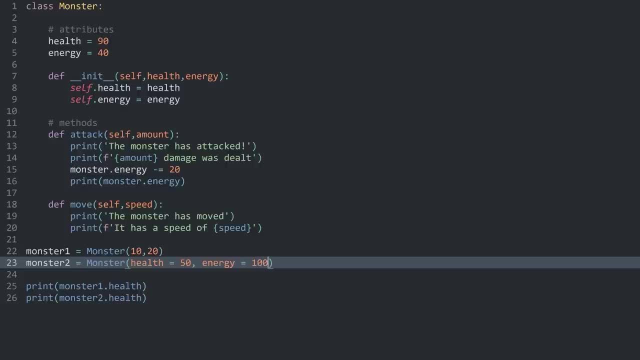 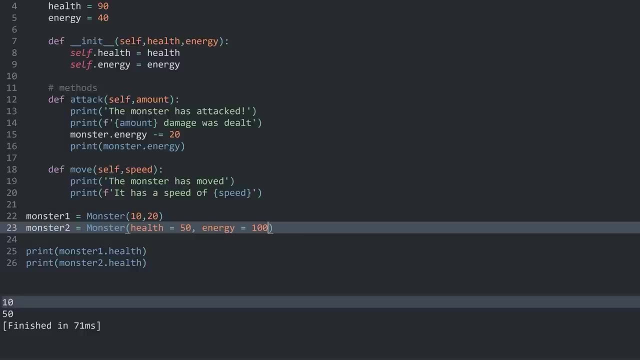 and energy being 100.. Now if I run all of this, we get: monster1 health is 10 and monster2 health is 50. And this 10 here refers to this 10 and this 50 is referring to this 50 here. 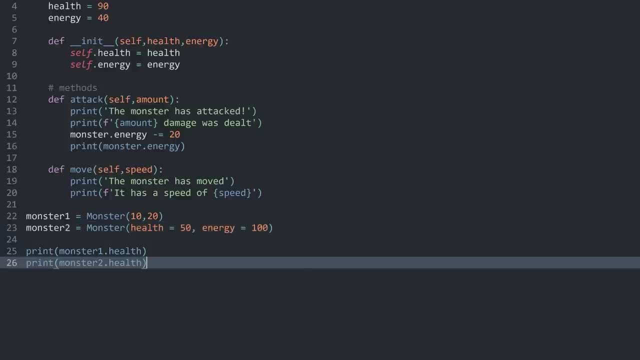 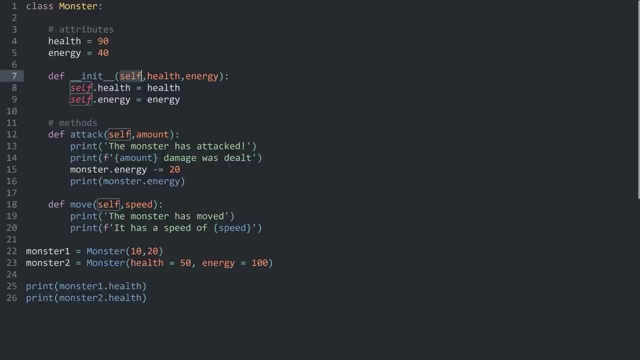 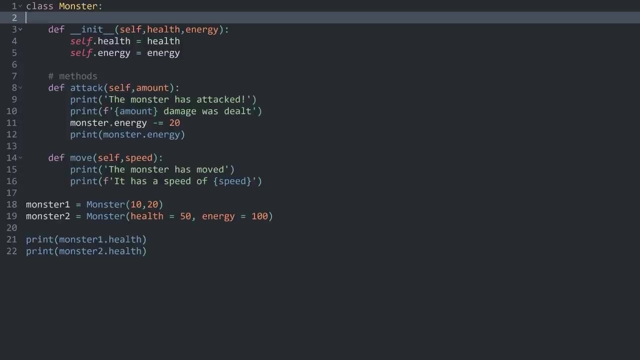 Meaning. now we can have custom attributes And what is even better, since this self is a reference to the class itself, we can just create the attribute in here, Which means we don't need those lines at all. It would still work without them. 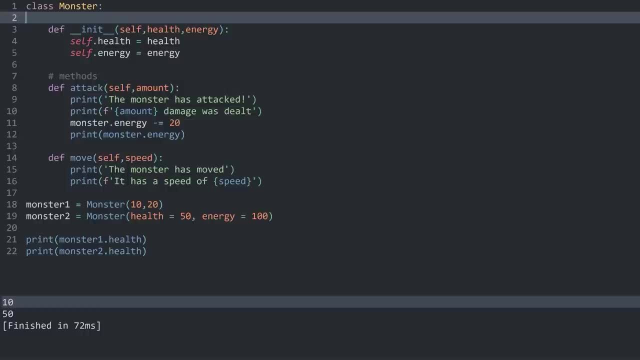 If I run this now, this is still working just fine, And this is what you see most of the time where the class by itself doesn't have any attributes. We only create attributes when we are creating the class with the init method or the dunder init method. 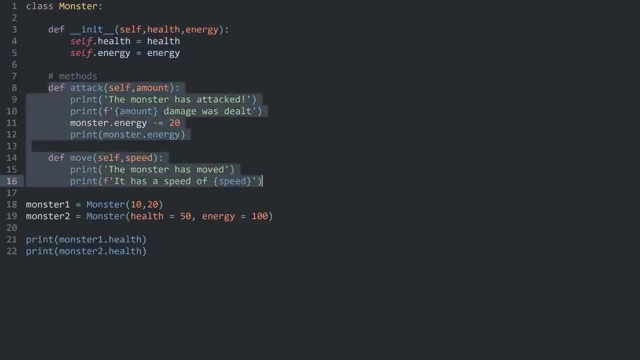 And then, inside of the other methods, we are calling self all the time to refer to the class, And I just realized this should be self instead of monster. So we're capturing this self here And what you are going to notice is that you are going to write self. 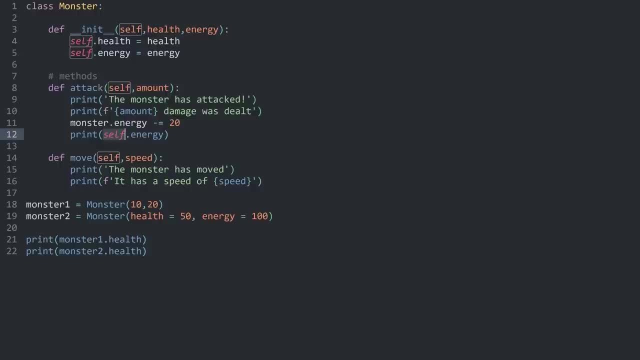 all the time, Which is a little bit annoying, but it is manageable. And with that we have the first init method, But there are quite a few more, although those you wouldn't use that often. And just to keep things simple, 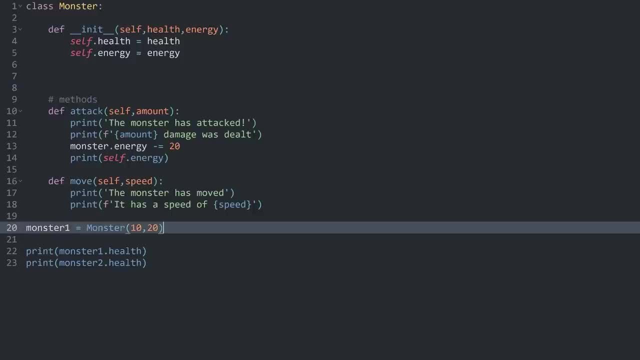 let me get rid of monster2, and I don't want to print anything at all. Another dunder method I talked about in the introduction is len, And this one needs self and no other parameters, And in here we just want to return something. 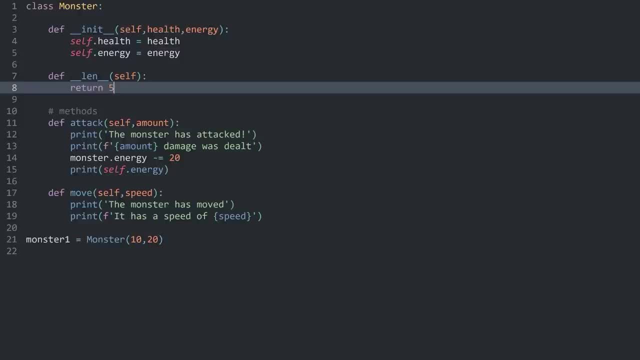 Let me return the number 5. And what this one is going to do is if I call len and pass in monster1 in there And this len, just as a quick recap, if I pass in any kind of string into len, let's say test, 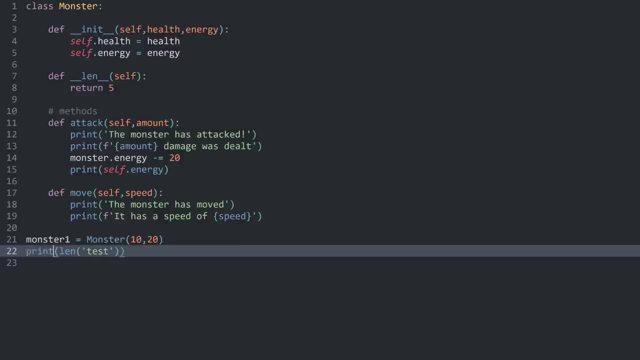 and if I print the result I get 4 or the number of characters inside of the string. I guess I could also pass a list in here that might make a bit more sense. So I have a list with 5 entries and the length of it is 5.. 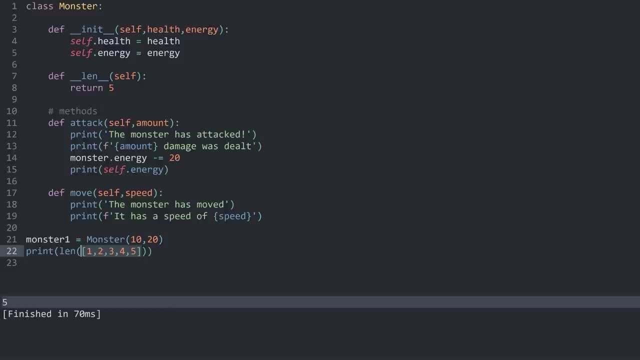 But what I can do now. if my monster has a len method, I can pass monster1 in here and it's going to be passed into the len function And it would return 5 as well And any number that is being returned here. 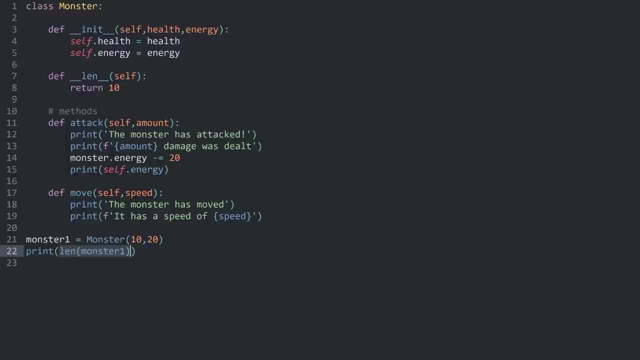 is going to be passed into the len function And I guess, for something slightly more relevant, instead of returning a number, I could return selfhealth, And now if I run this, I'm getting 10 or the amount of health my character has. 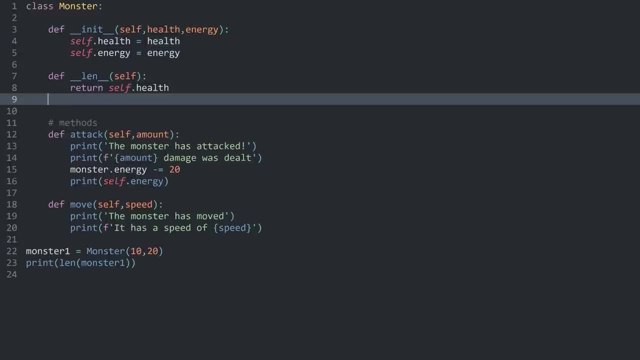 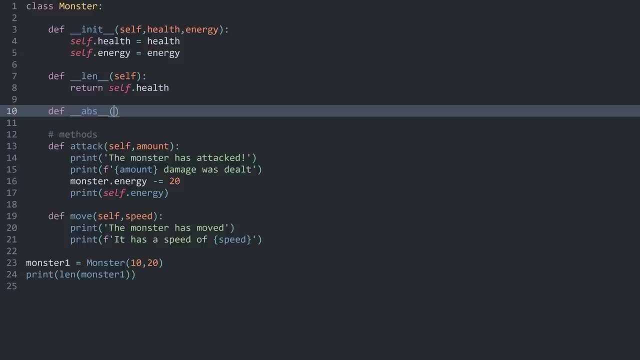 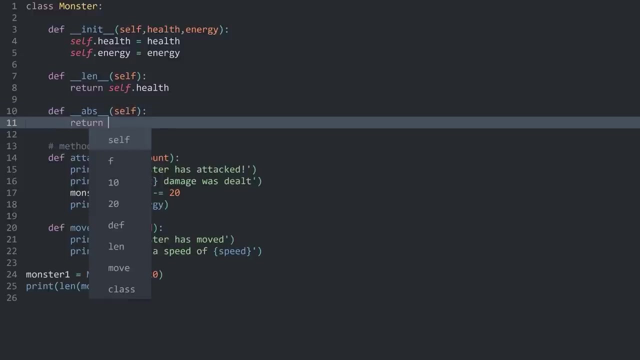 which is 10 right now, And another example we have seen in the introduction that works in the same way is abs, And we need dunder on both sides and in here self, And again I have to return something, So return, and for this case, 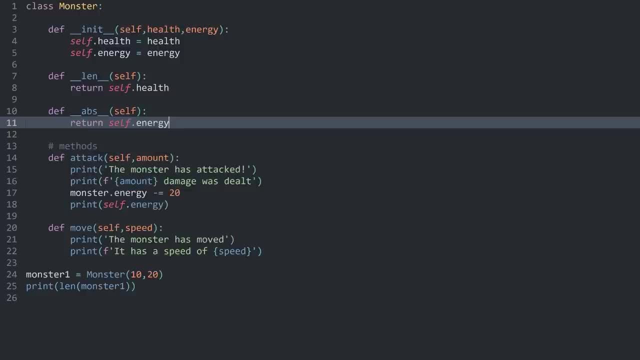 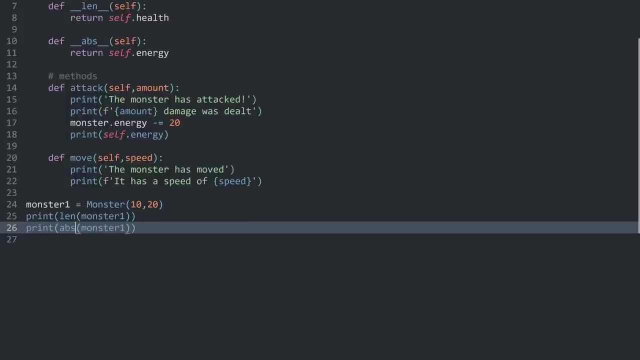 let's say selfenergy, And if I copy this and pass it into absolute, I get 20.. Now, usually absolute is if you have a negative number and you want to make sure it's always positive, That's what it does, But well, 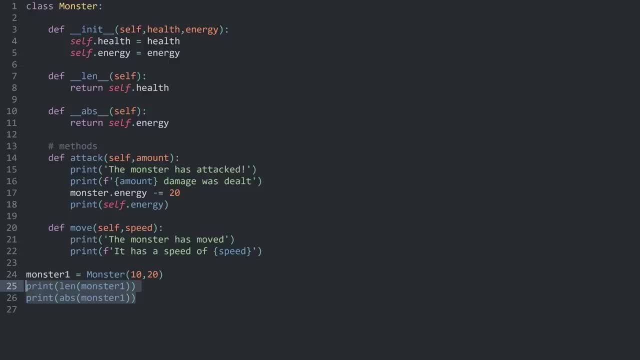 you could theoretically do whatever you want with it. Now, what you can also do is one specific function in Python, And that is called dir, short for directory, I think, or directory listing or something like that- Basically what it does: you pass in an object. 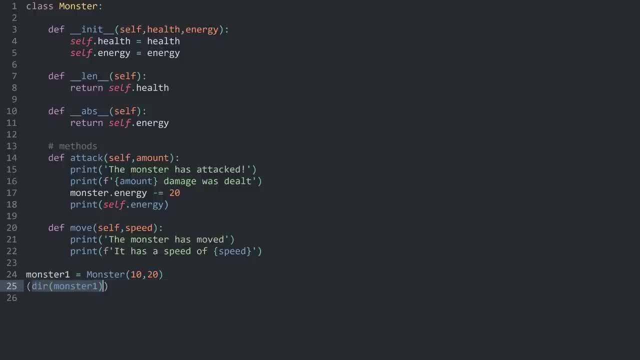 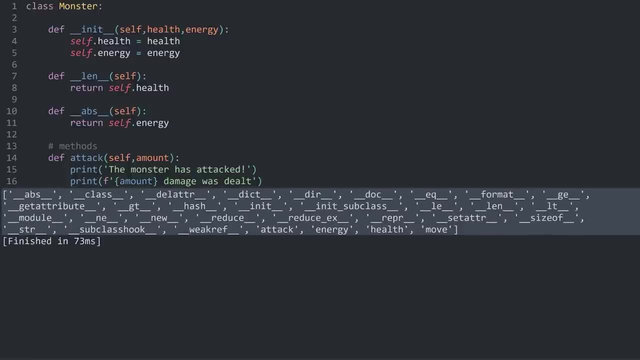 and then you want to print the result And what you get from that is all of the dunder methods and, at the end, the attributes and the normal methods, And in here you can see a lot of stuff actually And what you have to understand here. 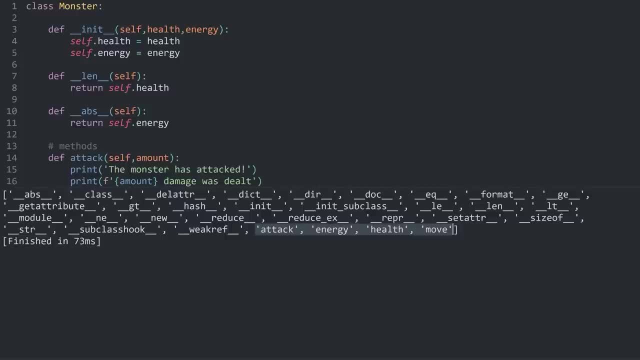 is, every time we are creating an object, Python already gives it some dunder methods. For example, here we can see the dir method, And this one is necessary for the dir function to work. It kind of works like the len method, the one we have created ourselves. 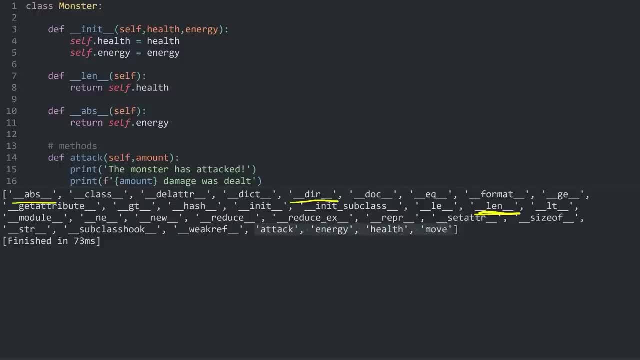 or the abs function, And I guess the one we have just created is the init method. This is the really important one, And most of those you really don't want to worry about because, well, they're just there to make the class work. 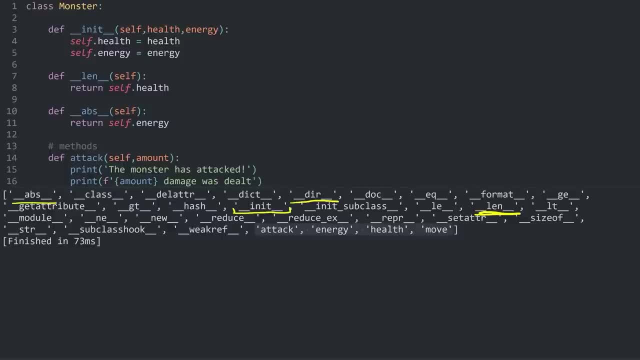 but we don't really have to worry about them, Although some dunder methods in here can be very useful. For example, dunder dict is well, it's kind of a dictionary, but not in the way you would expect Basically. 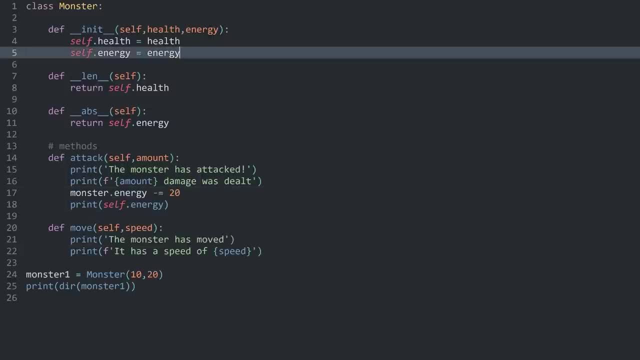 how you would use that one. Let me print it right after the monster. I want to print monster1 and then dunder dict. And in here, this is the one exception where this is not a method, this is just an attribute. 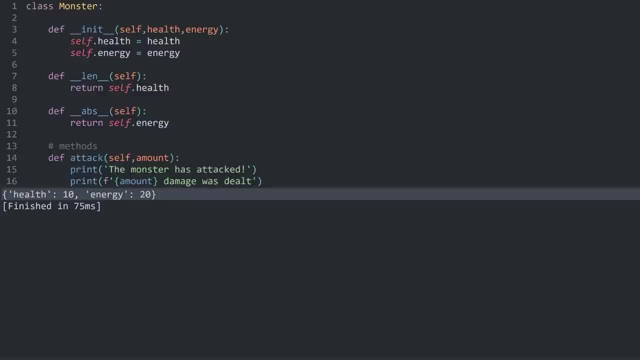 So no brackets afterwards. And this one gives us all of the attributes of the method inside of one dictionary- Can be quite useful sometimes, although you wouldn't be using it too often Now. another way to get to this dict here is to: 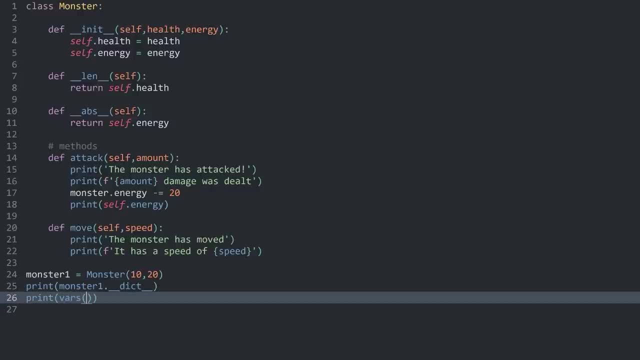 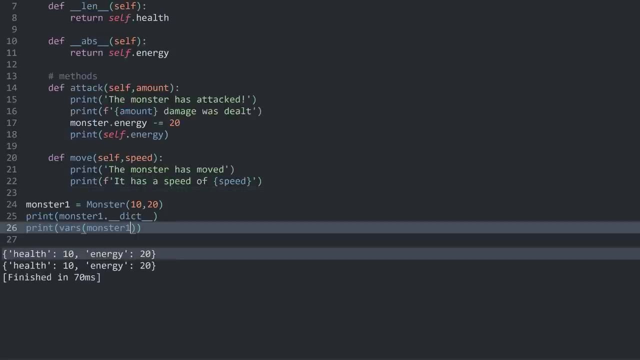 let me duplicate the entire line. You can call the vars function and pass in monster1.. And this one is giving us the very same thing, Although I have hardly ever used either of these. Most of the time, you just don't need them. 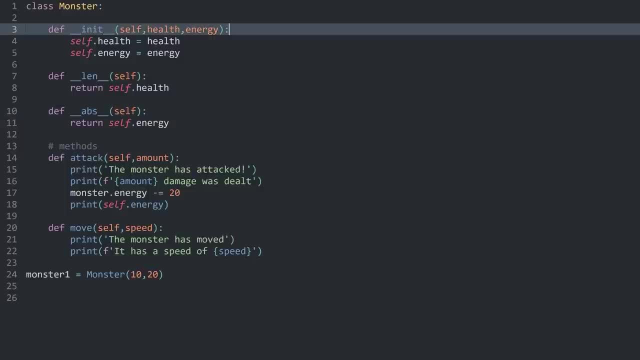 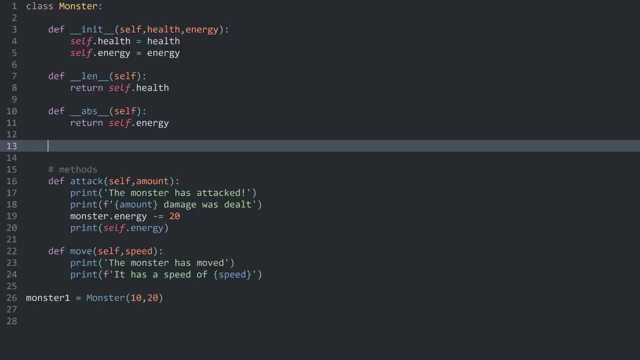 And with that you should understand dunder methods reasonably well. Now there are quite a few dunder methods that get a bit more advanced. I only covered the really fundamental one. Some other examples of dunder methods is, for example, dunder call: 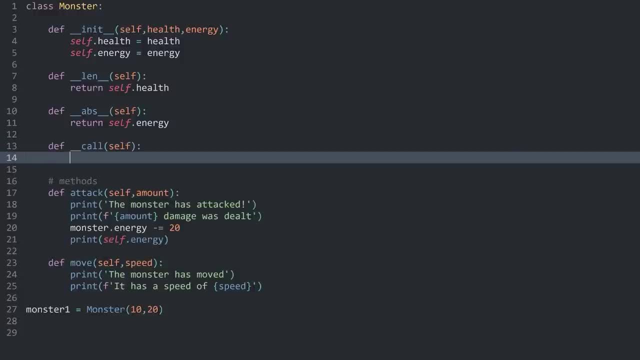 And in here we only need one parameter: self, And in here we can return something else again. And let me, this should be dunder on both sides. Let's say, the monster was called And what this dunder call does. 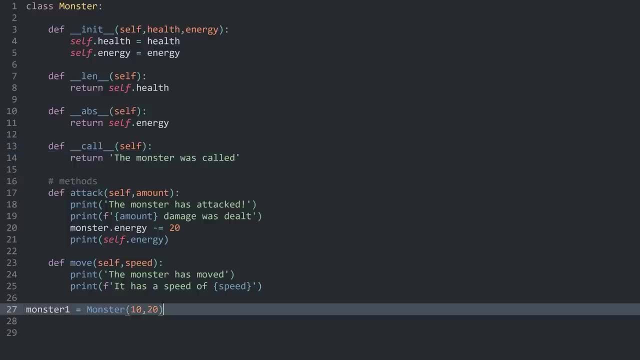 is. it essentially turns our object into a function, meaning I can call monster1 and then add brackets afterwards, And if I do that we are not getting anything because I would have to print what I get, So I have to put brackets around it. 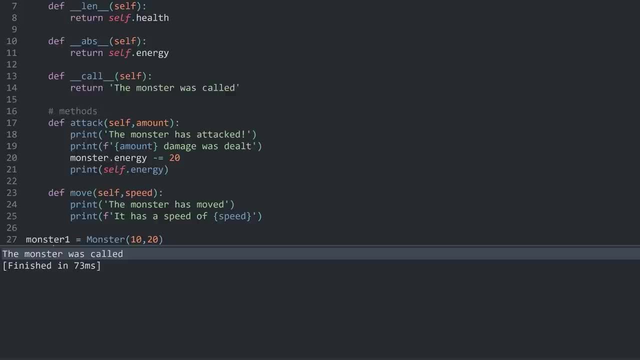 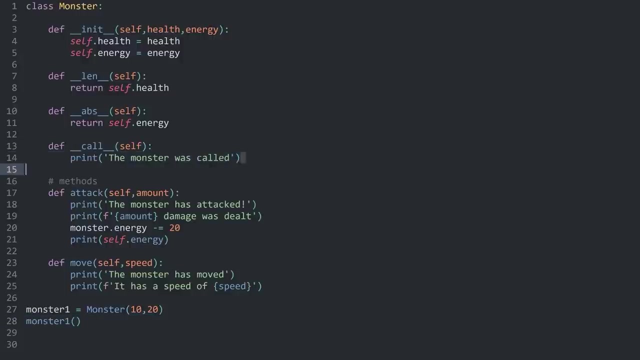 and call print, And now the monster was called. I guess a cleaner way of doing this is to return nothing and just print this string. So now, if I call monster1, we get the monster was called and nothing is being returned. And when you create a function in Python. 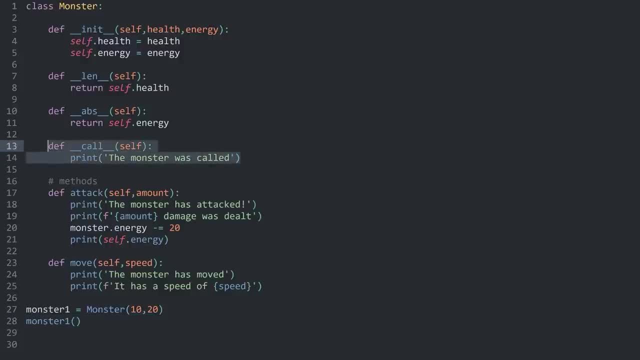 it basically, behind the scenes, creates an object with this dunder method here, And this we can just create ourselves. It really isn't that complicated, And what we can also do is to add and subtract numbers, And this you would, for example, 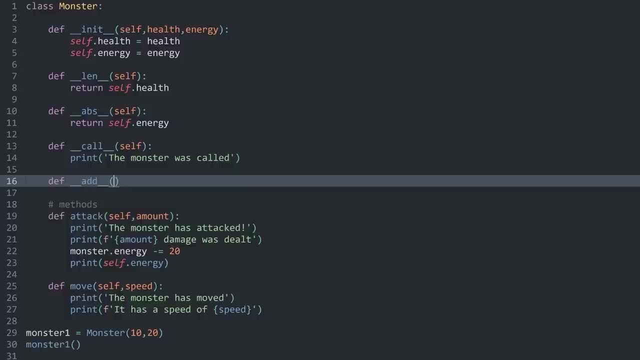 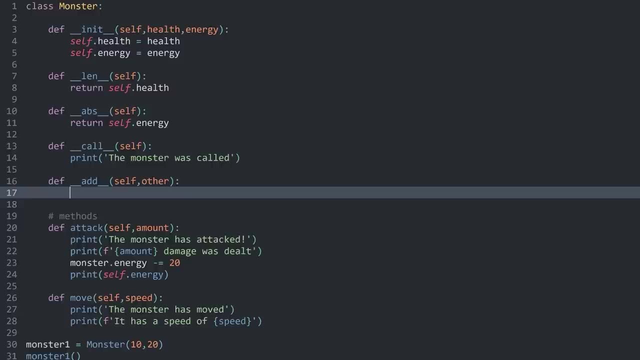 do with dunder add, And in here you need two parameters: First of all self, as always, and then you need some other number, And what you can do in here is return something. Let's say I want to selfhealth, and then plus whatever other number I get. 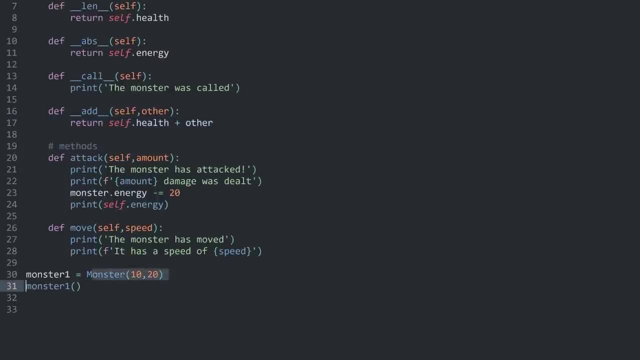 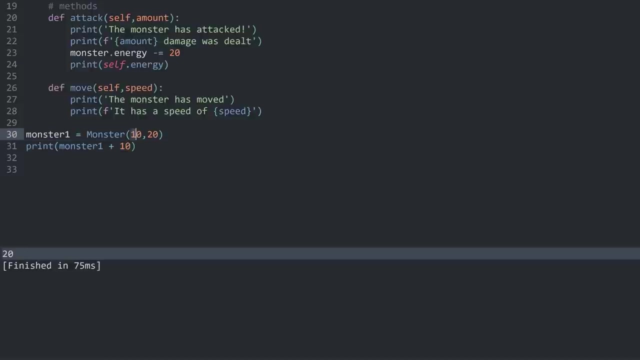 And now that I have that, I can print monster1 plus 10. And if I run it I get 20, which is if I find it. So the health of my monster is 10 and I add 10 towards it. 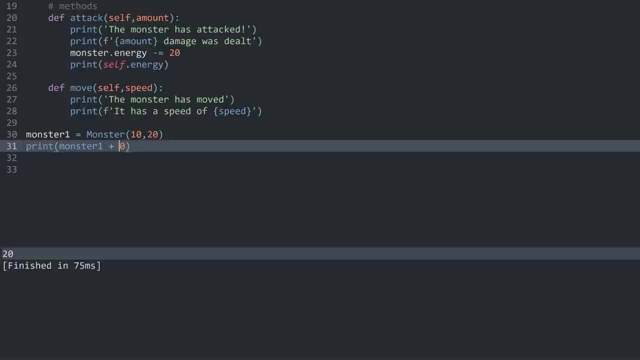 So I get 20.. And I guess, to make this a bit more understandable, let's add 55 in here, And I get 65. Which is 10 plus 55. And well, that is a couple more dunder methods. 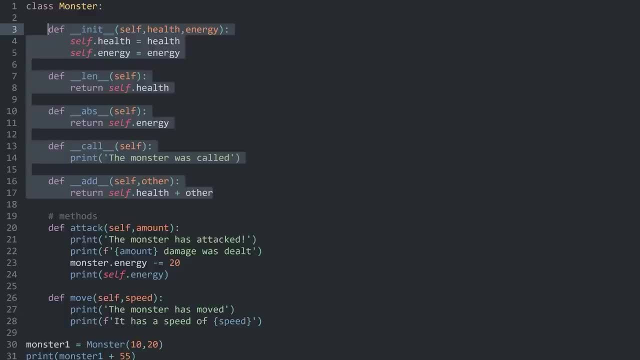 They can be incredibly useful, although most of the time you are only going to use dunder in knit. This is the one you absolutely have to understand, But I guess they don't really get that much more complicated, so it shouldn't be too hard. 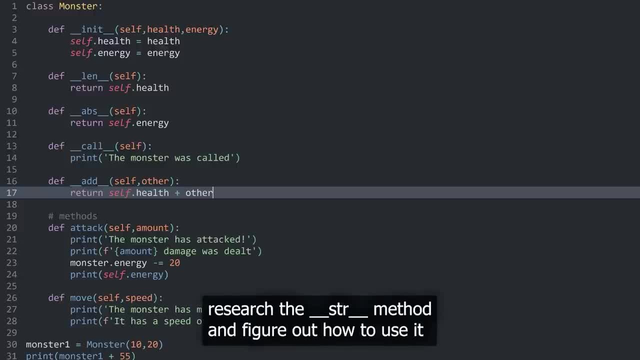 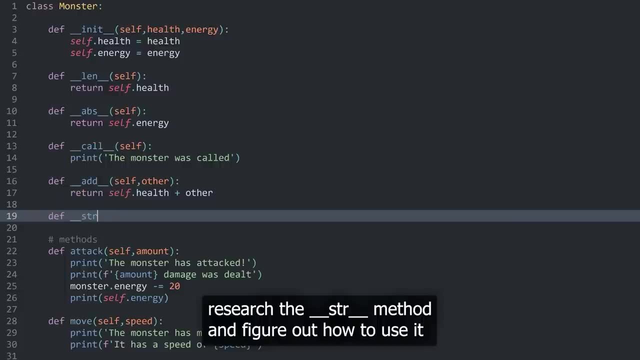 All right, Now for the challenge. for this part, I want you guys to do some research, because there's another dunder method that is called str, And I want you guys to look up online what it does and how to use it in code. 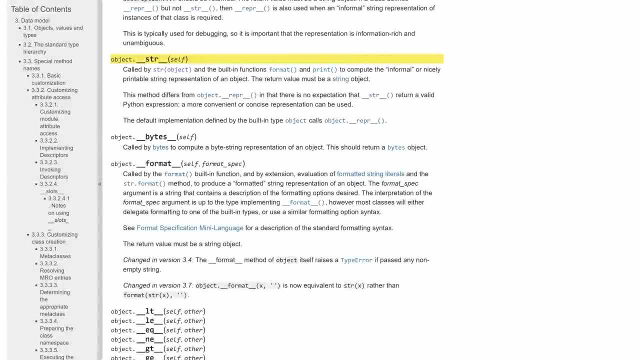 All right, Here we are in the official Python documentation And there you can see dunder string or dunder str And basically what it does. it's called by the str object build in function format and print to compute the informal or nicely printable string presentation. 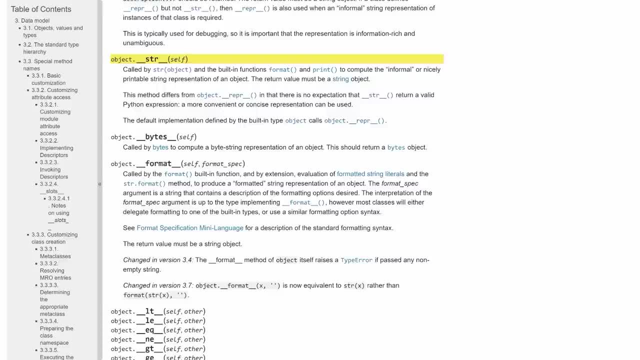 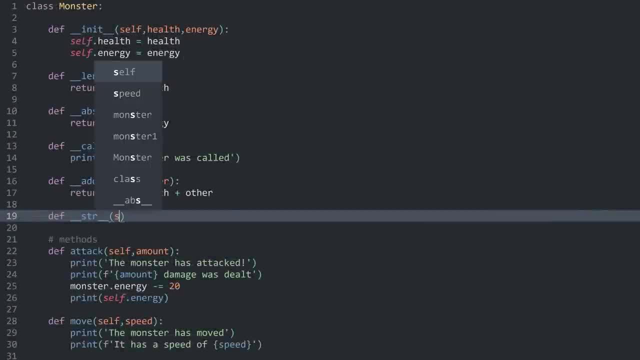 of the object. Basically, what it means is that this object is going to return some text. So let's have a look at it. Here we are back in the code and I only need one parameter, and that is self. And now I have to return. 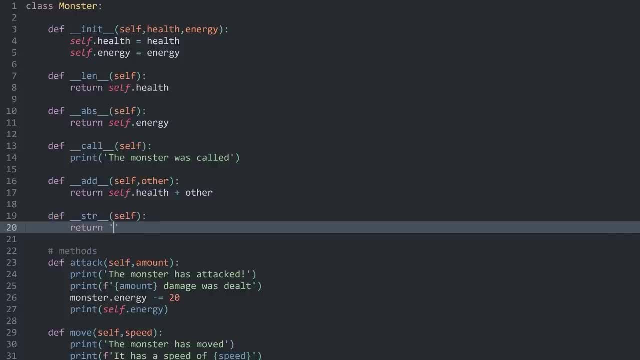 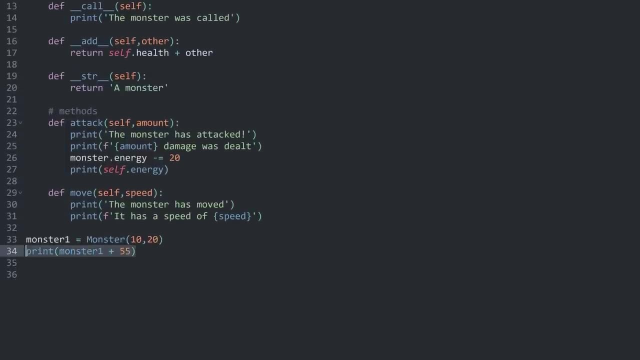 some kind of string And the string I want for this one- let's say a monster- And what I can do with that. let me get rid of this bit. I'm going to print statement and instead I want to print str or monster one. 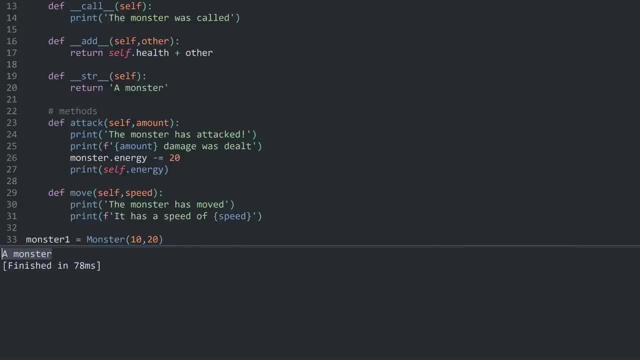 And this is going to return a monster, And we don't even need this str, because print is trying to find a string. So let me duplicate this line and remove the str and just have monster one. If I call this now, I still get a monster. 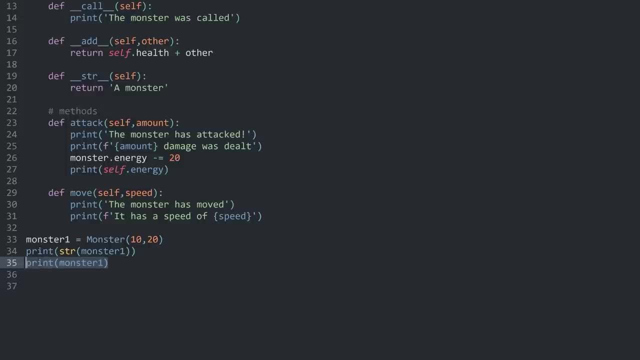 And this can be a really nice way to look at your objects and see what they are doing. Because if we didn't have this dunder method- let me comment it out and run this again- All we get is a monster object, which really isn't that useful. 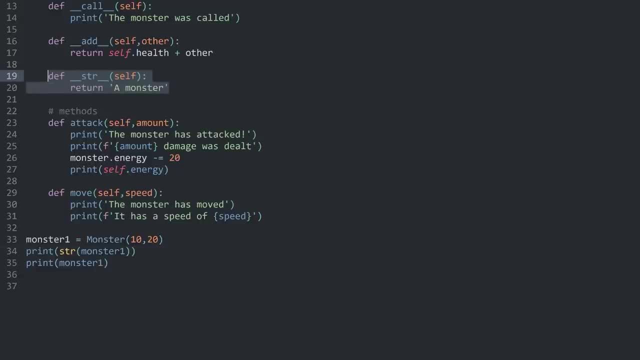 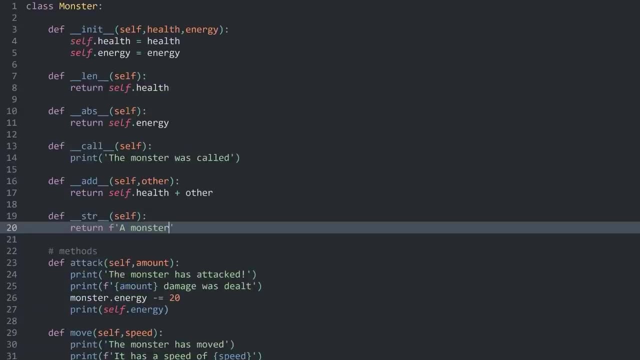 And obviously this str can return a lot more than just a simple string. For example, we could have an f string with health, that says self dot health, and energy, that says self dot energy. And now, if I run this, we get quite a bit of information. 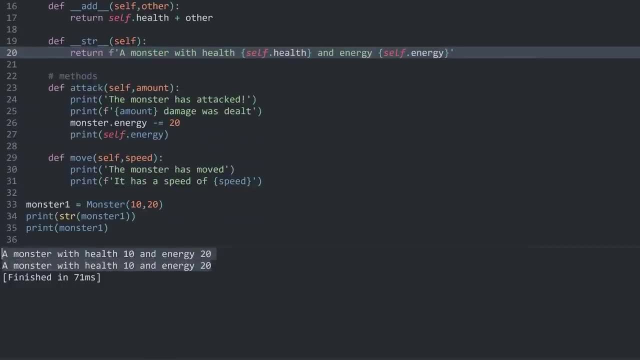 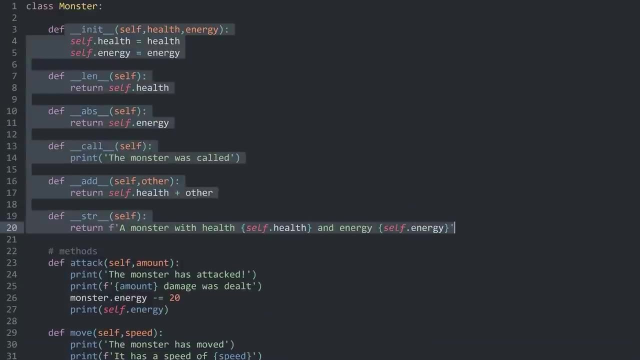 by just passing the monster or the object into the print statement. So this str can be really, really useful. And with that we have covered quite a few dunder methods. If you look online you can find even more, but well, 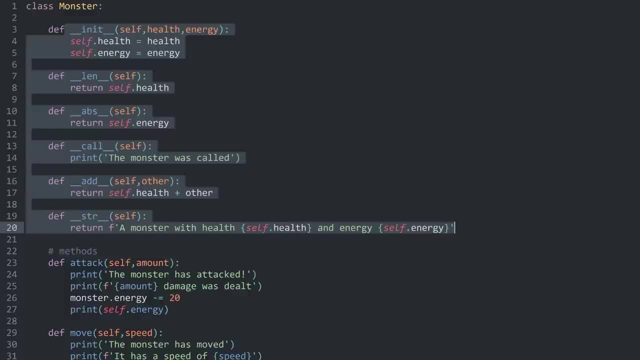 most of the time, you're not going to need them. This is very often a fairly advanced topic, Except dunder init. this is the one you are going to use a lot. But all right with that, we have dunder init methods covered. 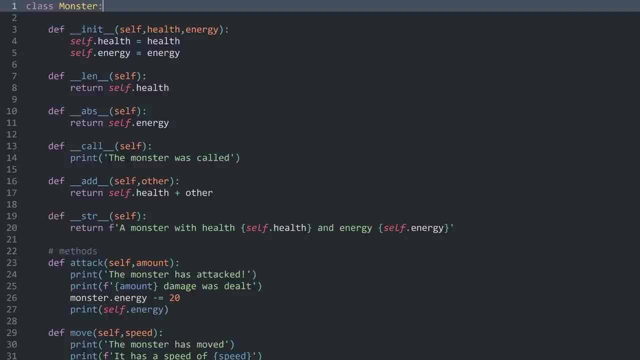 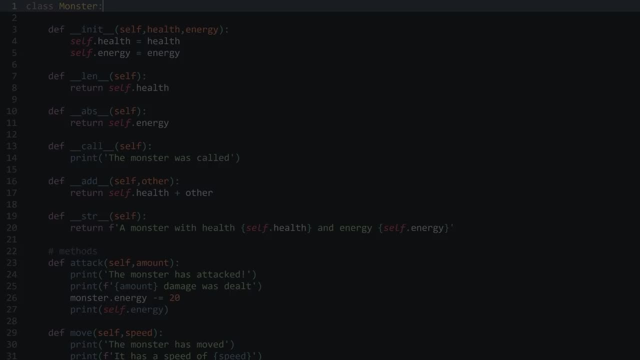 And if you understand all of this so far, you can actually understand Python itself quite a bit more. Let's talk about this one in the next part, And the one thing I think that confuses beginners quite a bit is that every single thing in Python 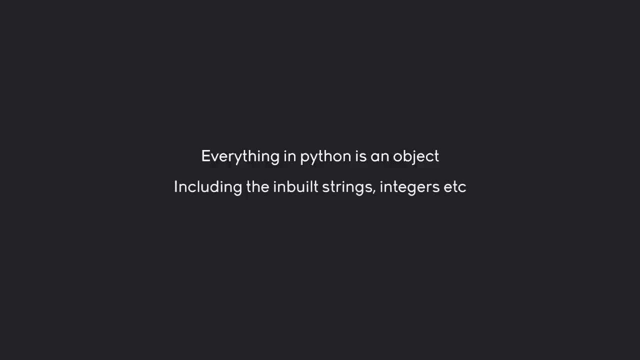 is an object Meaning. every time you see a string or integers, you are going to see an object, Just like the objects that we have created, so our monster. And this even includes functions, which are just objects, with the call dunder method. 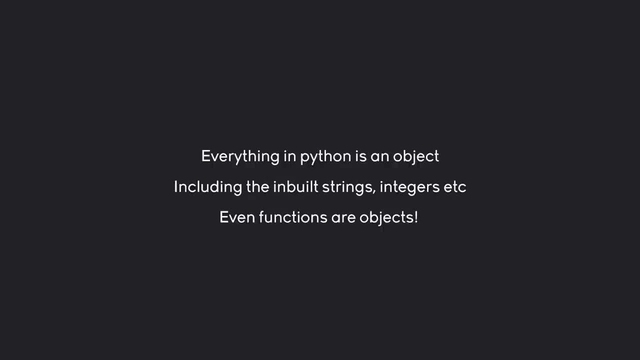 And I'm going to show you some examples in just a second. but most of what I will cover here isn't really important. I just want you guys to understand how it works so you don't get confused later on. And there's another thing. 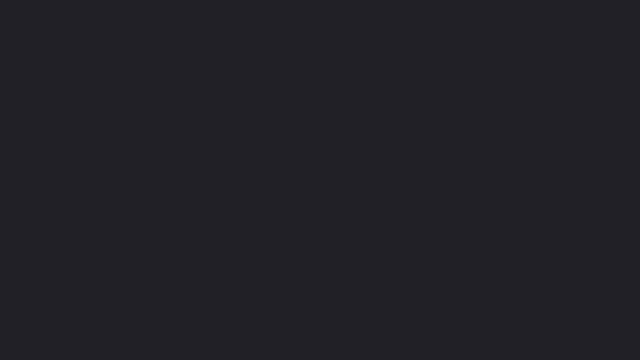 that, I believe, is very often confusing, And that is the difference between a function and a method, And the reason why this is confusing is both just execute a block of code, So in terms of functionality, they basically do the same thing. However, 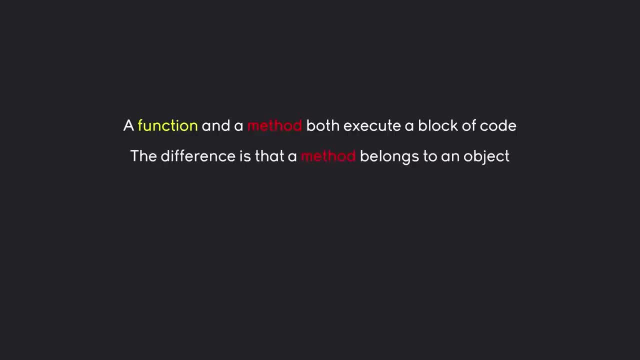 the difference is that a method always belongs to an object. It doesn't matter if the object was created by us or by Python, And a good example here would be using a string. So if we have a function, this would be len, for example, 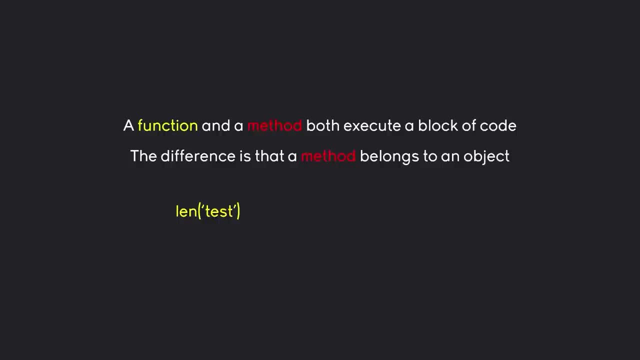 And we can pass a string into it. This will return for, And a method would be something with dot And then upper, for example, for a string returns uppercase letters for this string, And that really is the entire difference. That's the main thing. 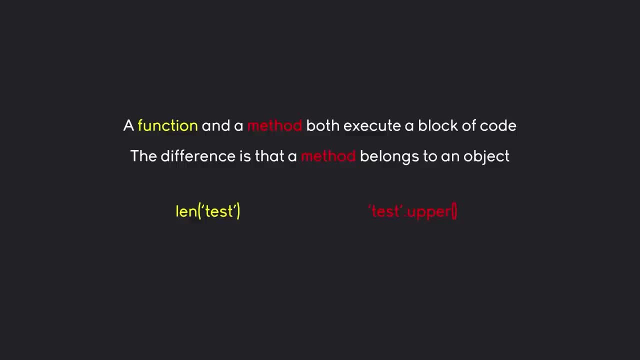 you have to understand, And it doesn't matter if we create the method ourselves or the function ourselves or if it's created by Python, And the reason why these are different, for example, is that the len method could work for lots of other things as well. 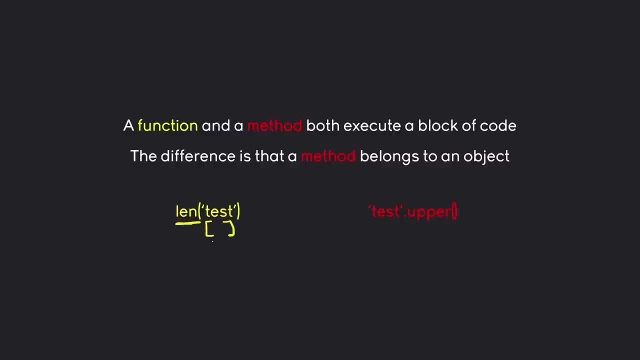 For example, you could pass in a list in here. You could pass in a dictionary or a tuple- It would still work with different data types, whereas upper only works for strings. You couldn't add a list with upper, That one would not work. 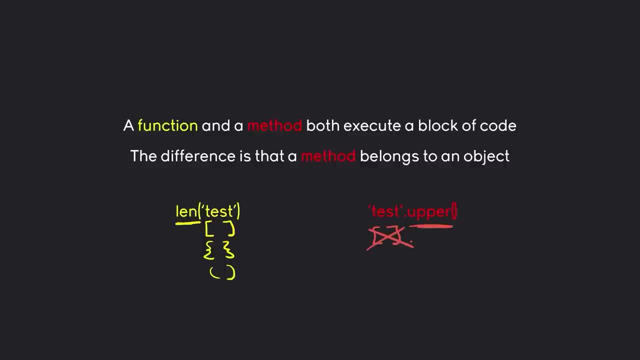 So it makes sense in this case that upper only exists as a method for strings, whereas len should be a function. so you can pass in different kinds of objects in here and they would all work. You could, perfectly fine, create some kind of len method for a test. 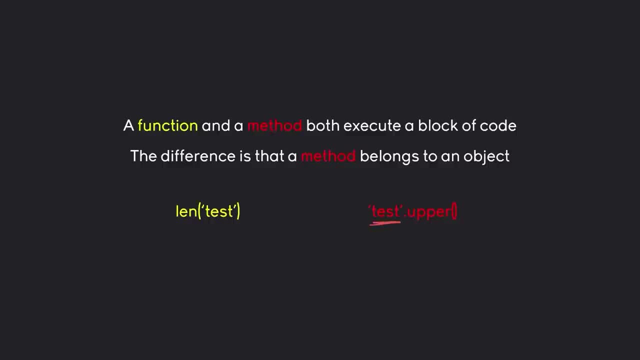 and it would work just fine, Although then you would also have to create a len method for lists, for dictionaries, for tuples, for all of that stuff, and it would be quite labor intensive. So all we're doing here is to keep things more efficient. 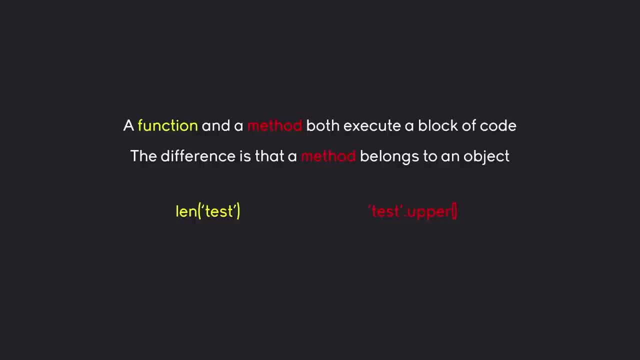 But alright, let's have a look at some code and let's have a small deep dive into Python. Here I have a completely empty sheet of code, and what I want to create for now is create a test variable, and this one should have a string. 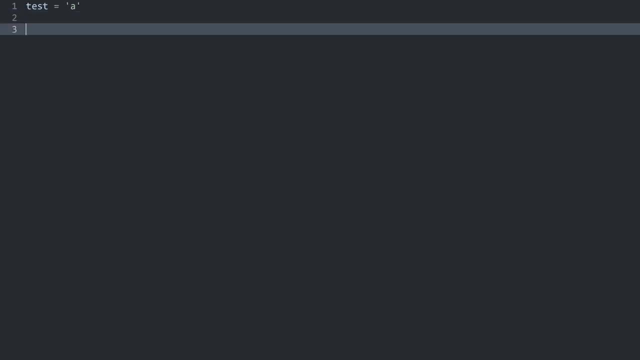 Let's call it a, doesn't really matter what it is And what I can do now. I can call my print dir and pass in my test in here, And if I run this now I am getting a bunch of dunder methods. 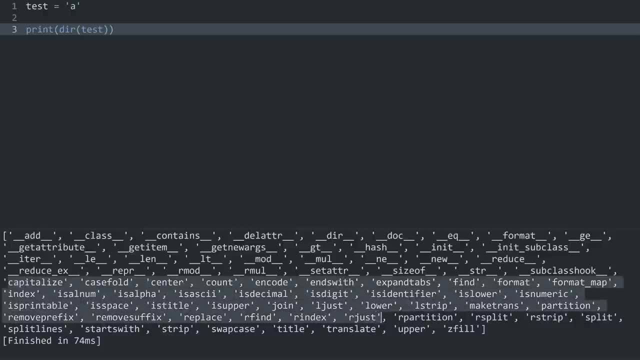 and after they are over. starting from here, I get a couple of methods and attributes. Now, the dir method doesn't separate between methods and attributes, So we just get one big list. But well, basically what we get here is an object. 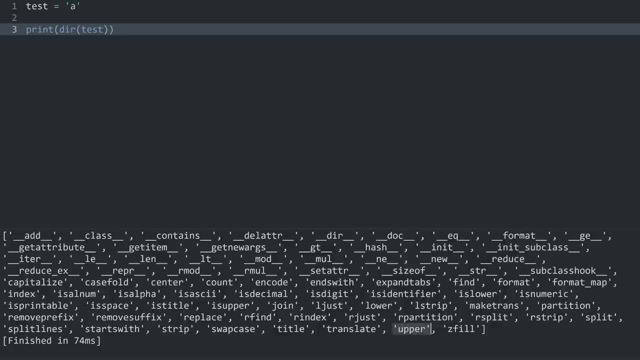 And anything in here you could just call, like upper or title or string or type. All of these are very simple methods And along with that we have the len dunder method, and this is what's being called when we are passing this string into the len function. 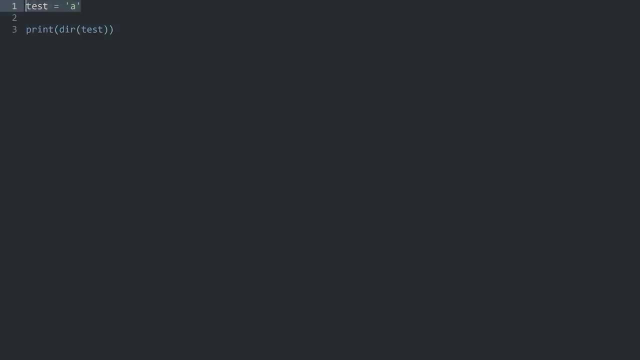 And besides that, what you can also do, let me get rid of this test and instead create define test. and then here I let me just add pass. So this is a function with the name test and I'm still printing dir test. 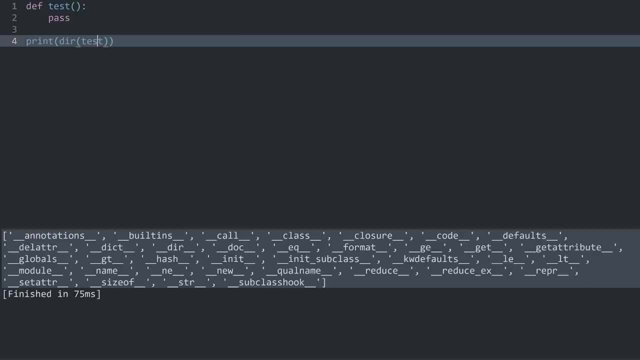 So if I run this, I am getting another object, and this object is special because it has a call dunder method, Meaning when we're adding brackets afterwards, it is being executed. And that's basically what a function is in Python. It's just. 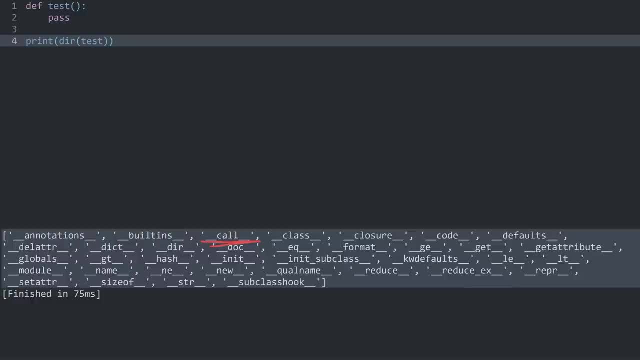 an object with the dunder call method. It really isn't much more than that, Although we do have a couple extra things that make this a bit more special. but that's the main idea And if you really wanted to, you could even. 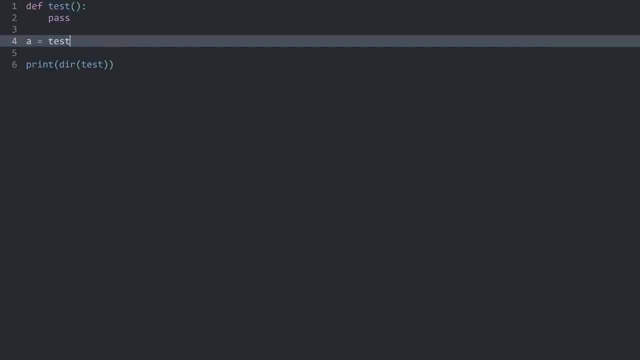 store this function inside of a variable, And this works because the function is an object, So this is just going to be an object Meaning. if I now print a, we are getting the same outcome, Although what we can even do now. let's call it. 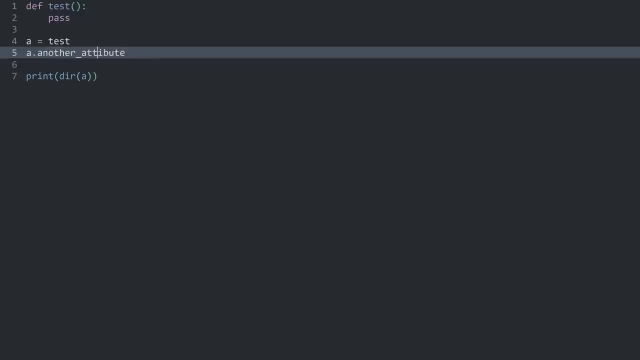 another attribute. That is not how you spell that, And this could just be 10.. And now, if I run this, our function has another attribute. And again, this is working because functions are just objects, Although in practice you wouldn't really do. 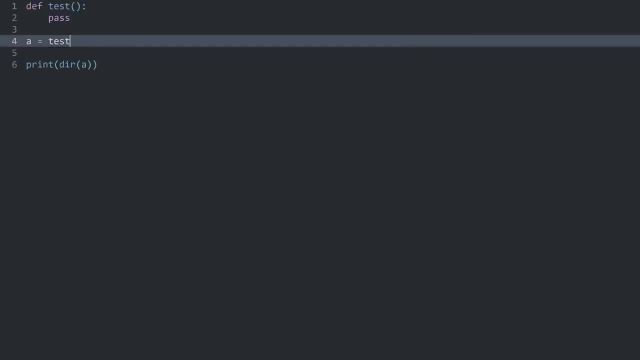 this. there's no reason for it. But what is much more common is that you are passing functions or adders. Let's say, for example, a simple add function And this one takes a and b and is going to return a plus b. 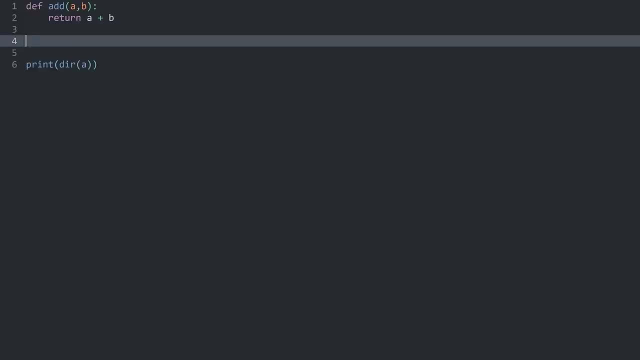 Obviously, this still isn't particularly useful, but I just want to illustrate what it does. And now I can create a class and let's call it test, And in here I'm going to add a function. And now, inside of this dunder, init. 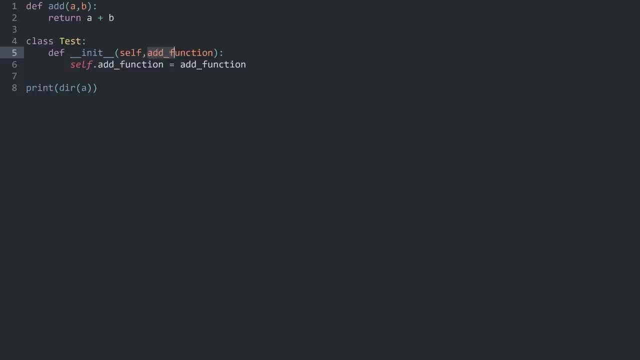 add function. I can set an attribute- self dot- add function- and this should be the argument we get from the parameter add function. And now, when I create this test, I can use a named argument, so it's a bit easier to see what's happening. And in 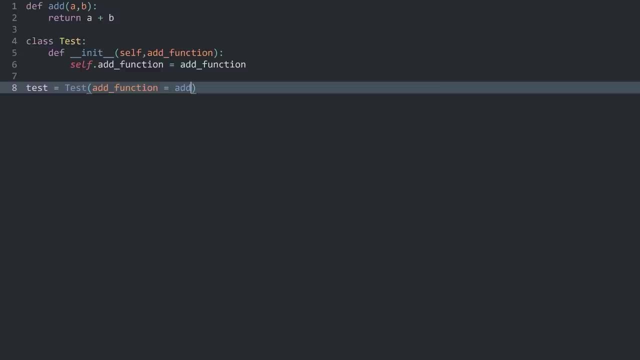 here it is really important that you don't add brackets, because we don't want to call this function, we want to get the function itself, So the object of the function, not what's being returned. Let's say one and two And this is not. 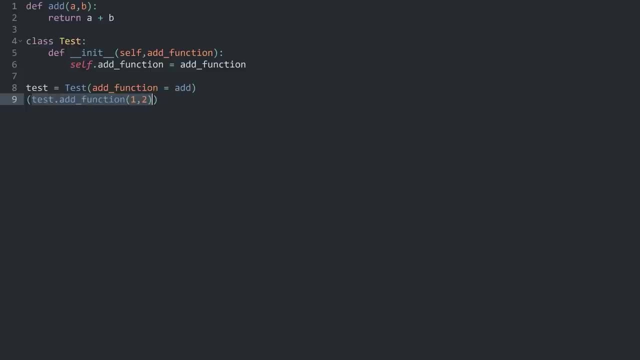 doing anything, because we're not printing anything, we're just returning something. So if I put all of this into a print statement now, we are getting three And I hope all of this is making sense. This is working just fine. And then, inside of 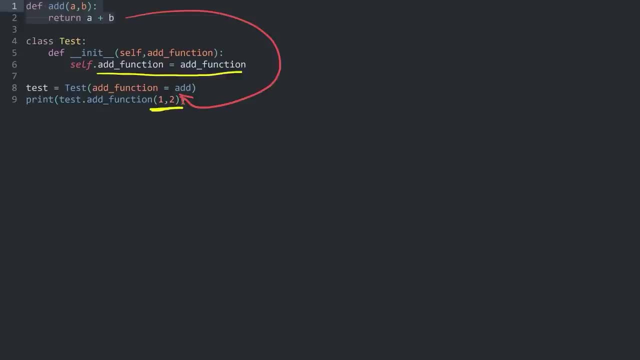 the class. we can store it inside of an attribute and then call it from outside of the function. This is working just fine. there's no limitations on this, And this is something you really want to practice, because passing around all of these parameters is not going. 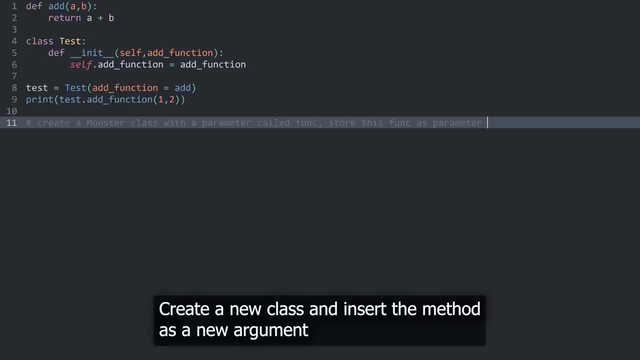 to help you in any way. So let's see what we can do with this function. So we have a function called func and this should work kind of similar to the function we have in the class. So let's see what we can do with. 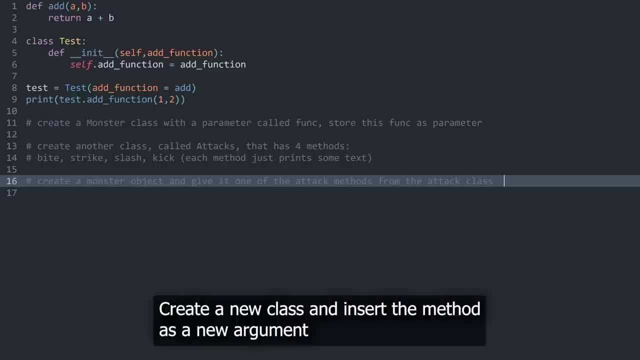 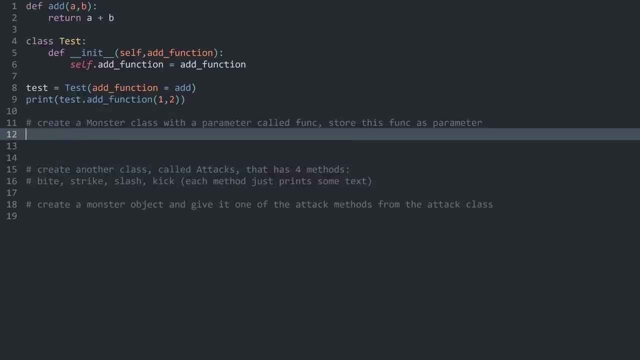 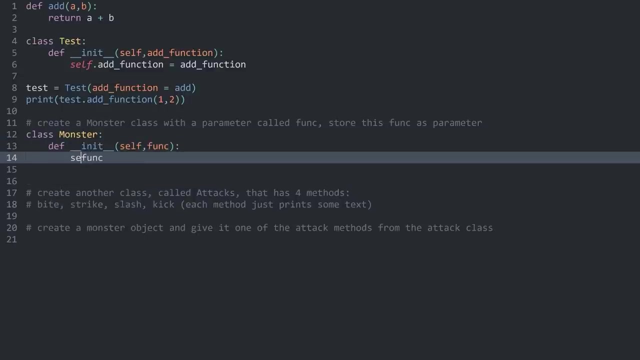 this function. So let's see what we can do with this function. So this function is going to work- kind of similar compared to what you have seen here, But well, it's going to be slightly different. So I'm going to turn into an. 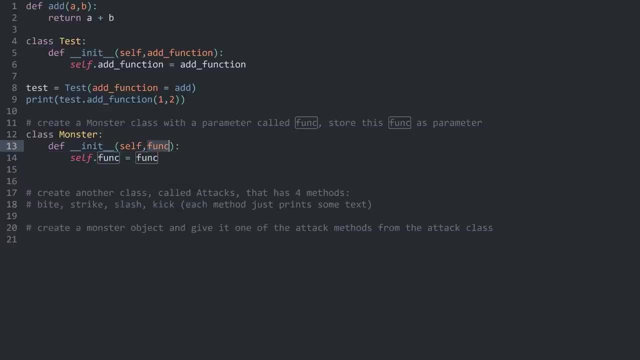 attribute so selffunc and I want to capture the parameter or the argument we get here in there. And this is covering all of this. Next up, we want to print byte, And since we need four attack methods, let me copy this a few more times. 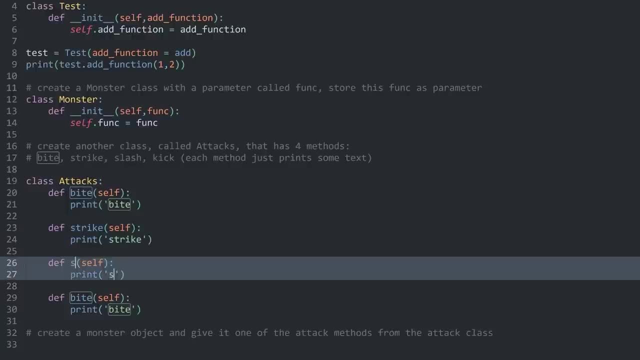 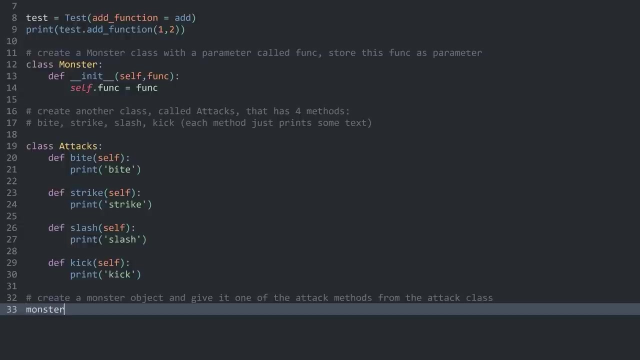 And now, besides byte, I also want strike, then I want slash, and I want to create an object of my monster, So monster in lower case. and then here I want to have my monster. And now we have to do a couple of different ways, Although 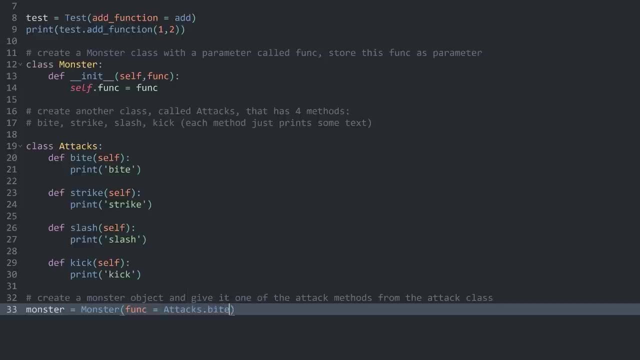 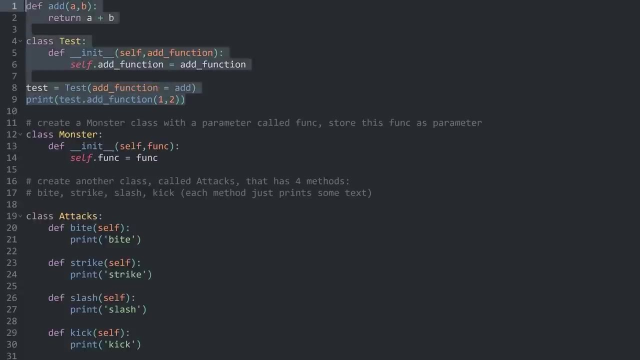 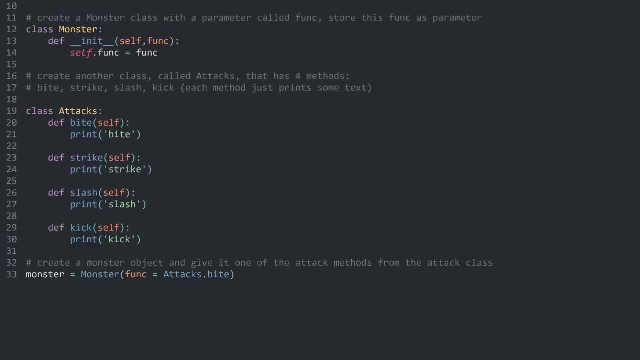 there's one way that is definitely wrong And it's very tempting to go this way. You could write something like attacks and then dot byte, And we are getting that attack. dot byte is missing one required position argument, and that is self And this: 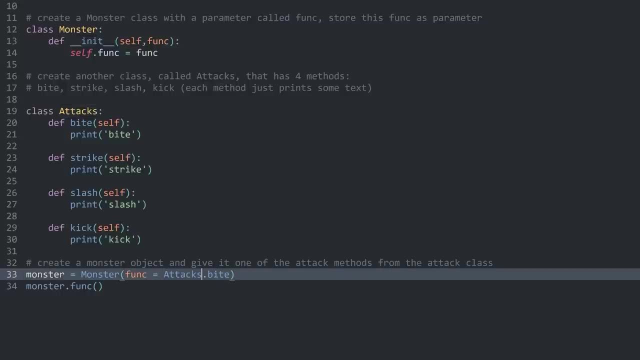 is a reasonably common error. The reason is that this here is a very complex function And basically what is happening here? think of this in terms of return statements. When we are calling this attacks, it's returning an object, And then we call. 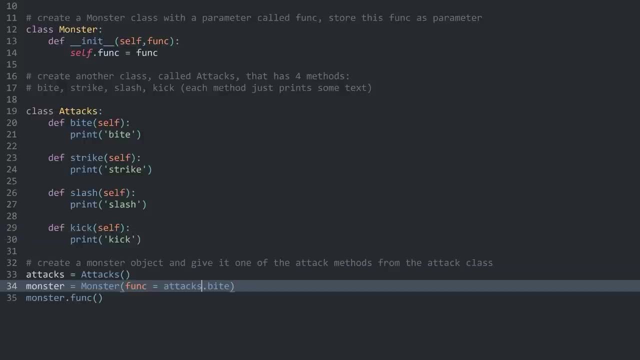 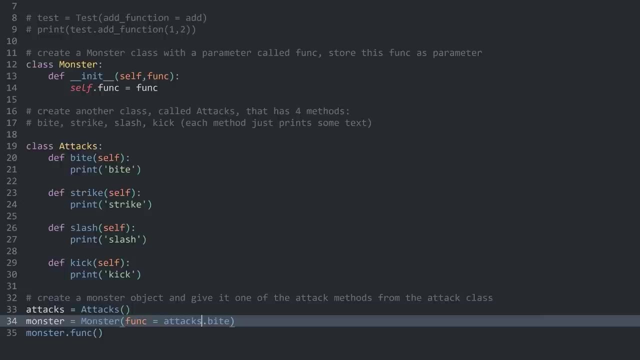 attacks dot byte and we will get the same result, And this is something we are going to explore quite a bit more: That you pass different code, Because a key part of object oriented programming is that you work with different objects and make them interact with each. 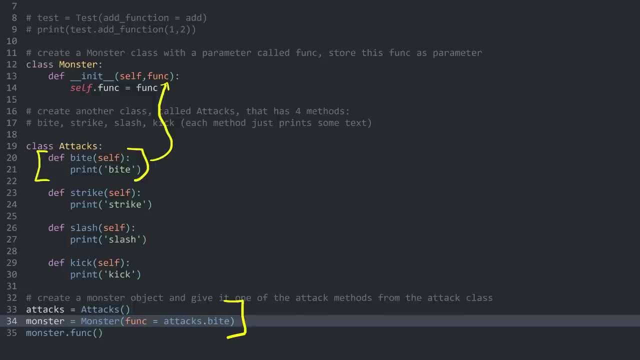 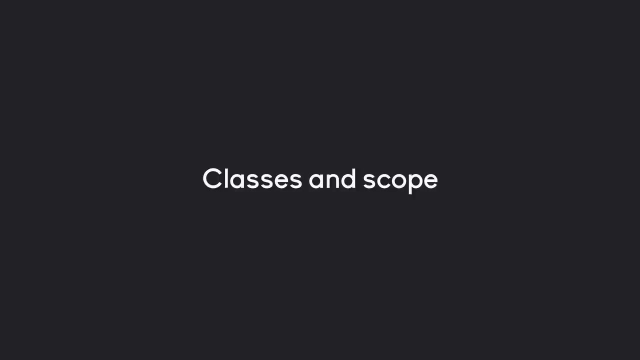 other And this example here. so this part down here is one example to make it easier for you to work with objects and classes. Let's talk about that in the next section. Alright, so let's talk about classes and scope, And 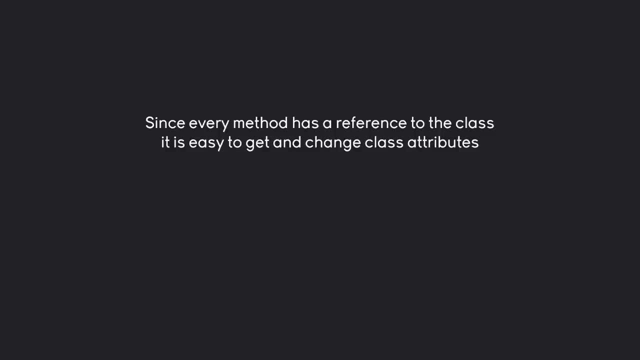 this is what we are going to talk about in this video, So let's start with class attributes, And because of that, methods are much easier to work with than normal from outside of the object itself and even from the local scope of a function. 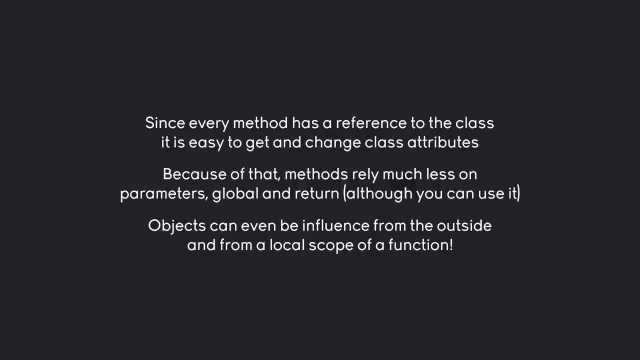 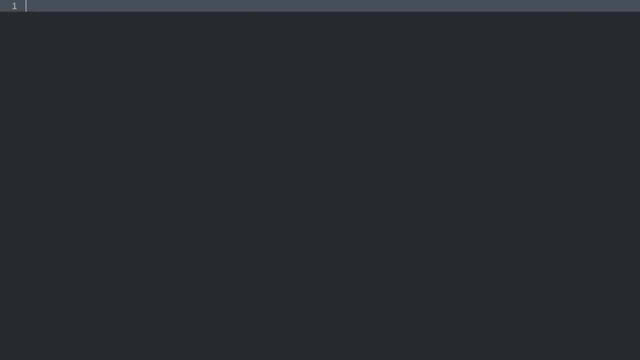 Basically objects, you can change wherever you want. There is no limitation on the scope for the function. let me add a comment: scope problem. And let's say I have a game and I have some kind of health that right now is 10.. 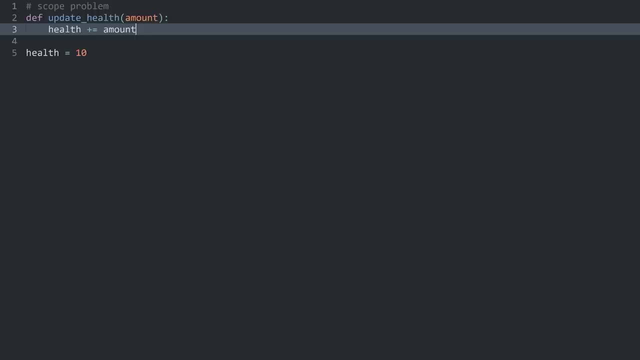 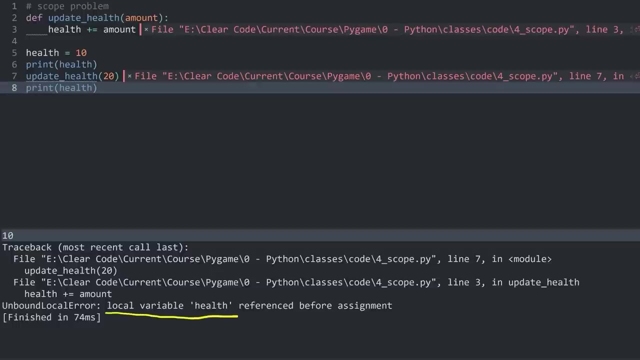 And for this health, I want to print health, update my health with 20, and print my health again. And if I were to run this, what do you think is going to happen? Just think about it And what you'll see. 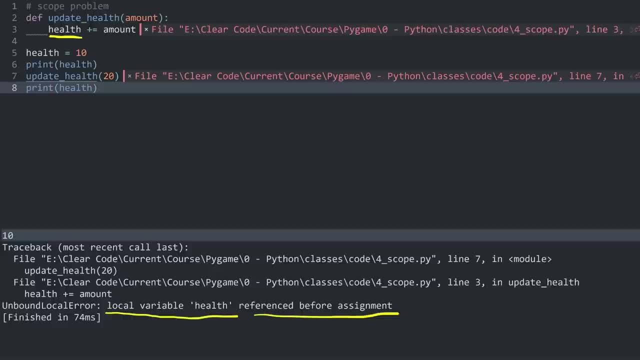 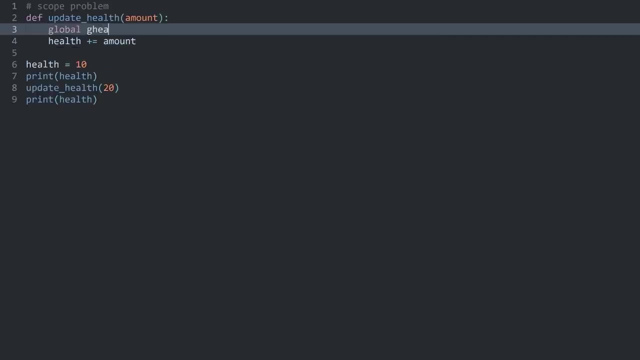 here is that this health to Python is a local variable. Let me remove the error messages. They are getting a bit annoying. That's easier to work with If I want to find some amount. Python cannot find any starting amount for this health. 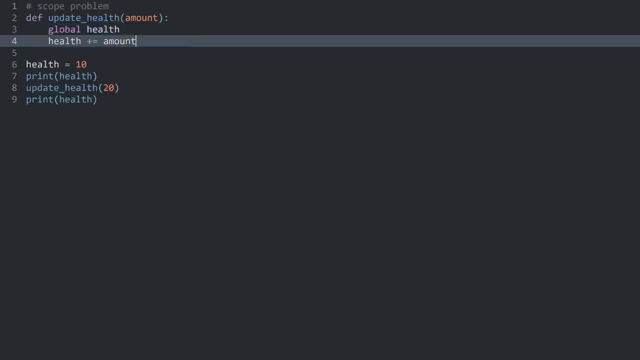 As a consequence, we are getting an error And there are a couple more problems. Let's do the same thing with classes. So let me create a class monster again, And in here I want to create a dunder init method that needs. 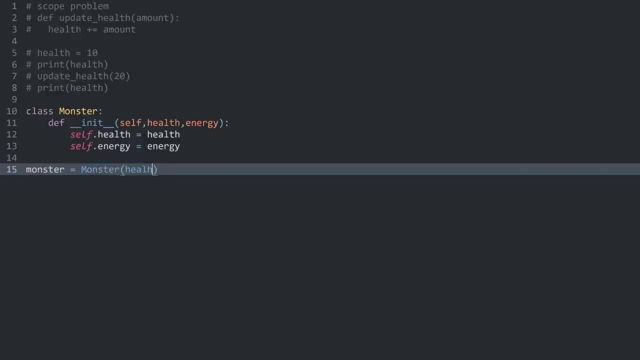 self health and let's give it a health of 100 and energy 50. It doesn't really matter what values you put in here. So now I can print monsterhealth And we are getting 100. Again, we are. 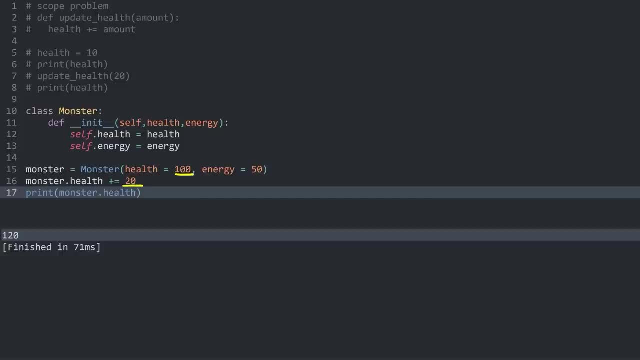 getting 120,, ie the sum of 120.. And what is even more powerful, Let me uncomment this function up here And now. instead of the health, I want to raise this by 20 again. And now, if I. 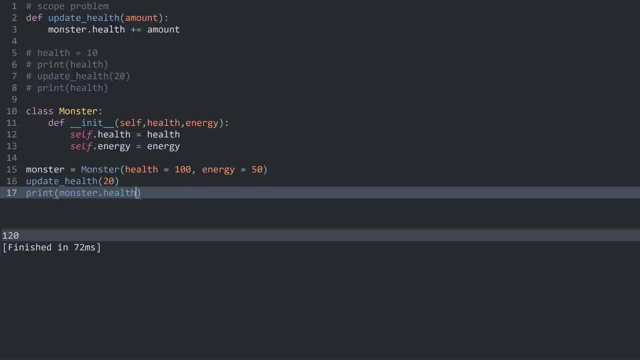 print monsterhealth. after calling this function, I get 120.. Meaning even inside of the local scope of a function. you don't have a variable in the local scope And this monster could be updated anywhere. It could be in the global scope. 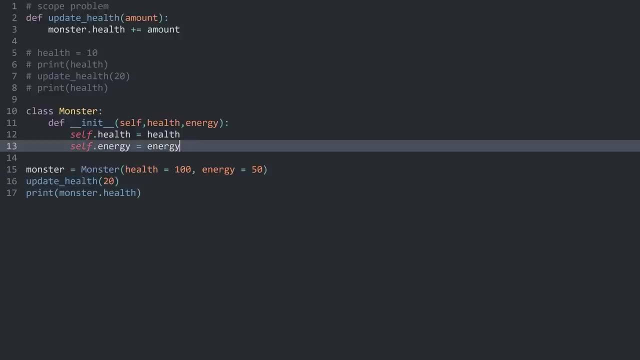 it could be in the scope of another class. You have something like: let's call this one update energy, And then here we need self and let's add an amount in here as well, And what I really want to do is just: 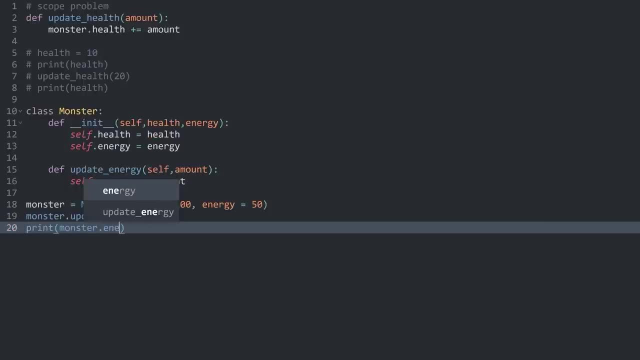 run monsterupdate energy, pass in anything I want in here and then print monsterenergy and we are getting 70.. And again here. this is a super easy to work with, Although, if you wanted to, you could use a return. 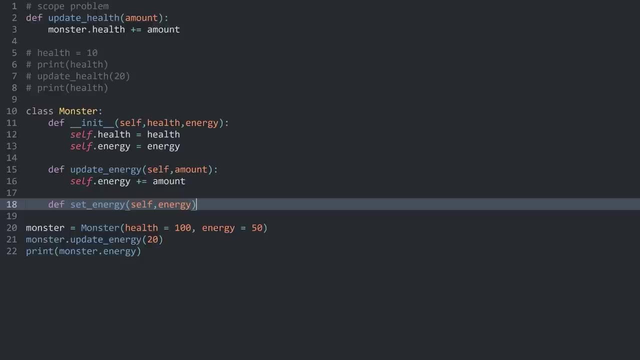 statement as well. For example, if I wanted to set energy- and in here I want self, this new energy. And now in my init method, instead of setting energy straight as the attribute, I want to call selfset energy and pass. 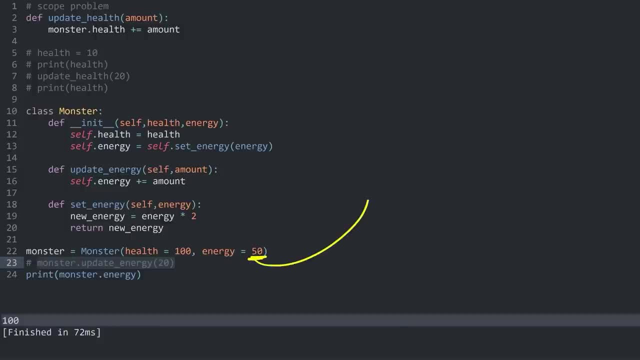 in the energy, And now I have this energy here. From that energy we are passing it inside of another method, inside of the monster class, And this method is down here. We are going to use this method in the next video. I. 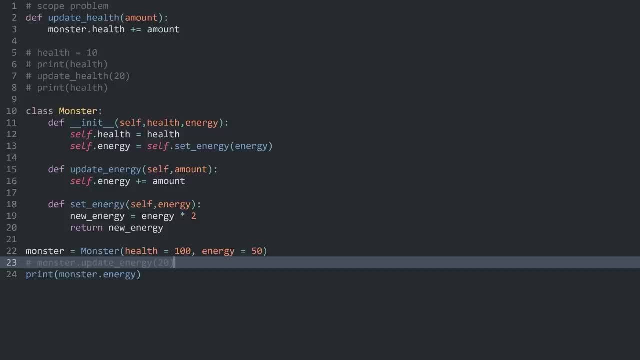 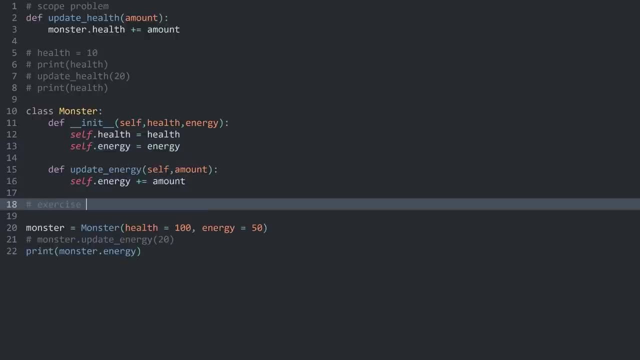 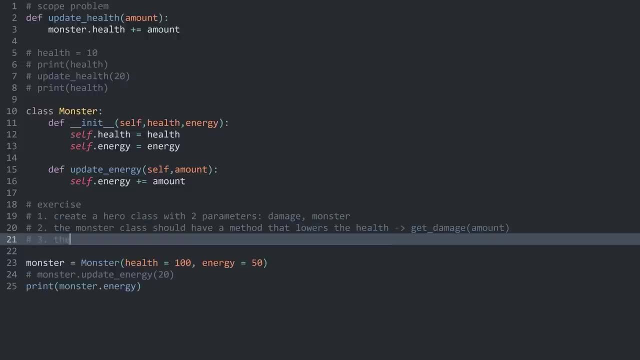 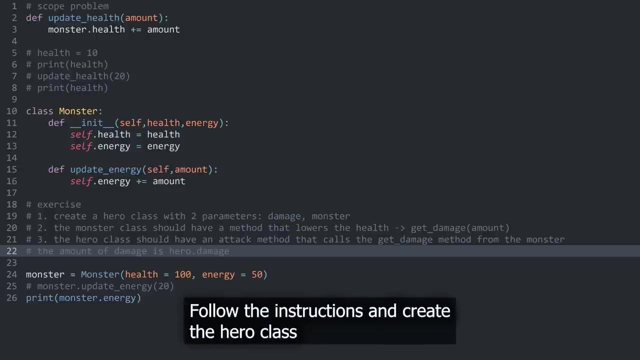 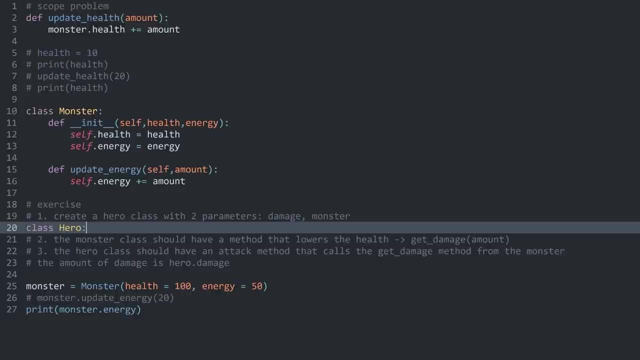 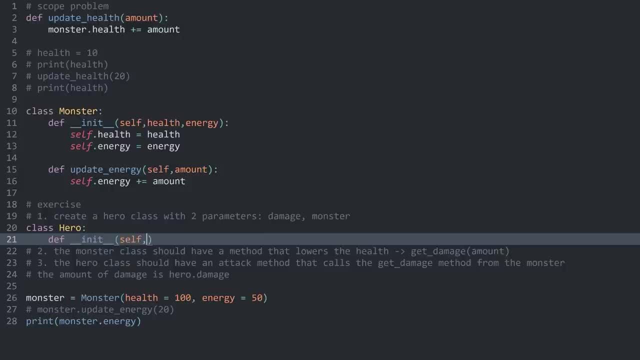 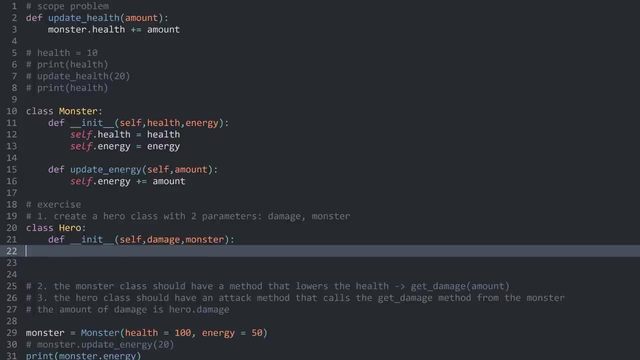 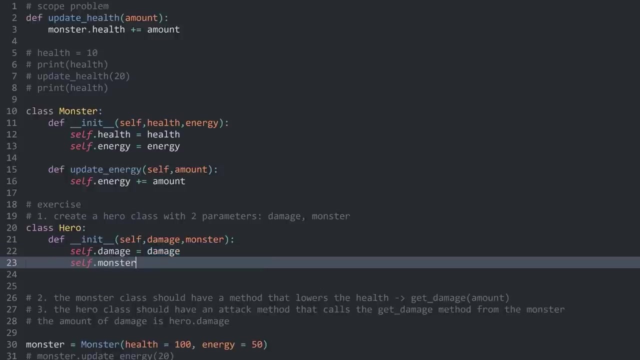 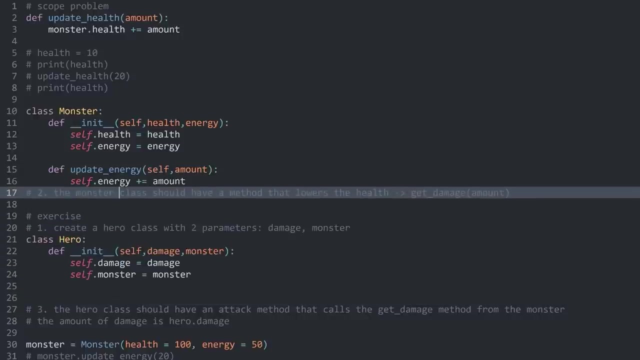 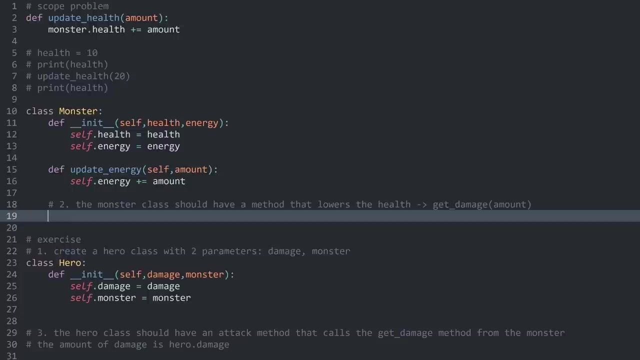 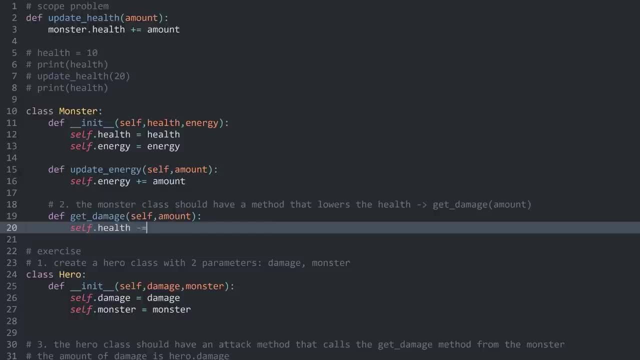 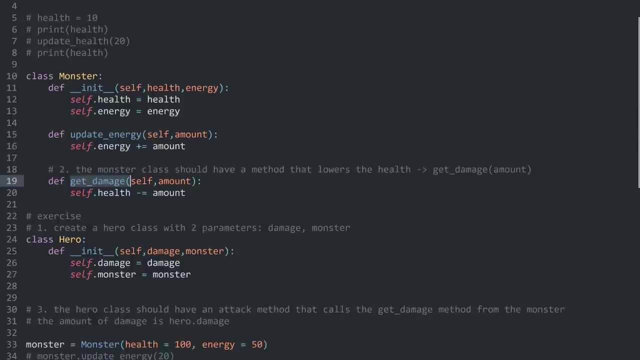 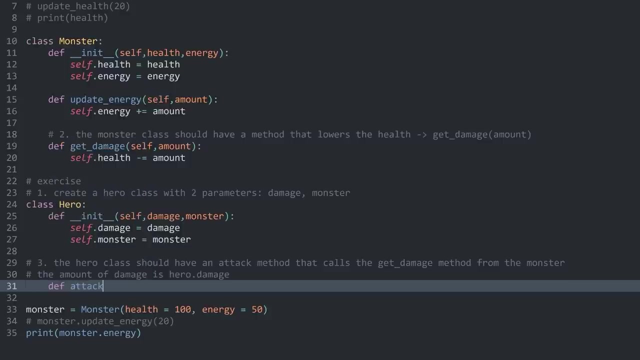 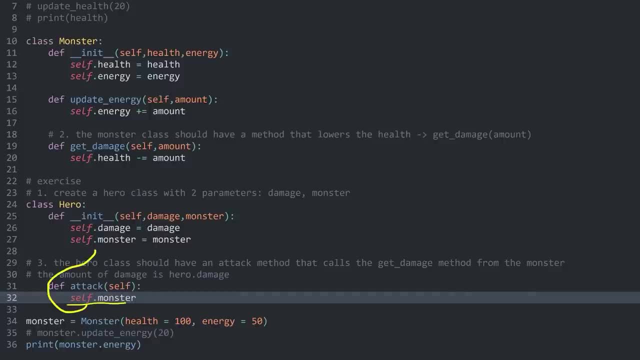 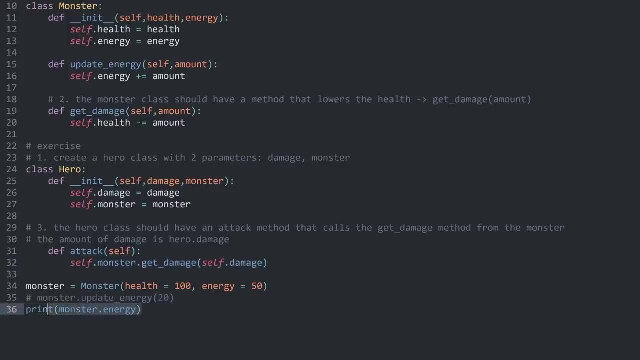 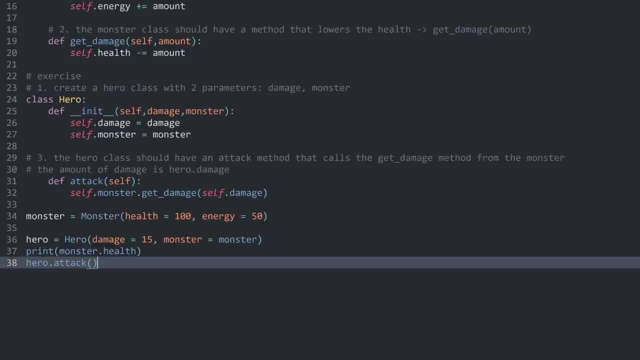 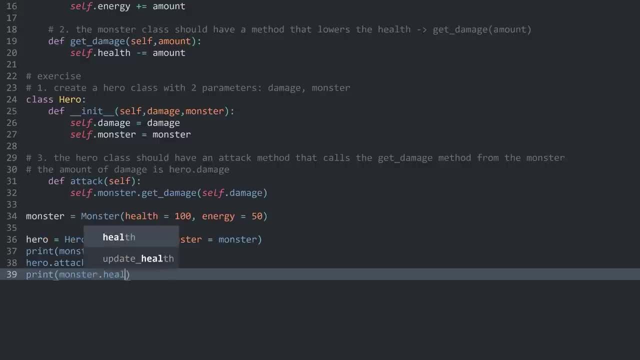 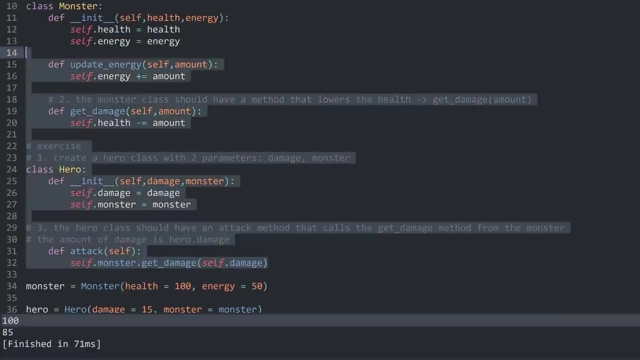 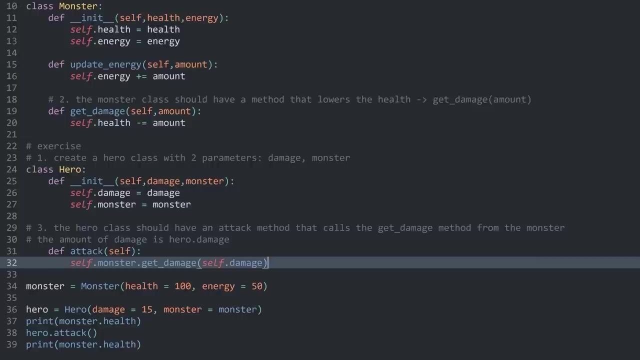 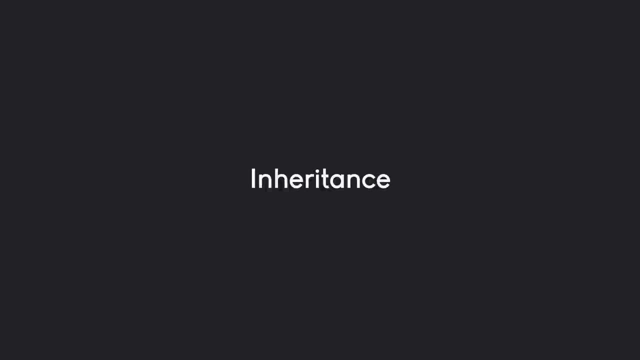 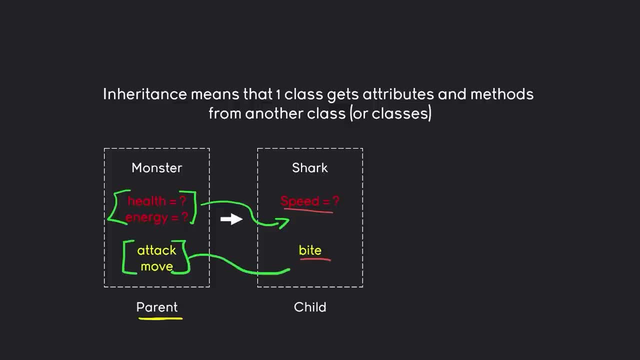 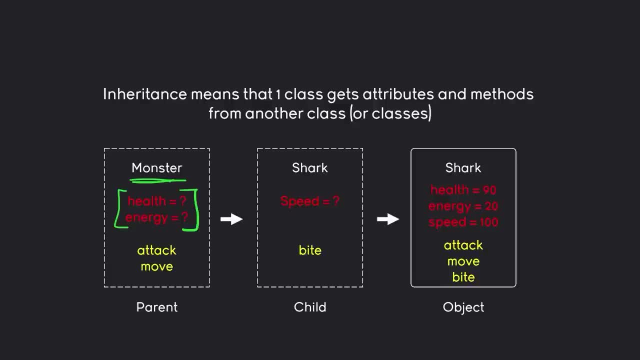 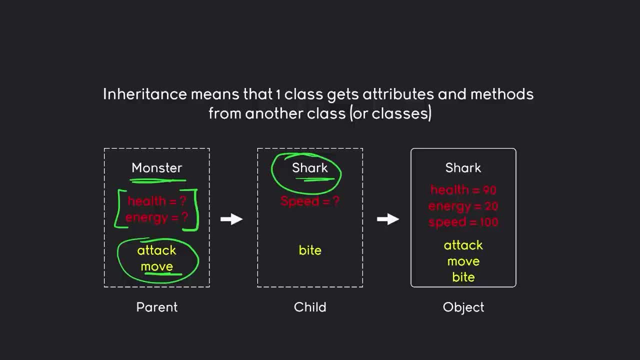 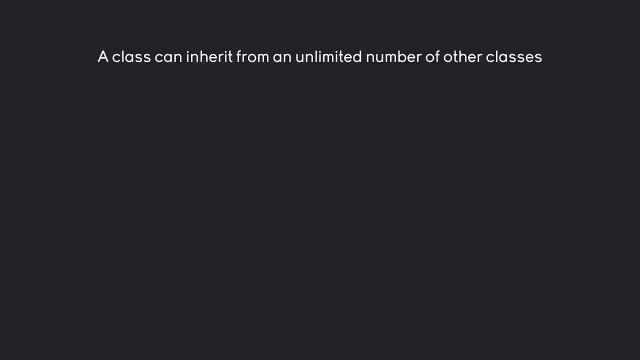 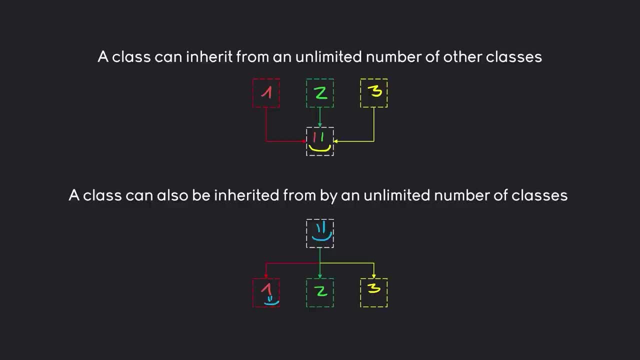 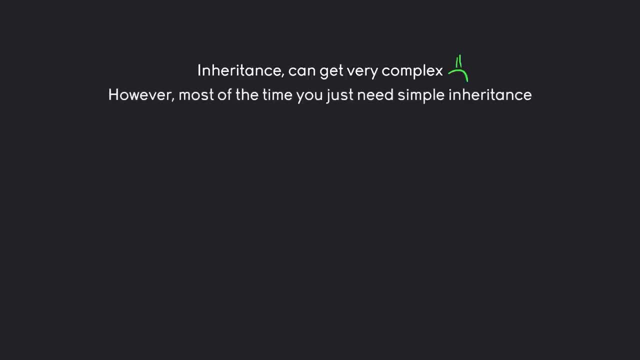 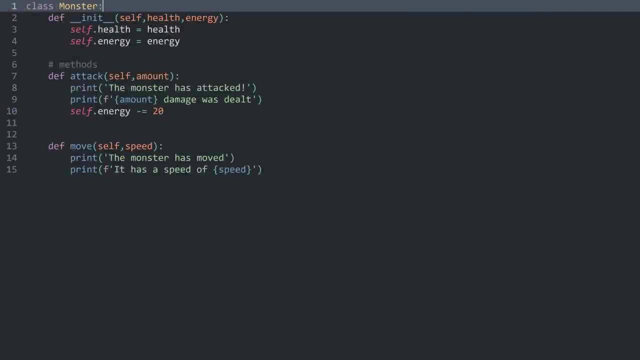 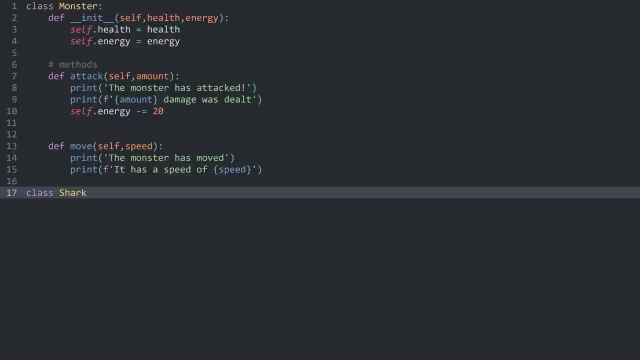 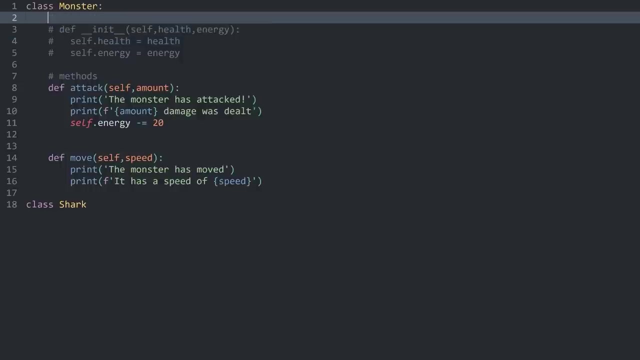 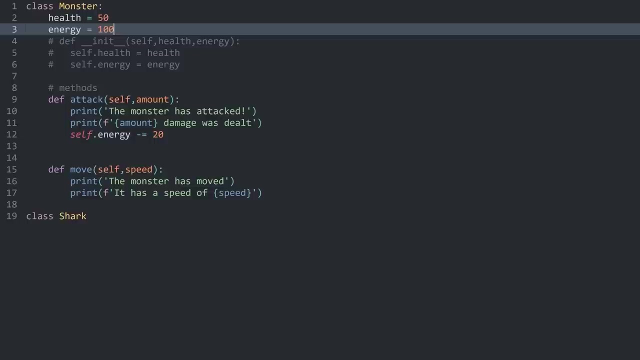 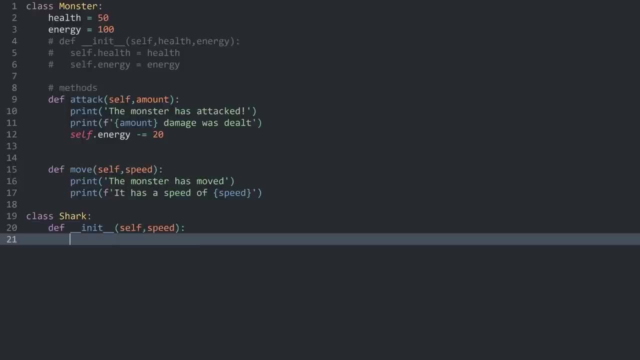 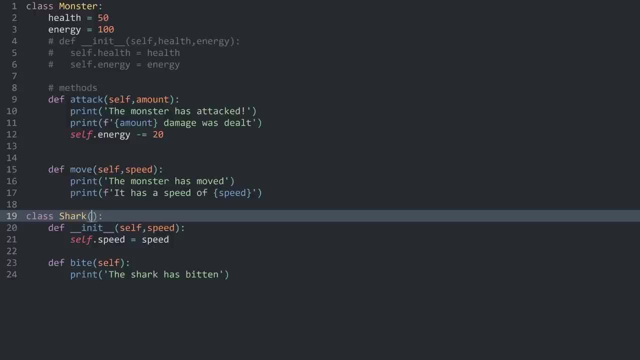 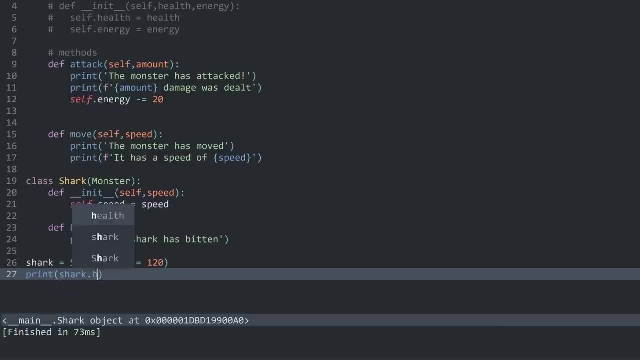 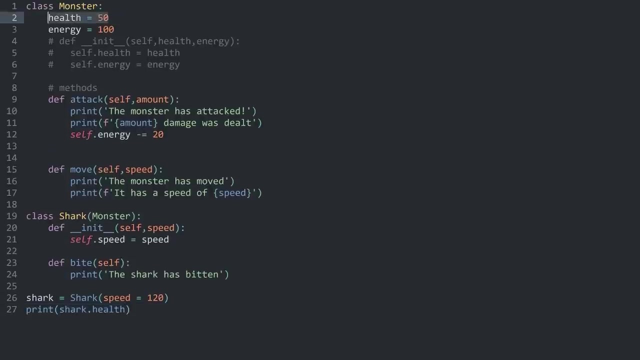 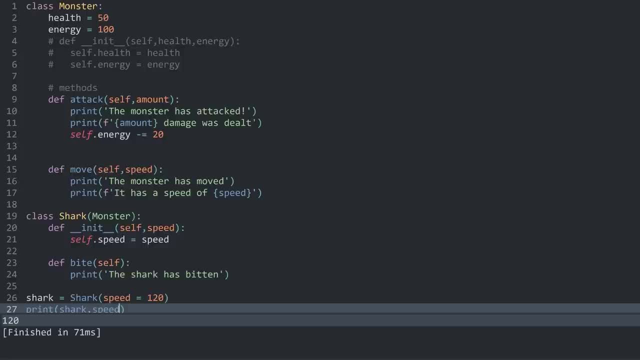 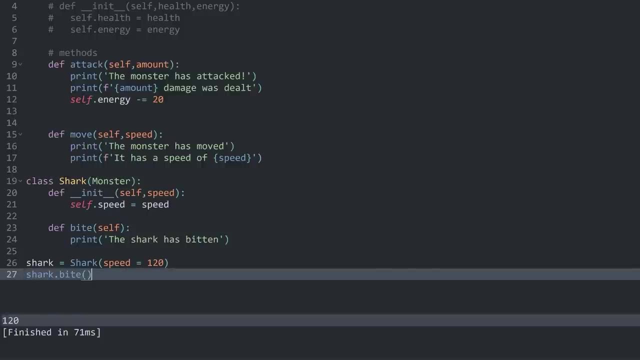 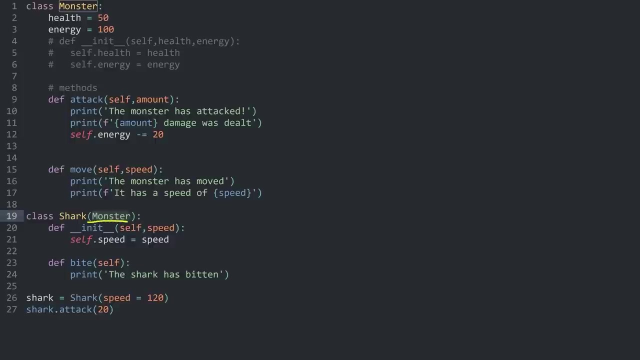 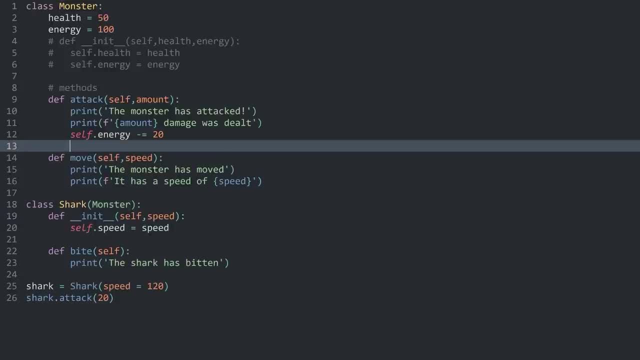 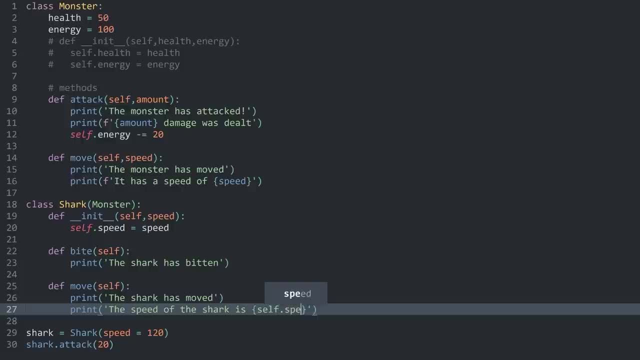 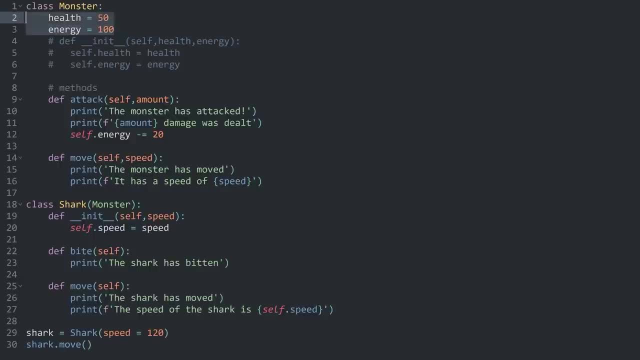 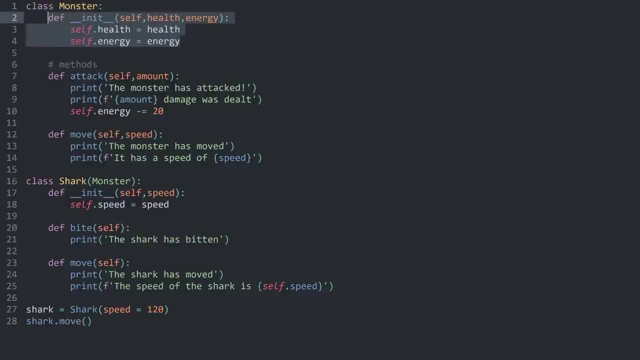 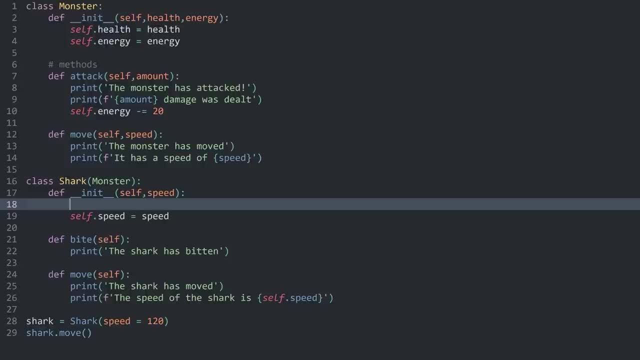 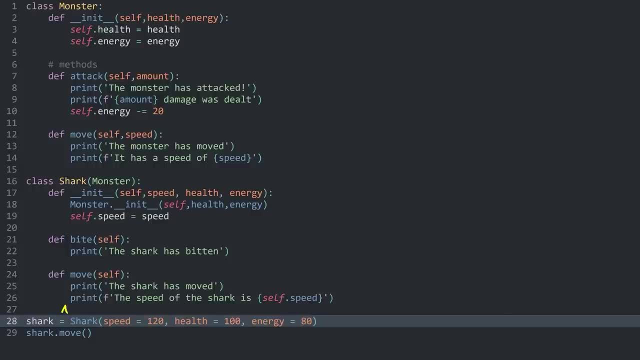 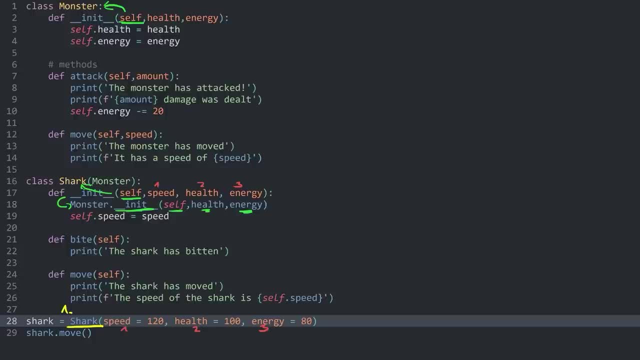 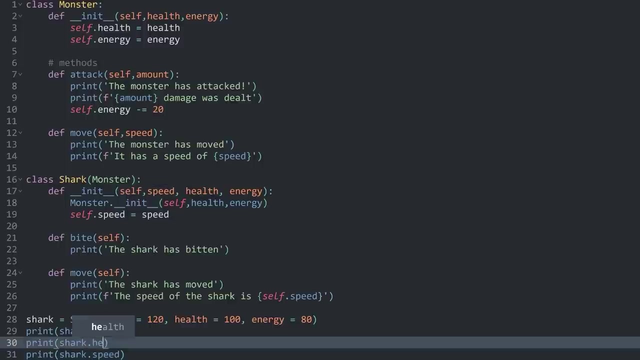 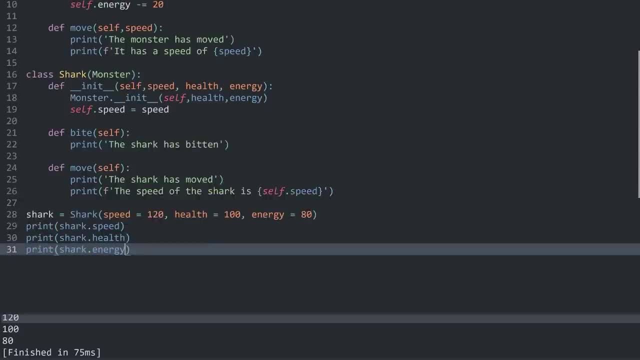 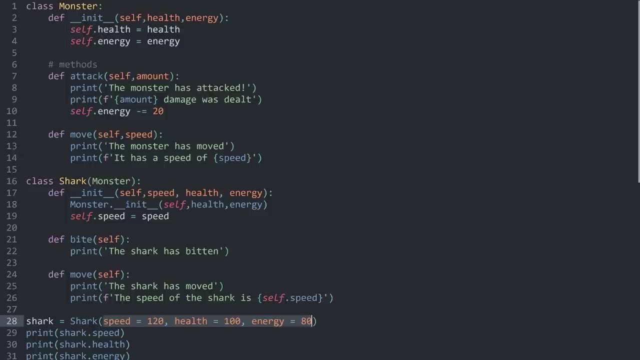 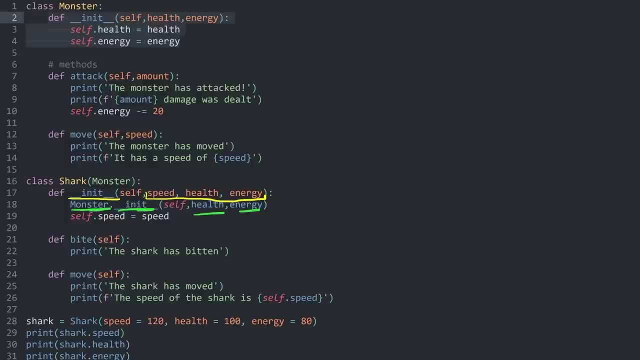 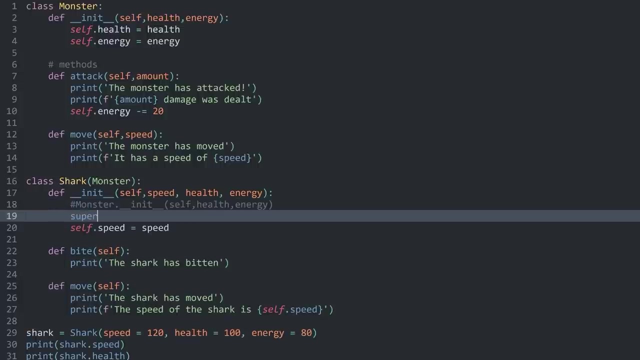 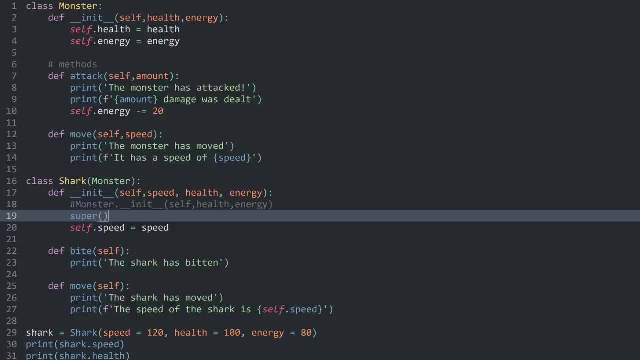 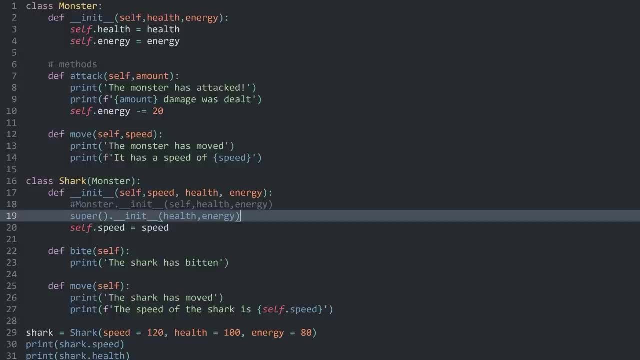 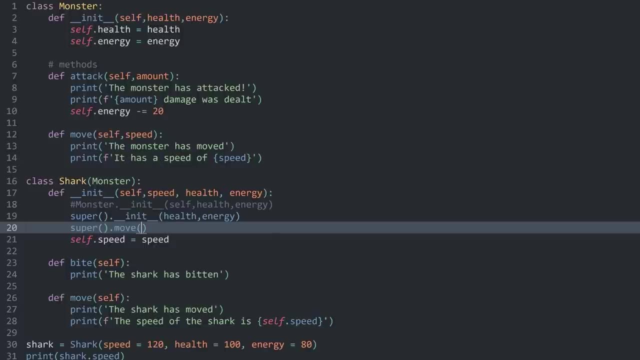 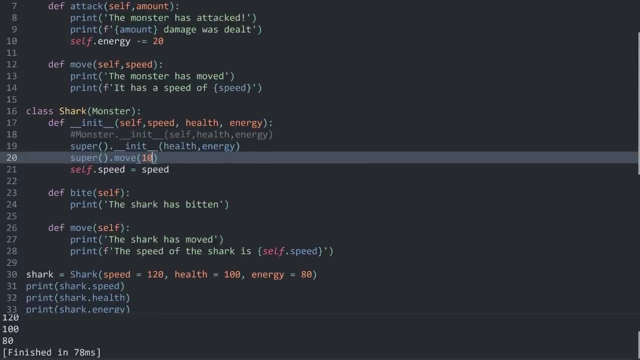 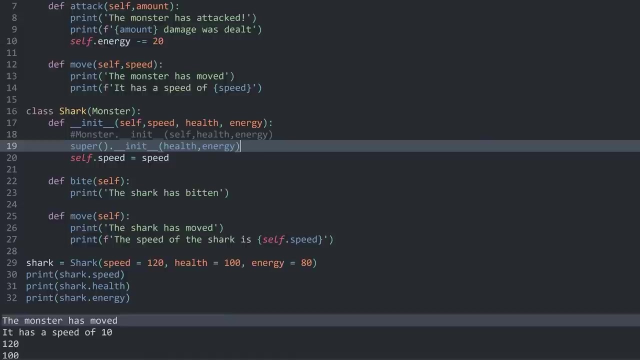 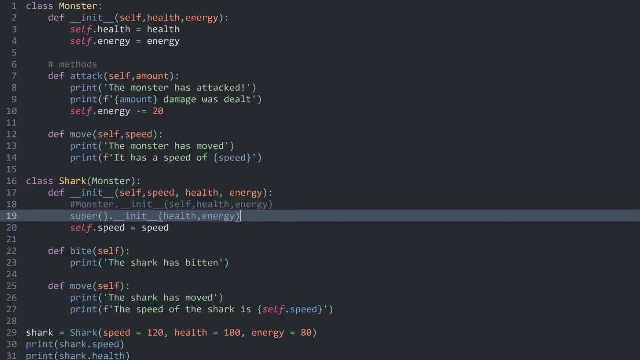 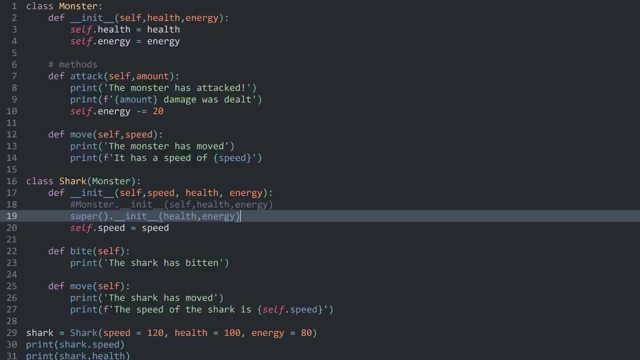 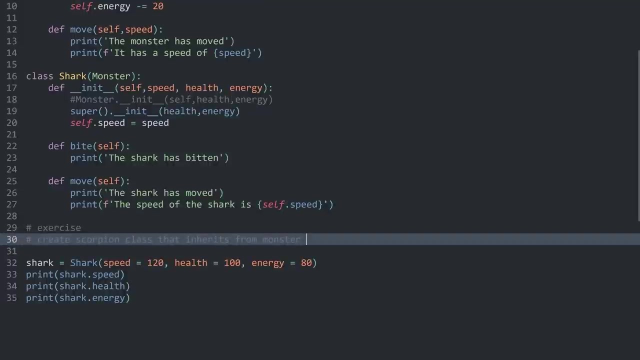 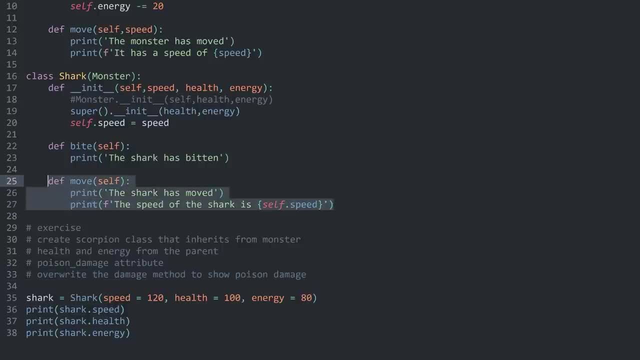 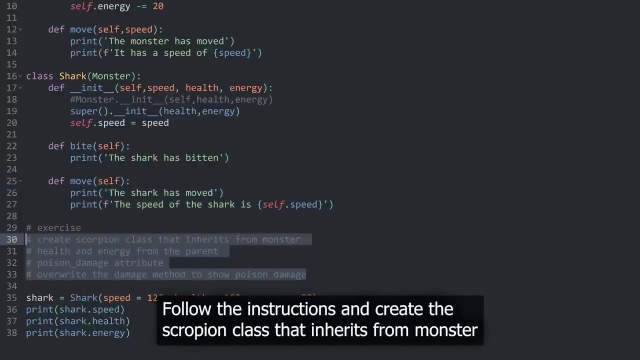 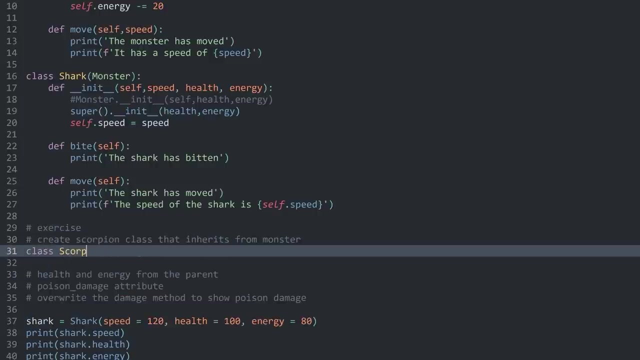 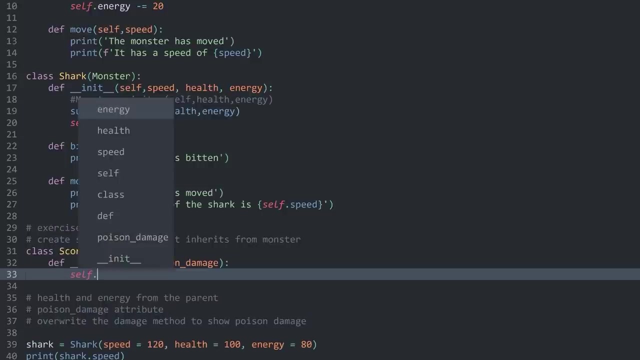 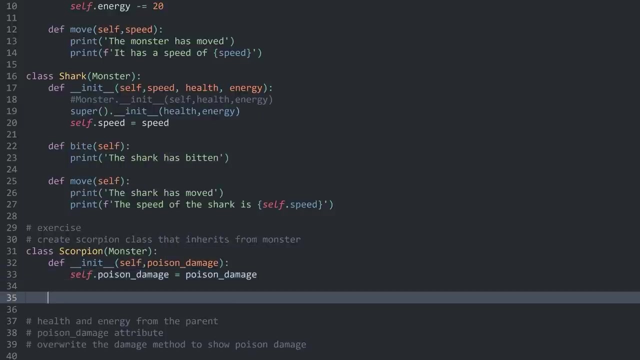 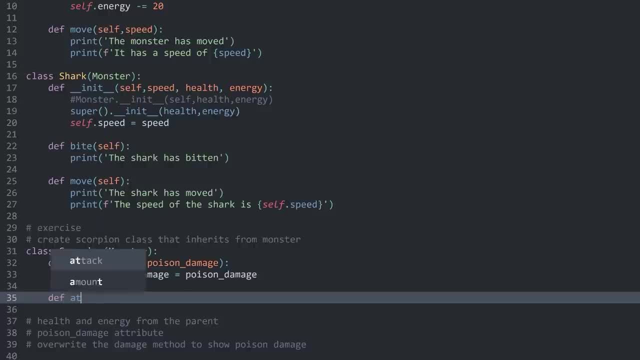 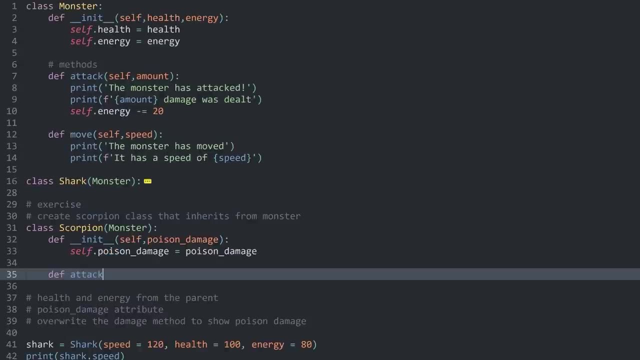 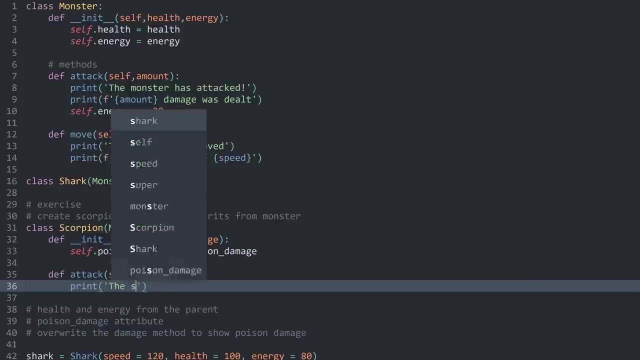 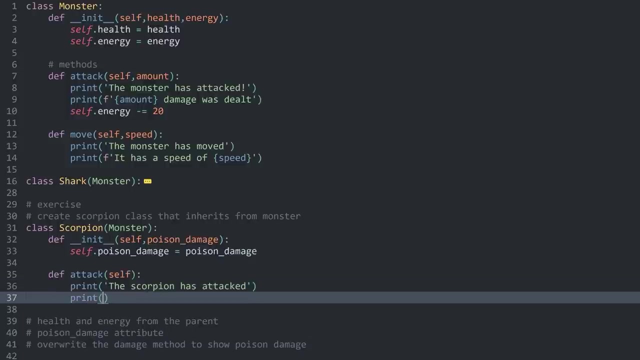 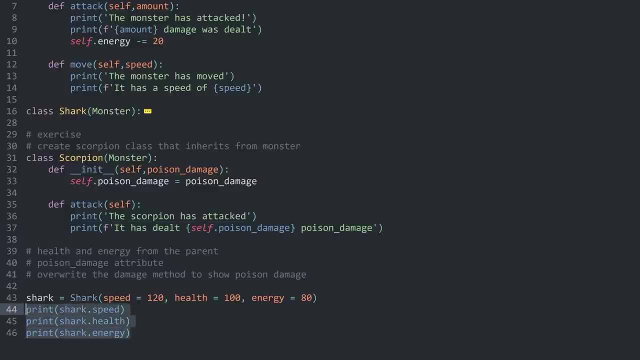 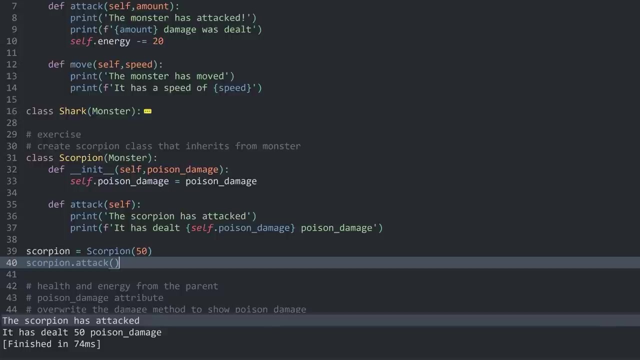 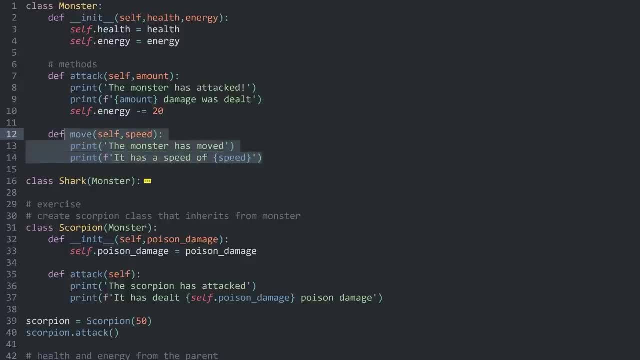 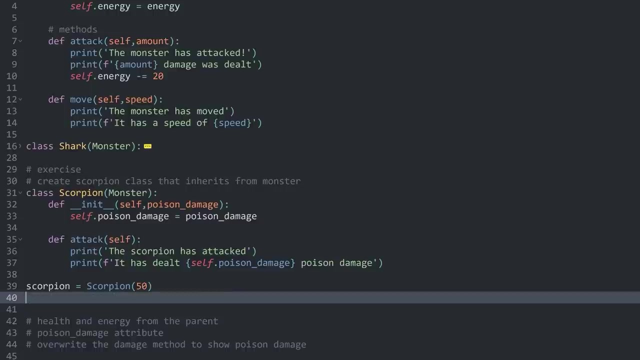 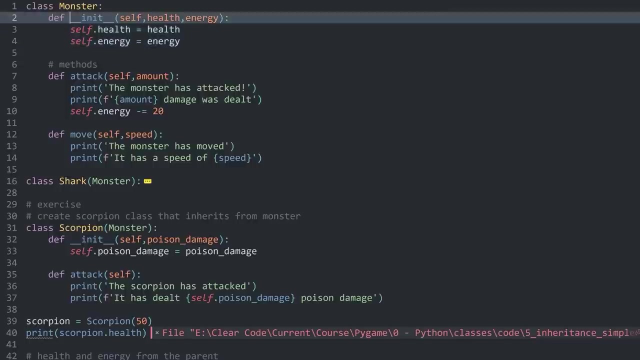 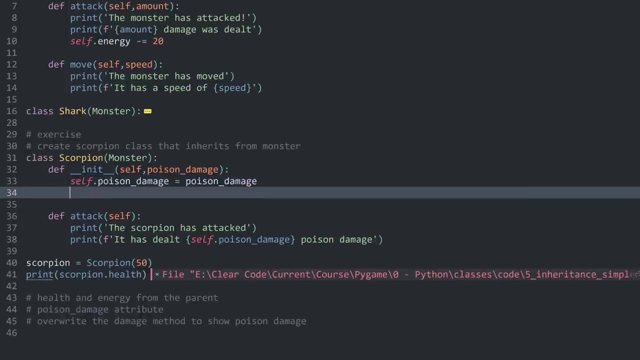 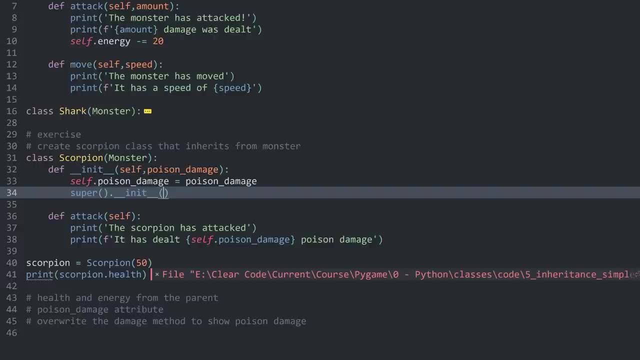 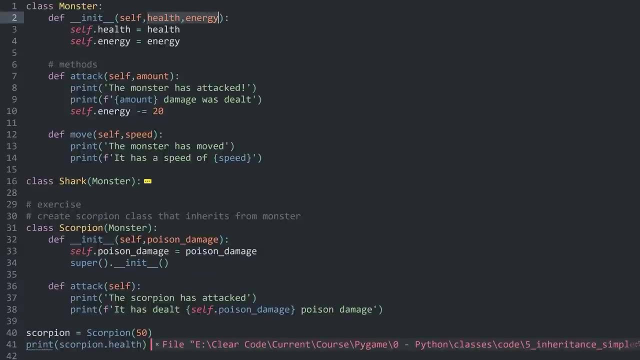 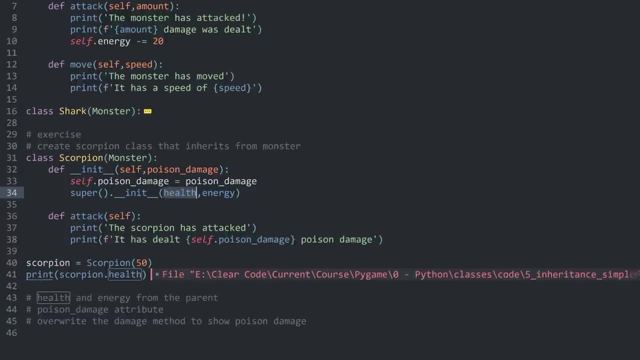 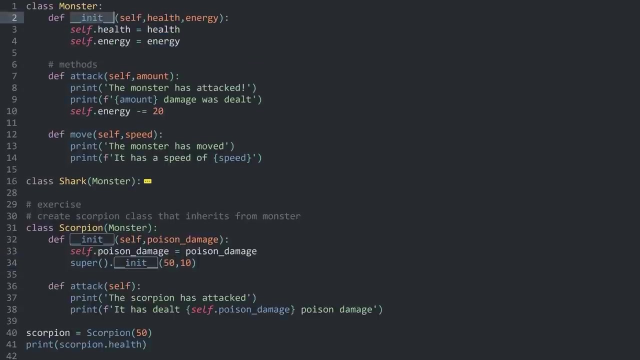 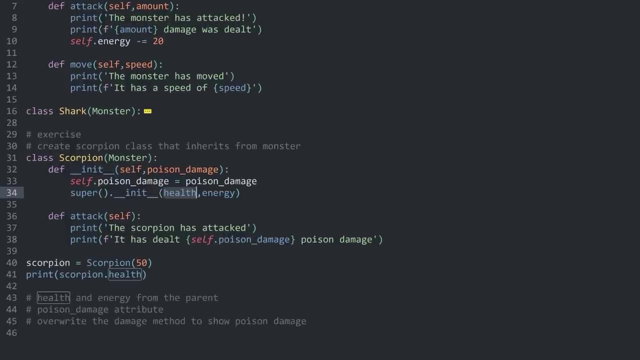 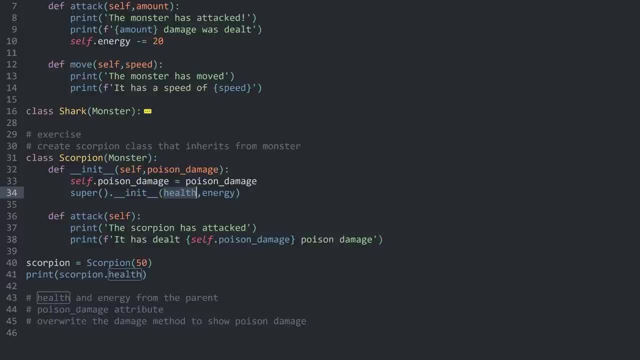 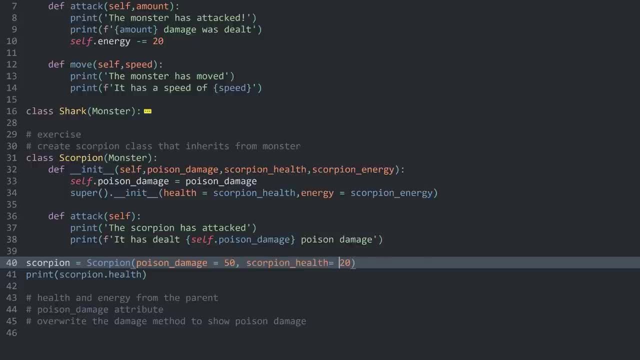 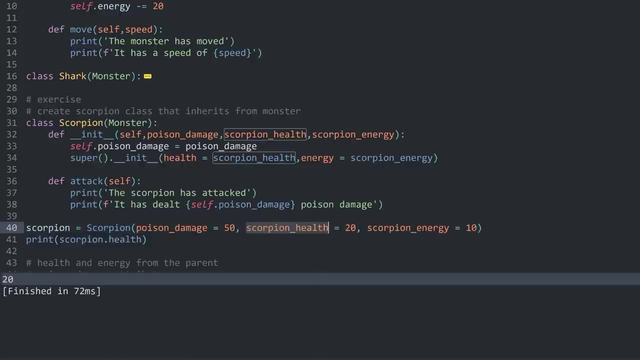 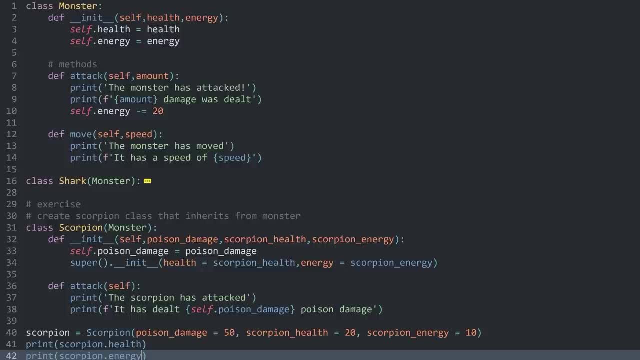 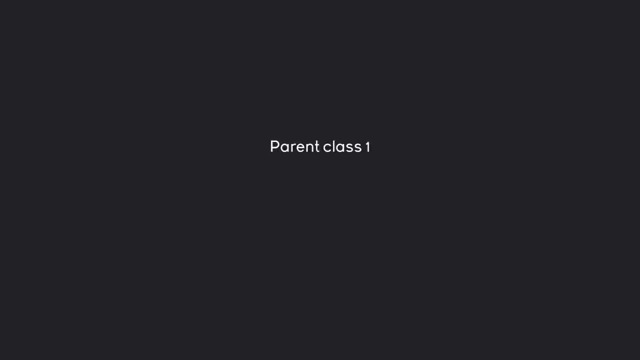 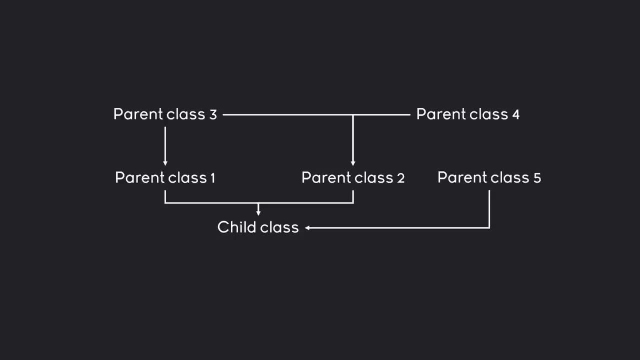 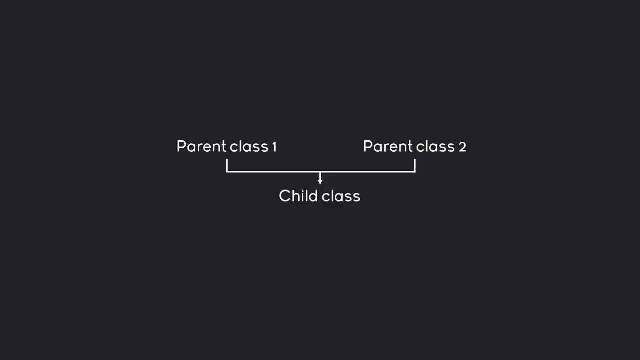 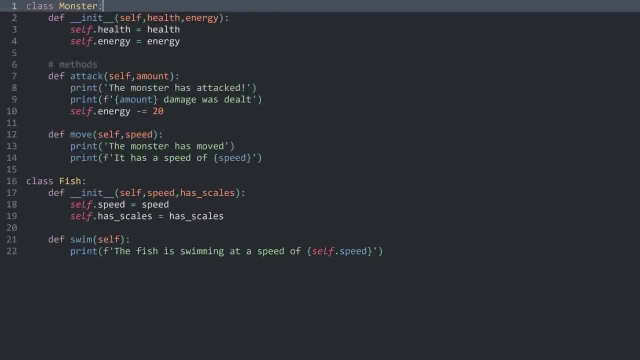 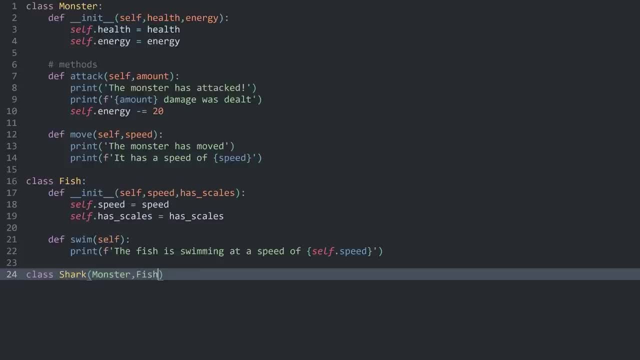 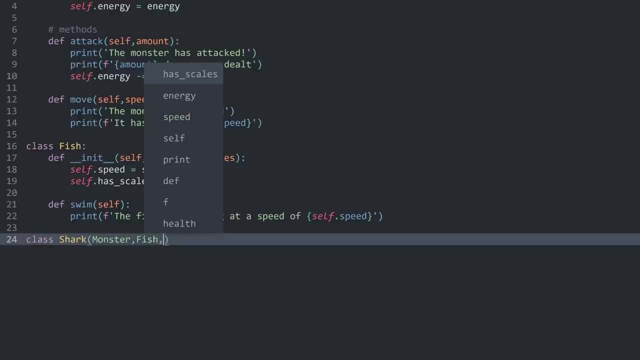 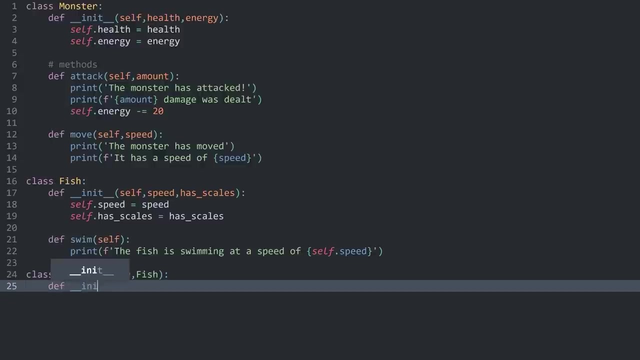 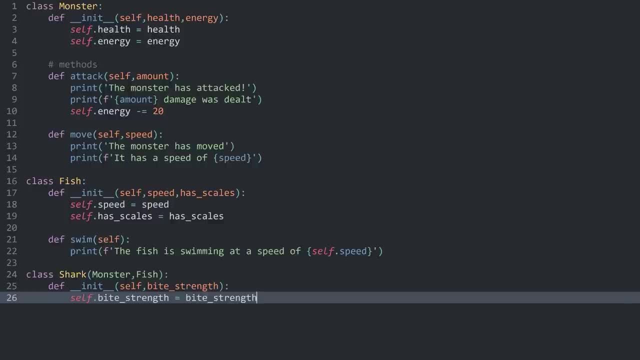 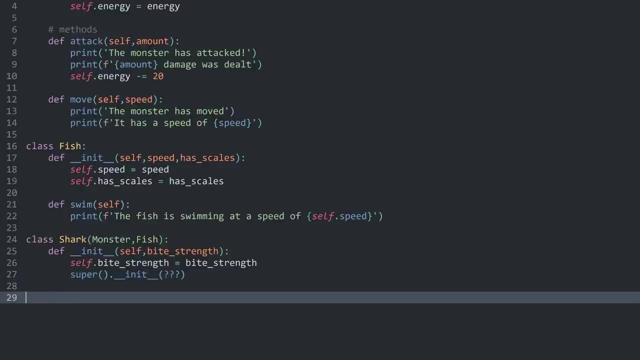 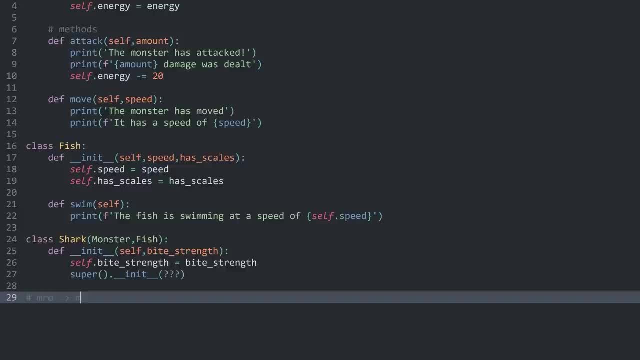 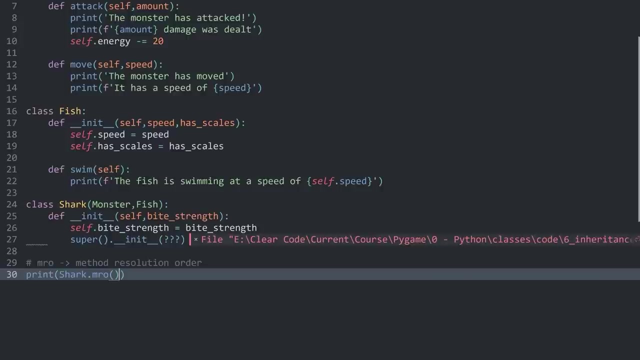 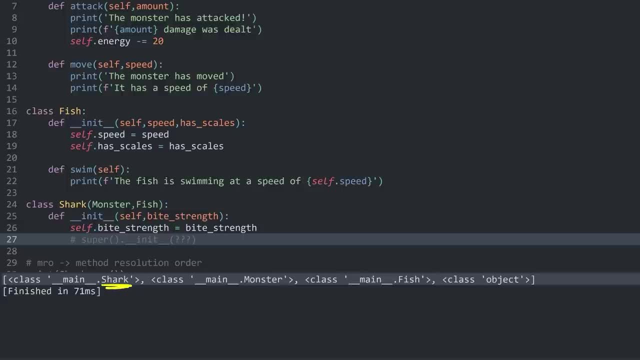 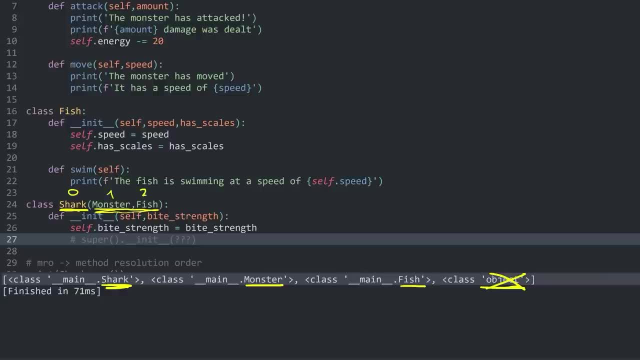 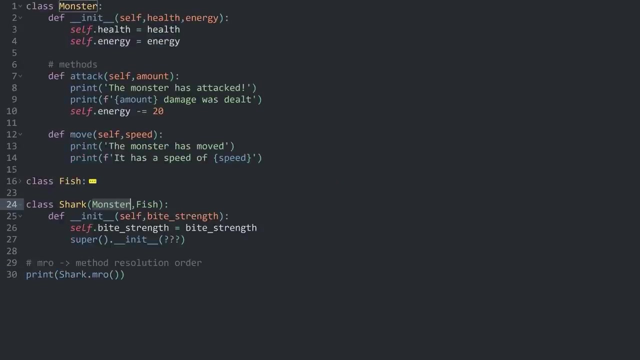 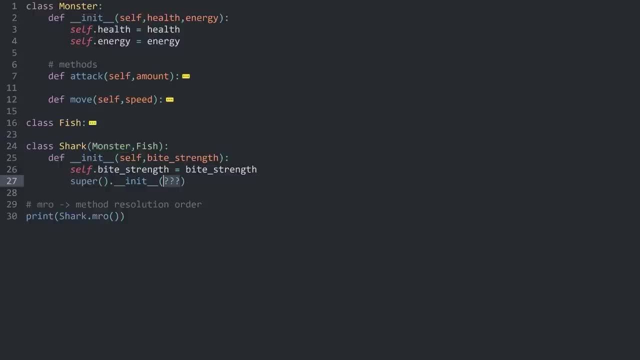 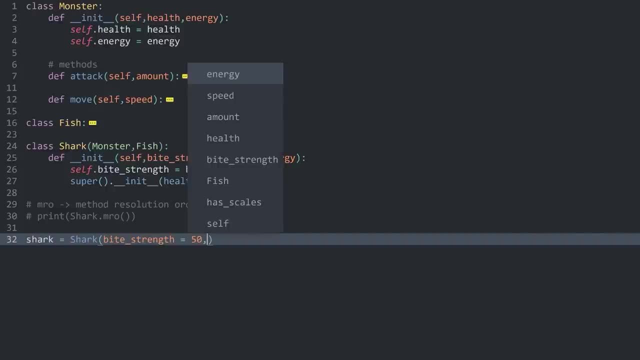 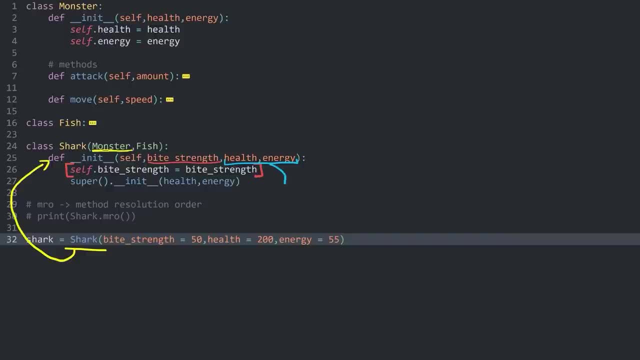 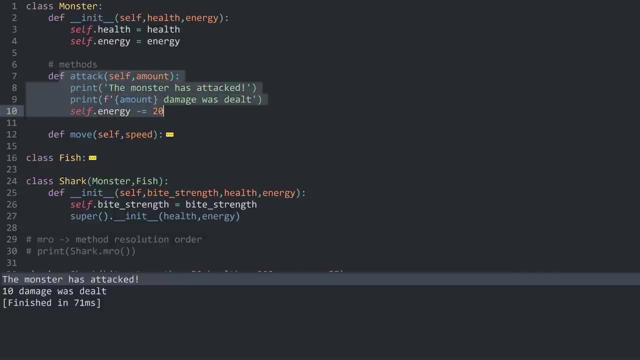 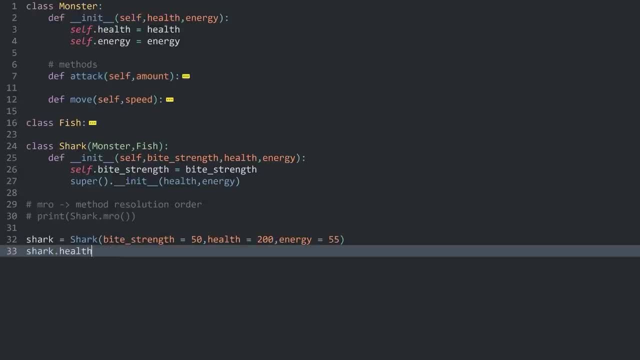 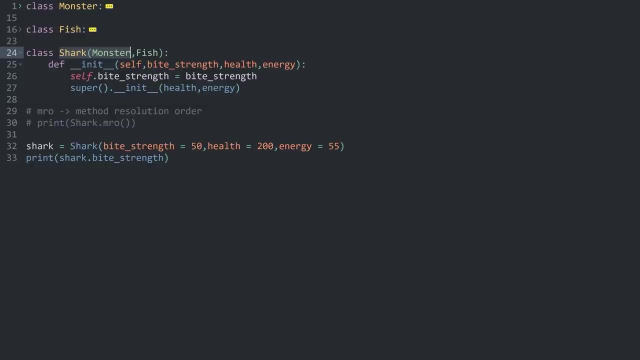 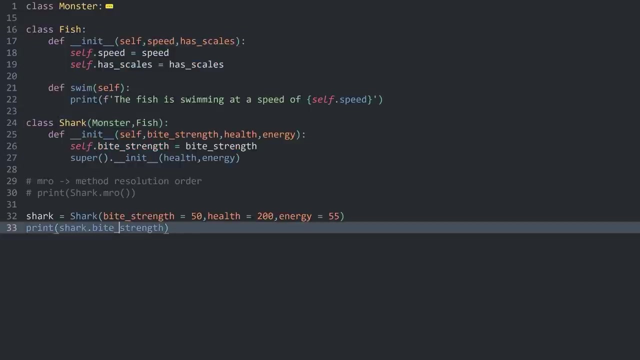 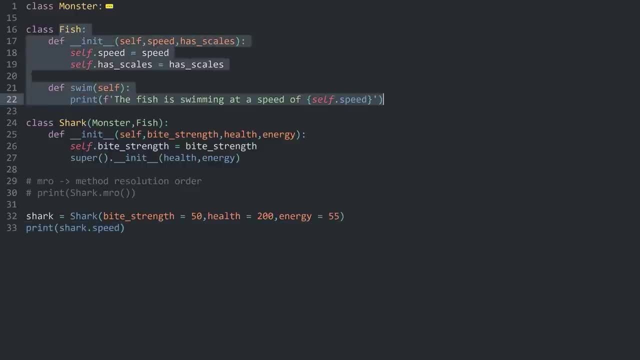 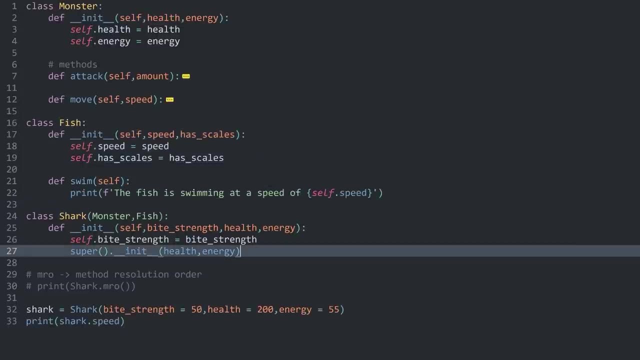 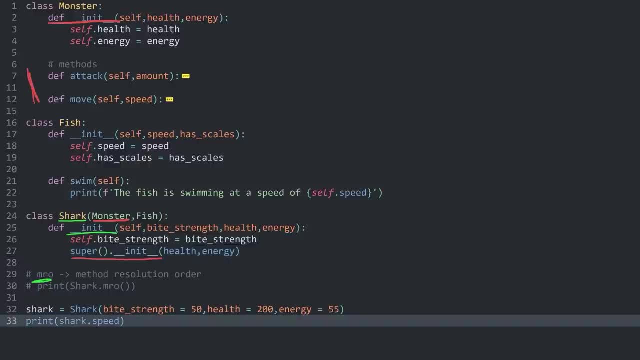 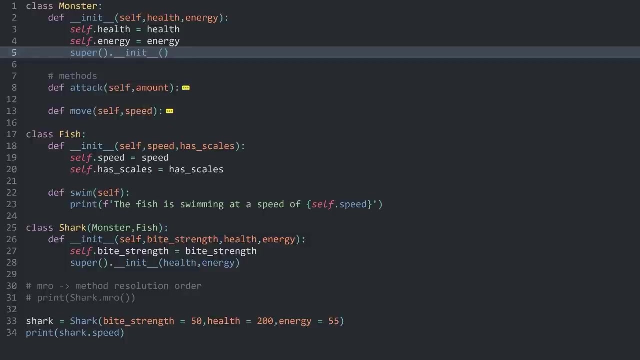 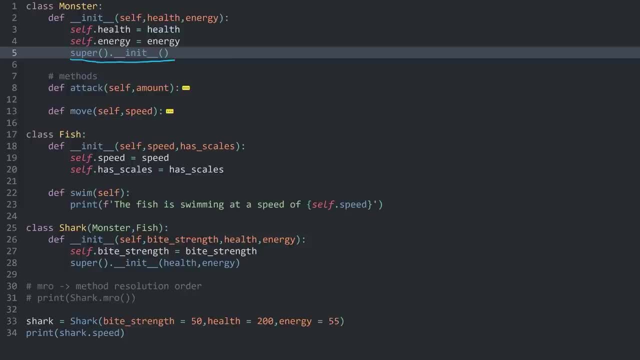 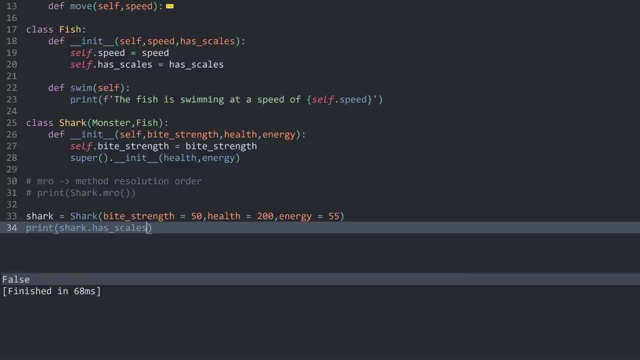 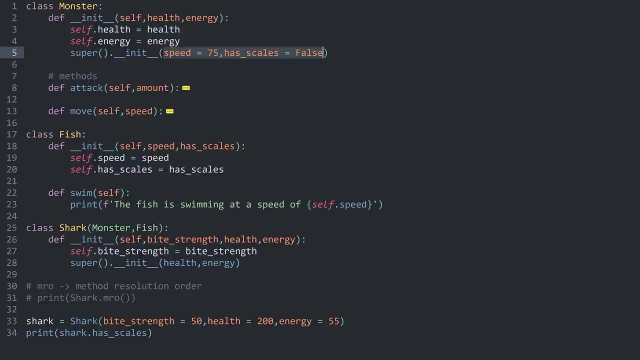 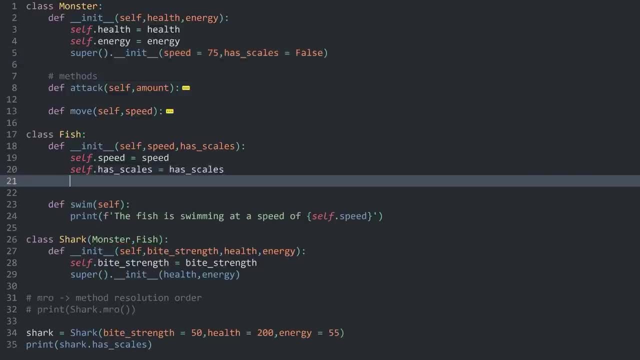 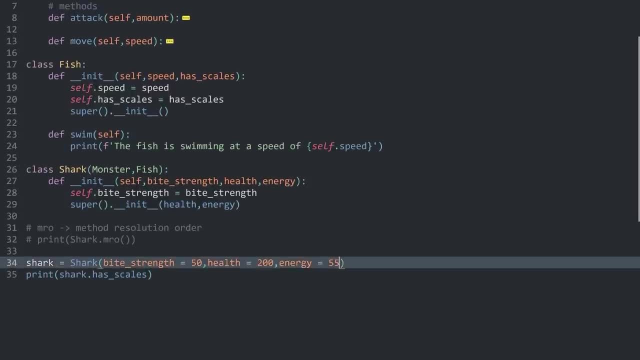 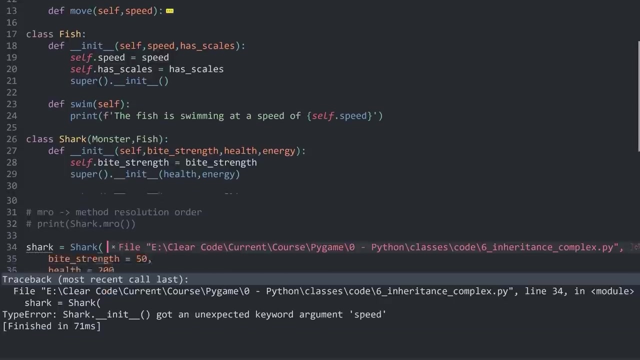 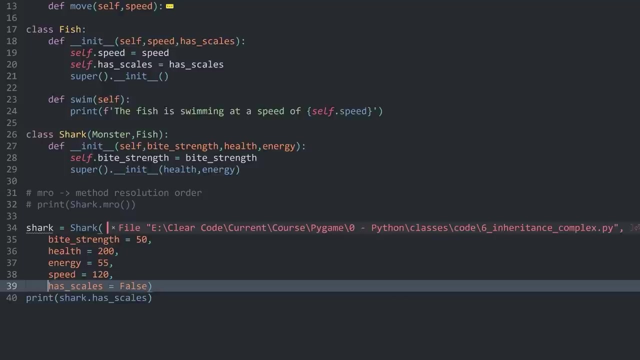 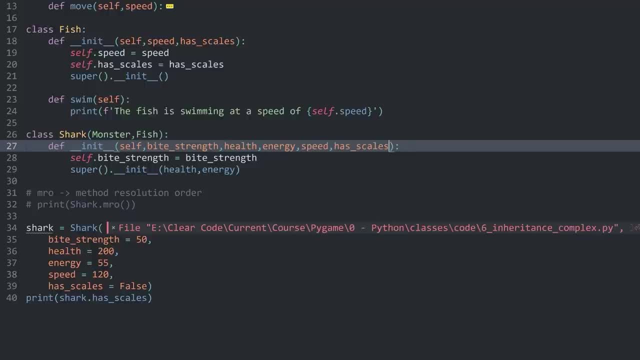 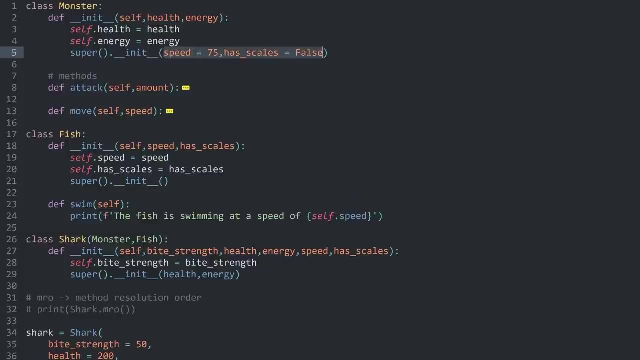 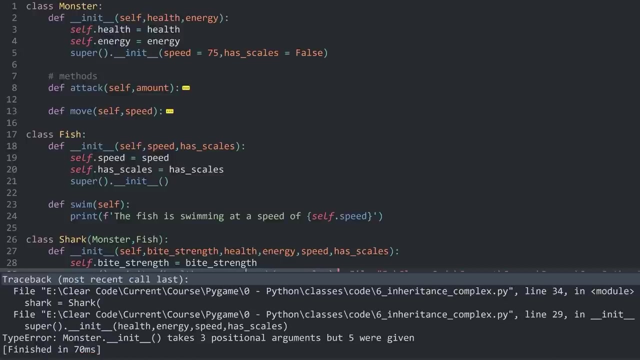 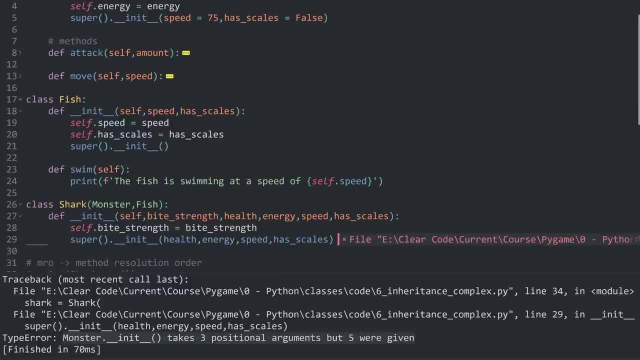 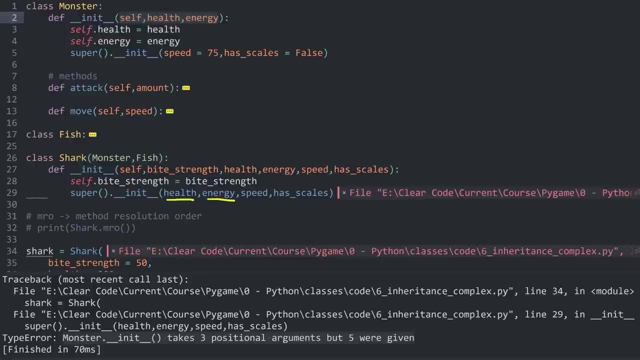 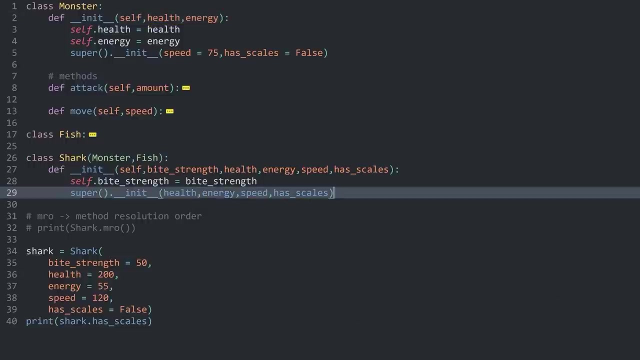 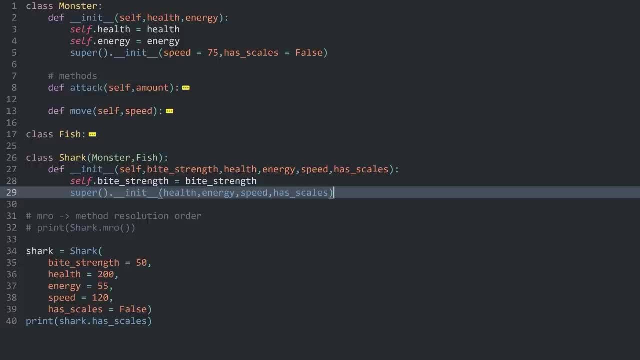 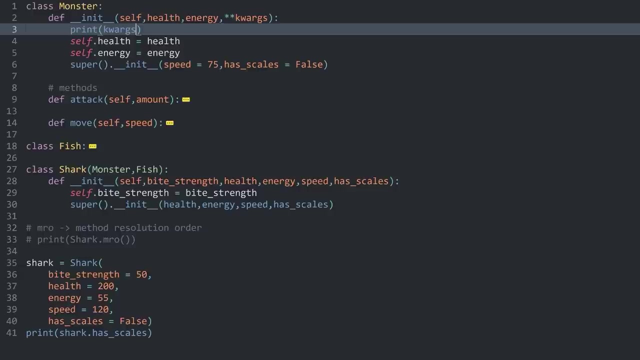 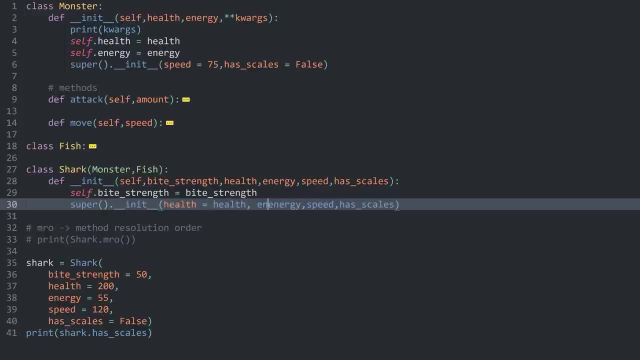 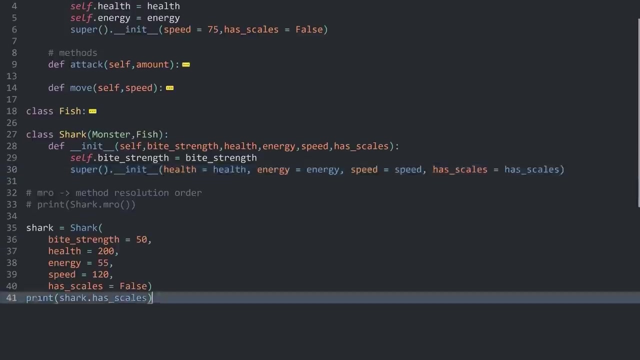 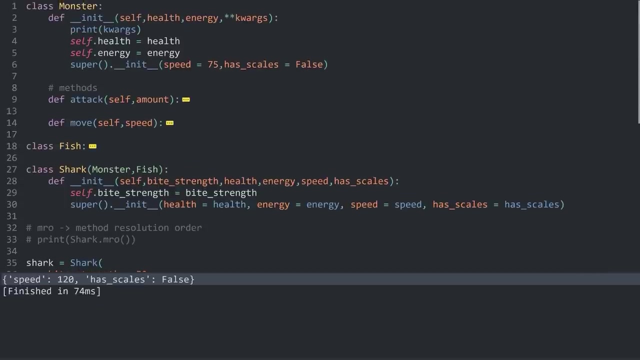 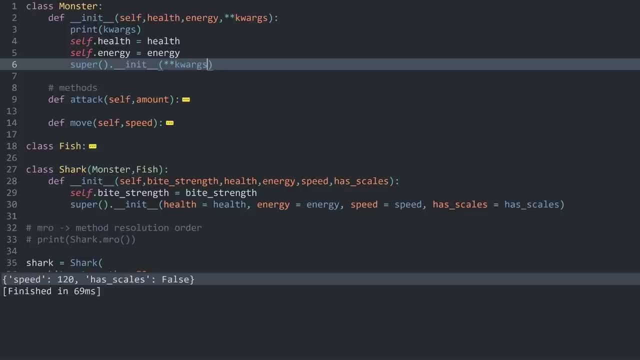 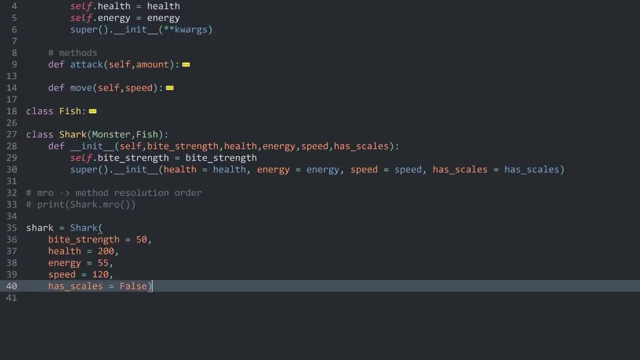 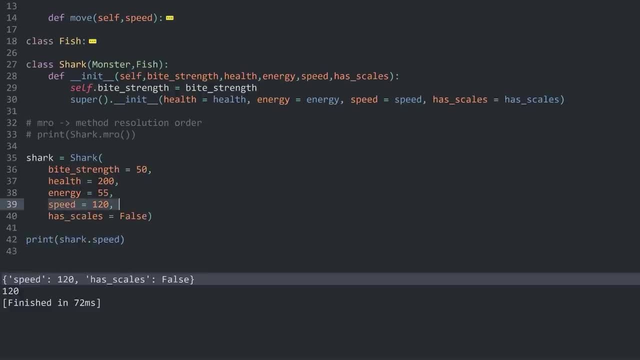 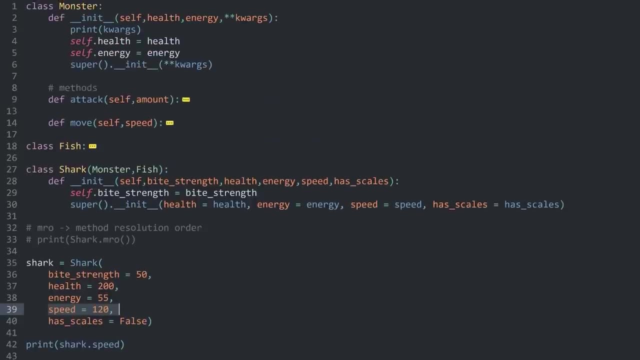 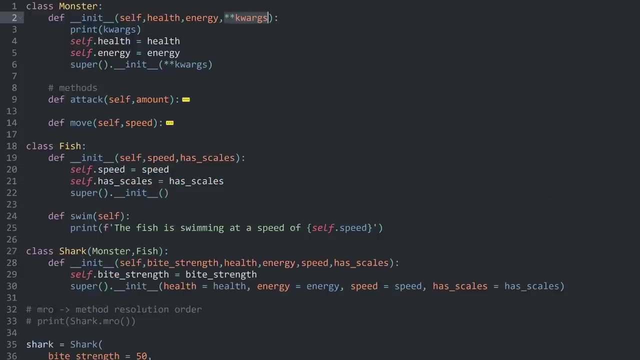 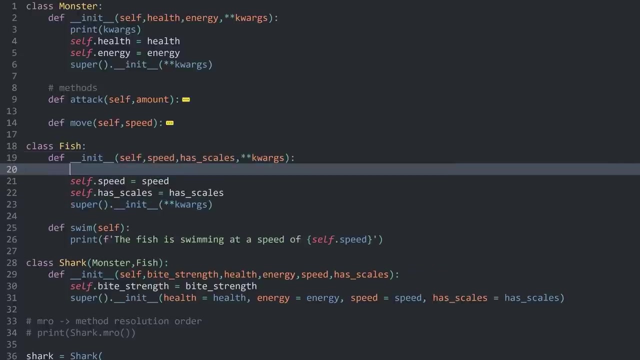 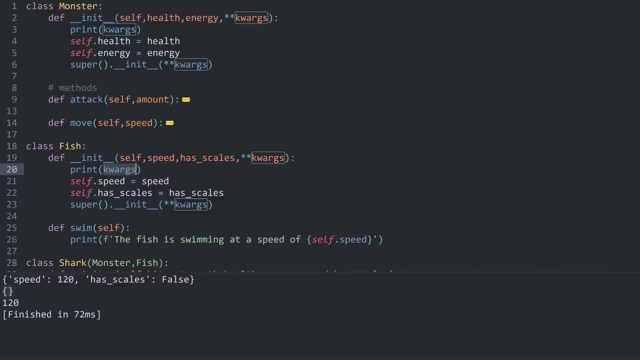 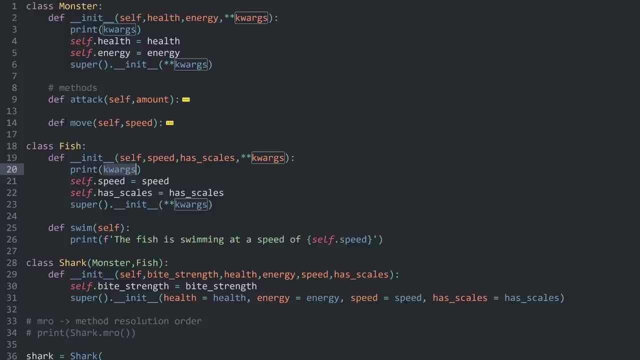 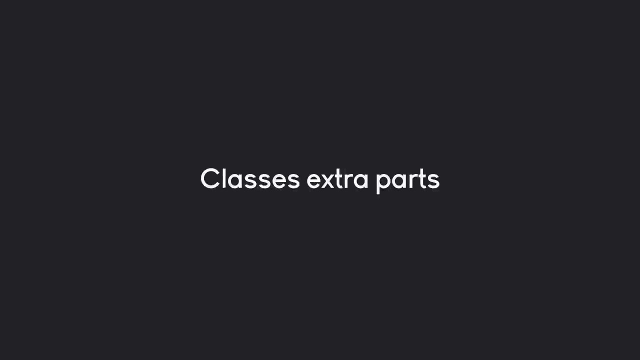 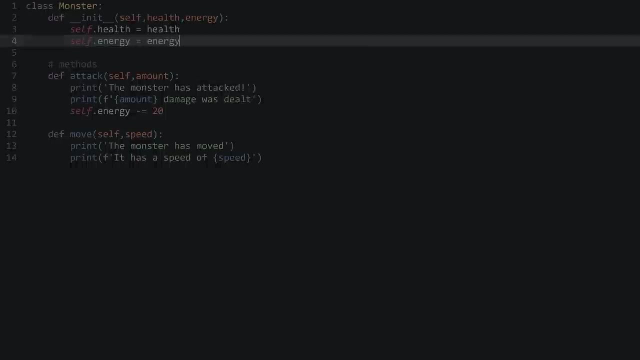 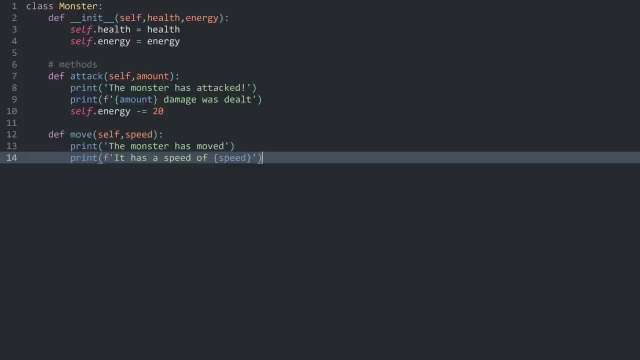 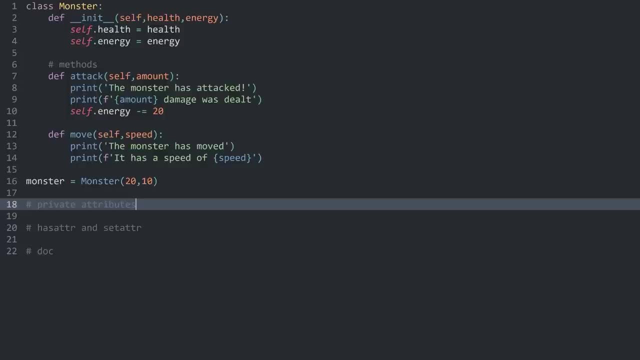 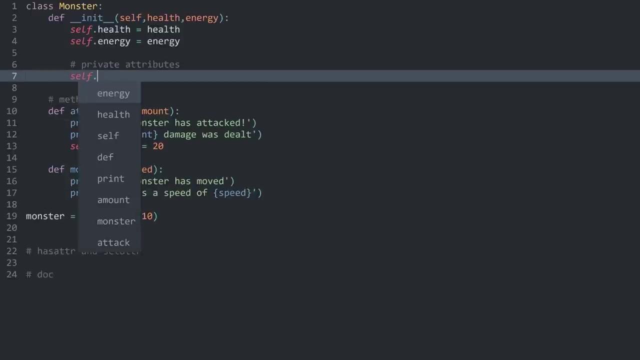 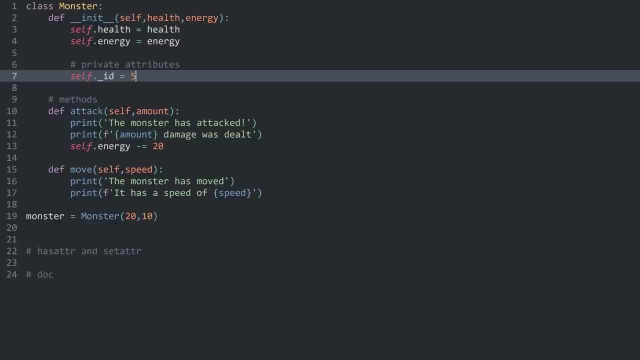 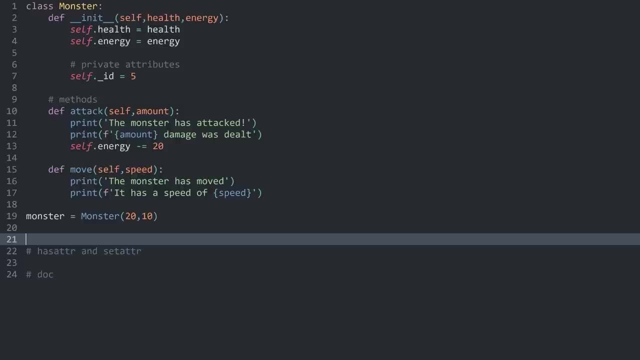 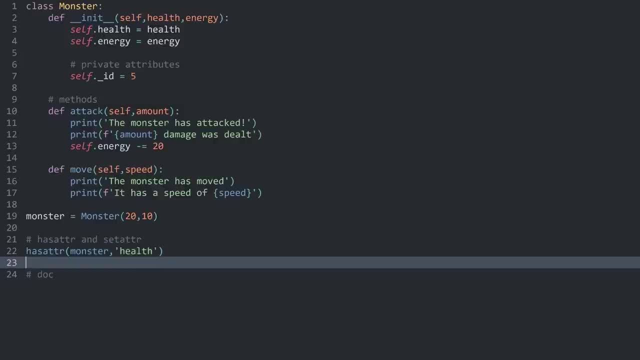 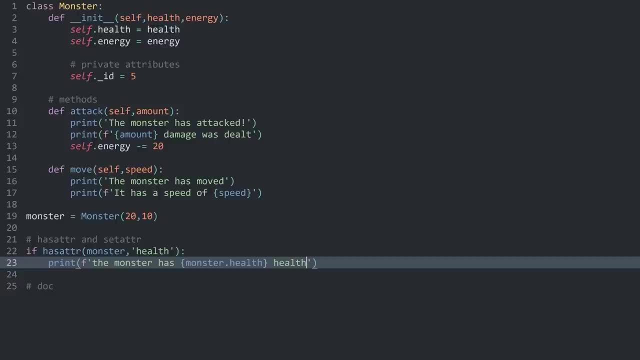 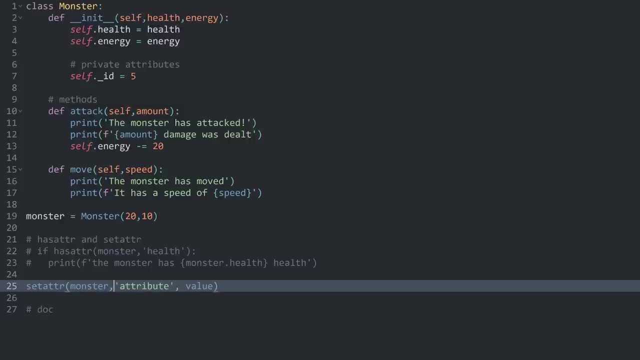 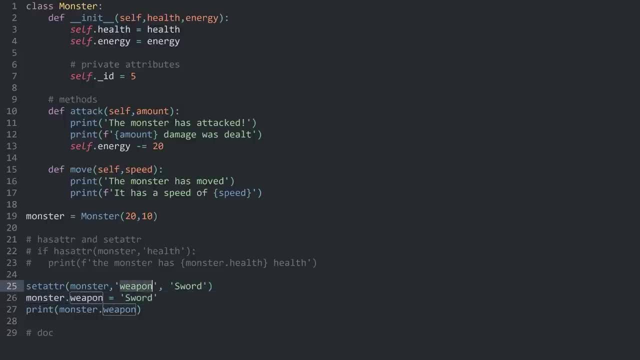 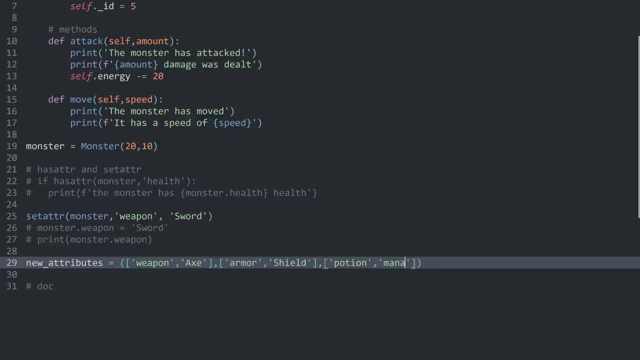 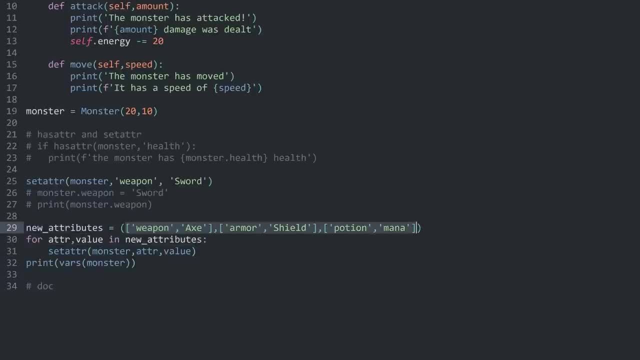 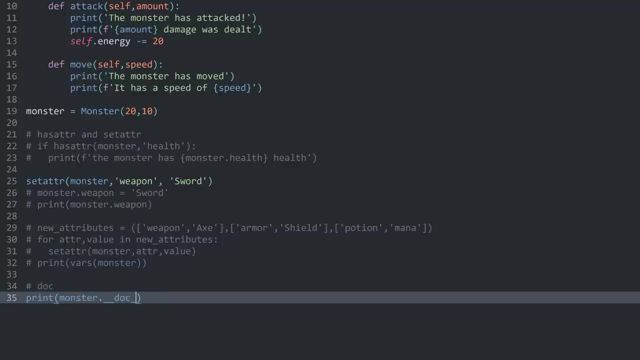 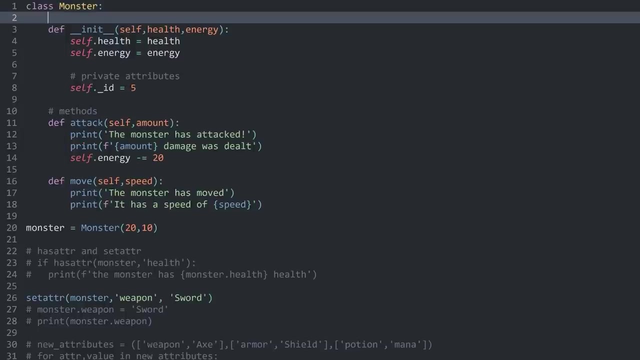 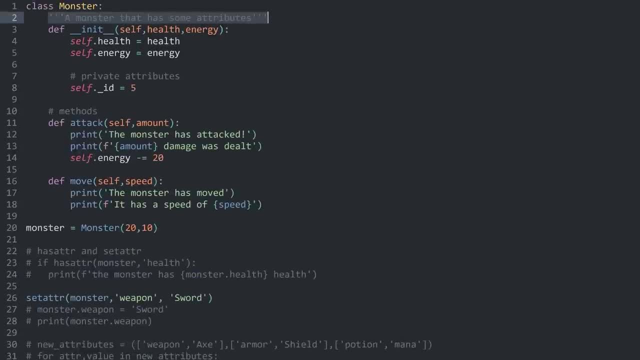 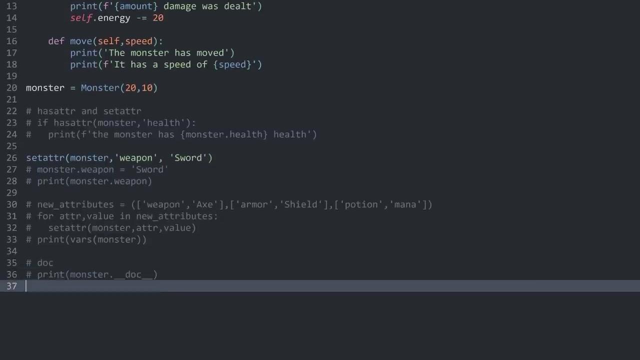 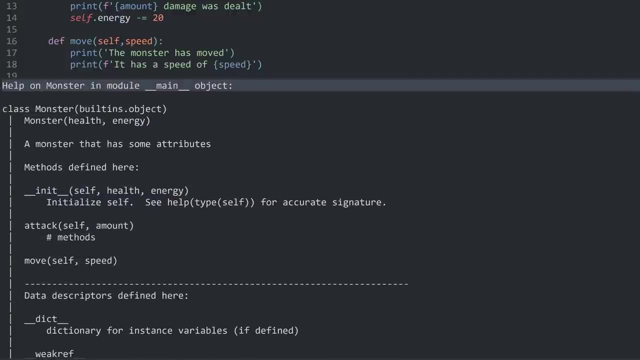 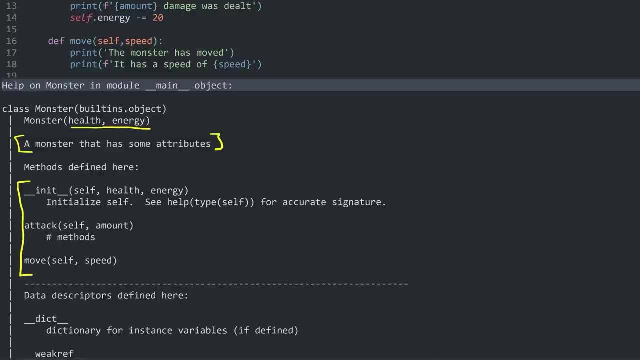 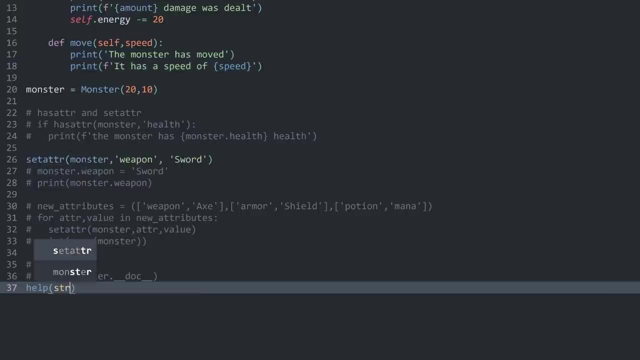 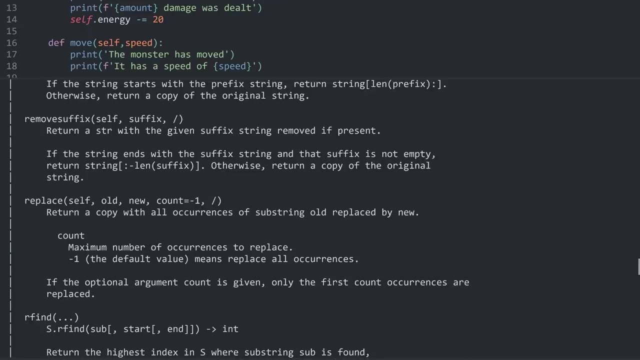 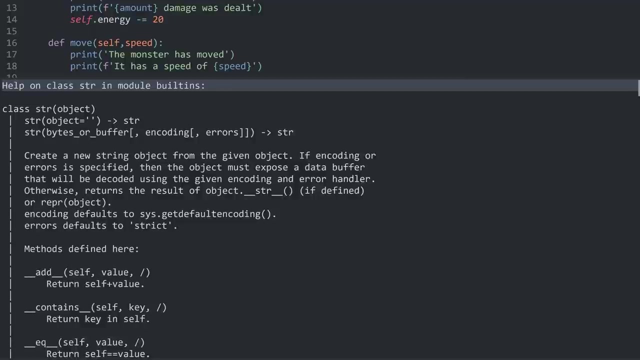 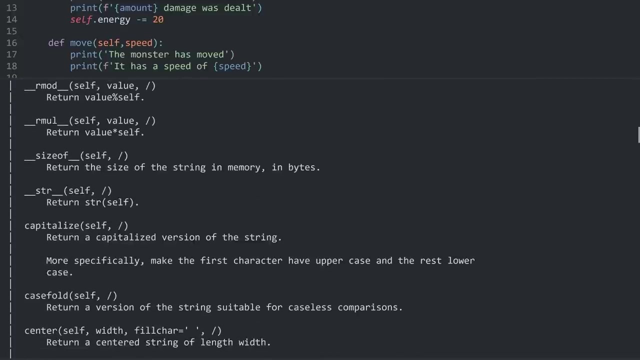 how to use this method in the next video. I will show you how to use this method in the next video. I will show you how to use this method in this video. I will show you how to use this method in the next video.